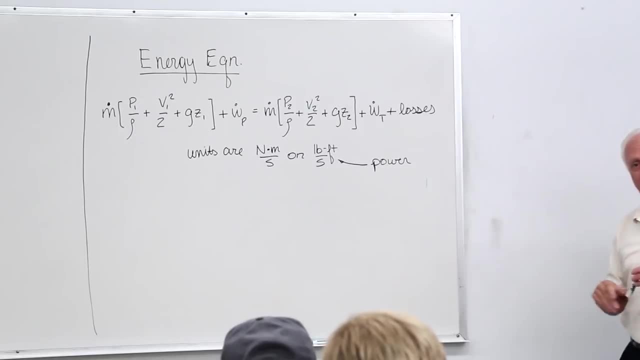 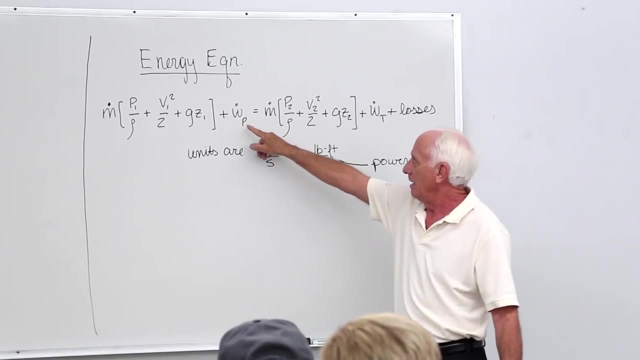 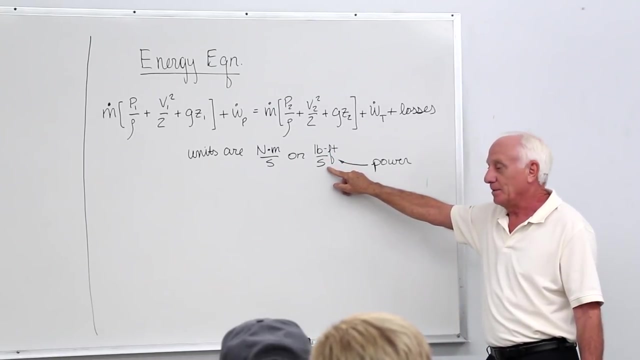 pound foot per second. Those guys are in power because a newton meter is a joule. A joule per second is a watt. These guys are typically in kilowatts. Pump power, turbine power- These guys are in pound feet per second. That can be converted into horsepower. So this 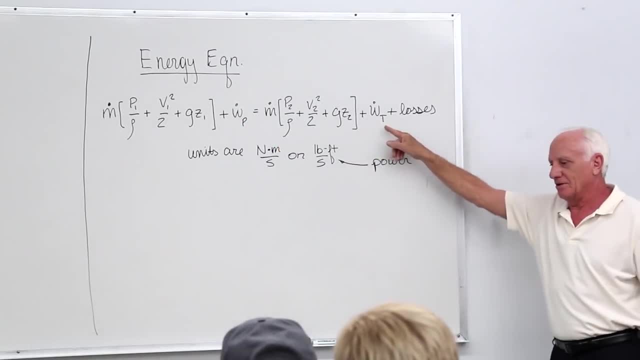 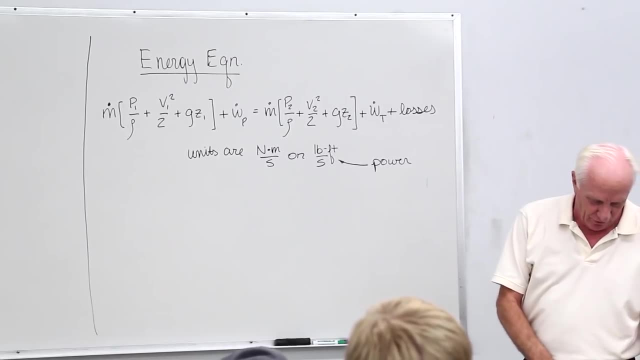 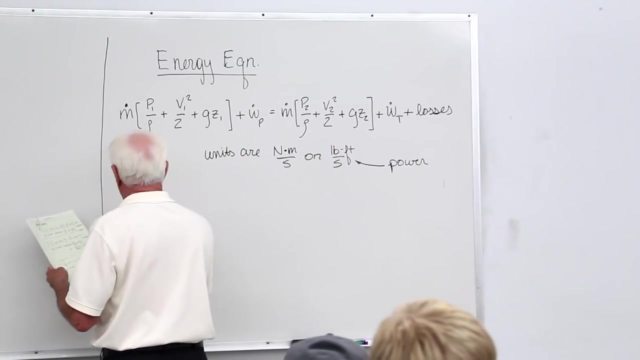 pump can be horsepower. W dot turbine can be horsepower. Now we have two other equations that we also looked at. One of them, I'll just do the one- that the head on the equation. This is the head form of the energy equation. We use gamma rather than rho. now 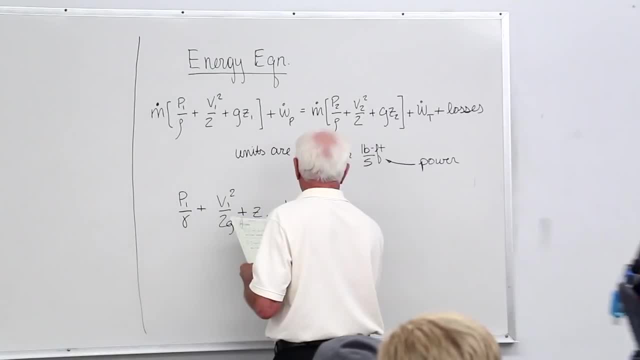 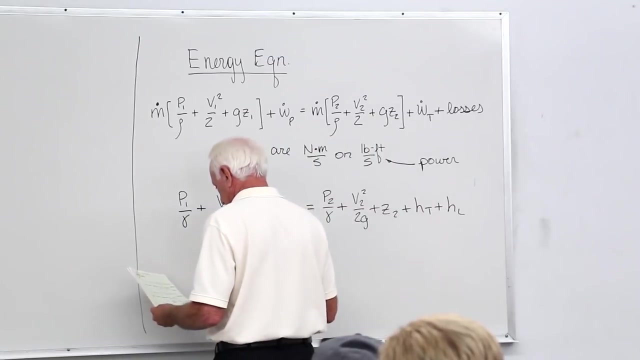 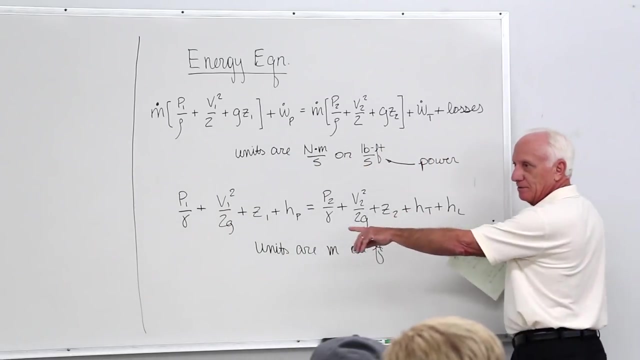 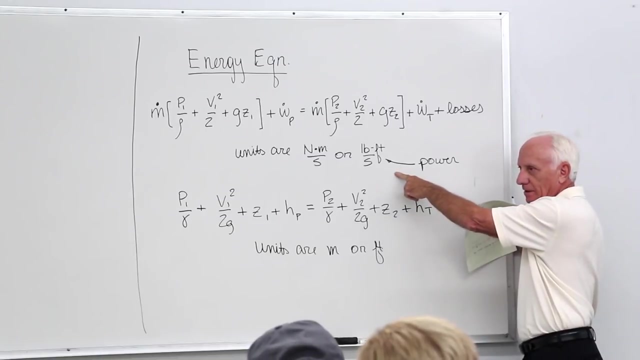 In this equation all the units of the terms are in, as you can see, meters or feet, And we call H sub P the pump head. We call H sub T the turbine head. H sub L is the loss head. Everything is in meters or feet. This guy is in kilowatts or horsepower once you convert. 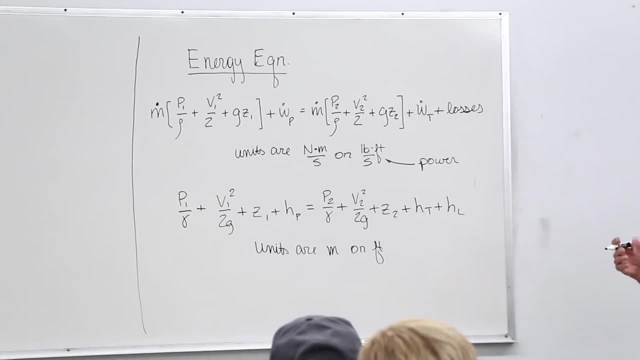 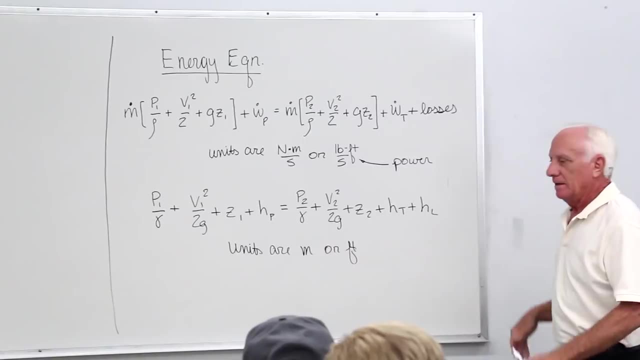 it. So you pick out the equation that you need. If the problem gives you the power in horsepower of a pump or a turbine, I'd probably use this one. You'll see in homework. If the problem gives you the losses in terms of feet of head, I 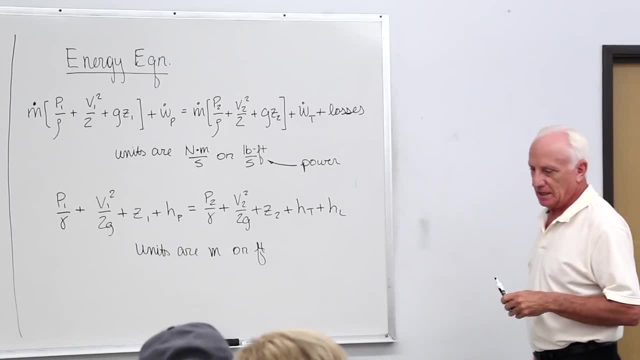 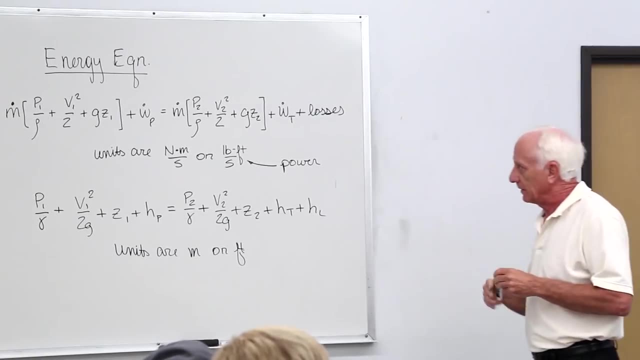 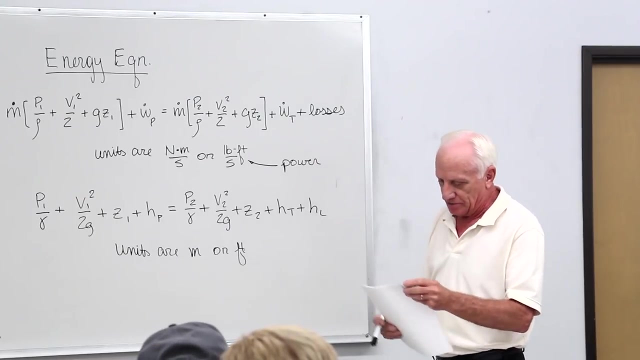 would use this one because the losses are in feet of head. So it depends how the problem stated to you which equation you might want to use, But they're equivalent. They're the same thing. Okay, There's three equations in your notes from last time. I put two back. 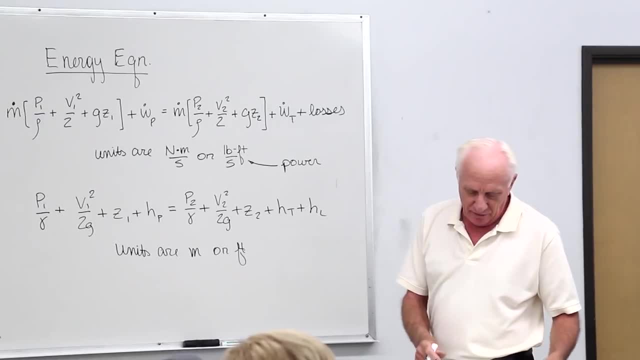 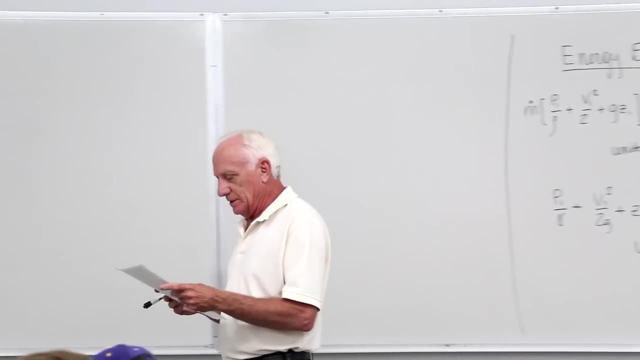 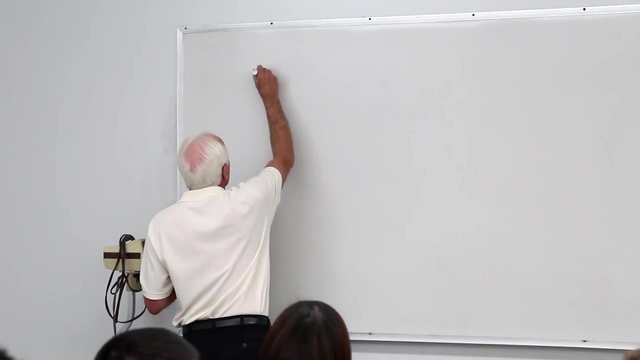 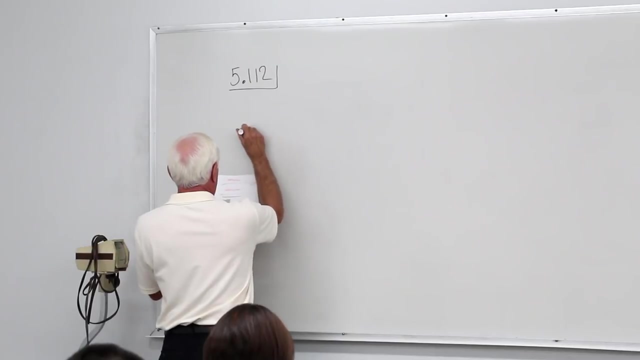 on the board here for you. The third one is in your notes And we worked an example problem last time. So you have problem 110 and 113 for homework. Let me just do problem 5-1-12.. It's in the middle of the two for homework, 5-1-12.. So we have this. would be a lake. 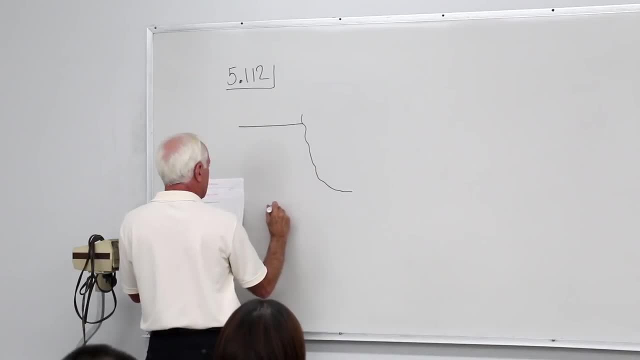 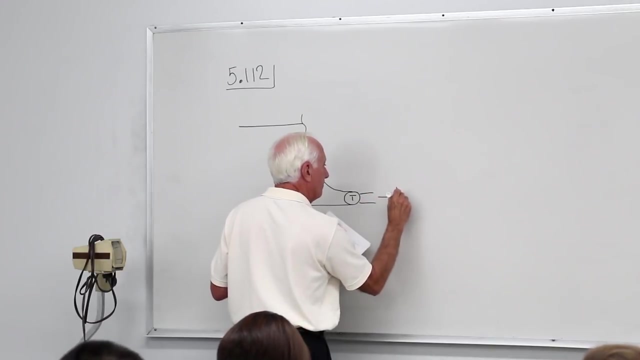 And then there's. this is how the picture looks. Looks something like this: At the bottom, here there is a turbine And let's see One meter in diameter. Yeah, One meter in diameter, and the velocity is six meters per second, leaving the turbine. And this diameter is one meter. Let's see. 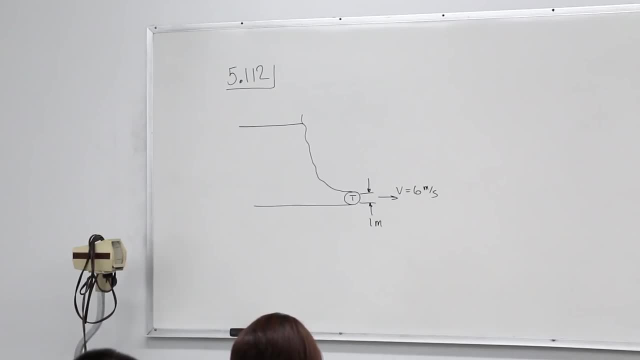 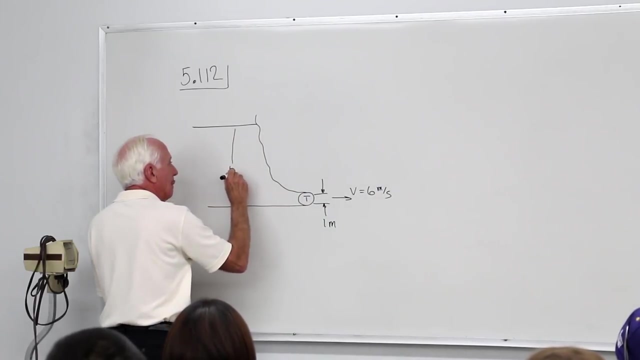 if that picture in the textbook looks somewhat like what I put on the board there. One-twelve, Yeah, Okay, Turbine, six meters- salir de vida. Okay, Fifty meters from the free surface down, So 50 meters down. 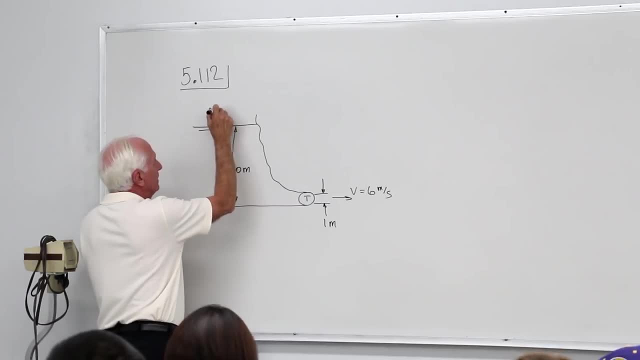 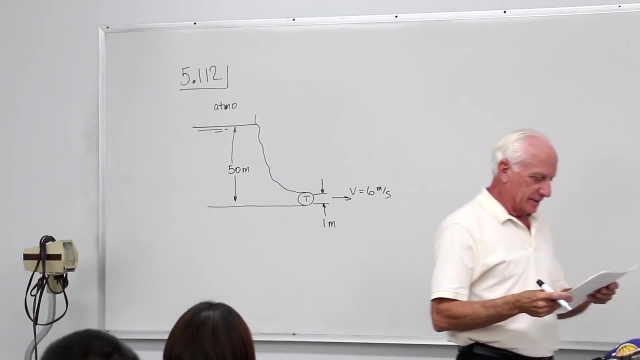 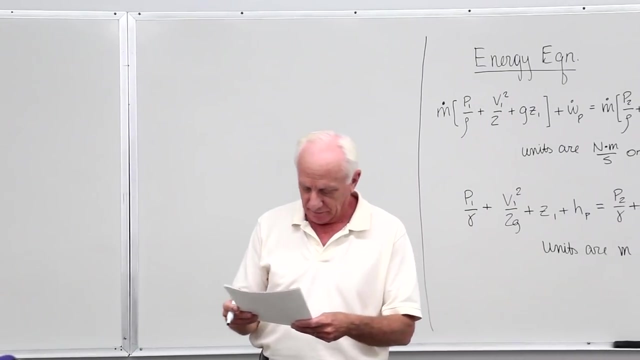 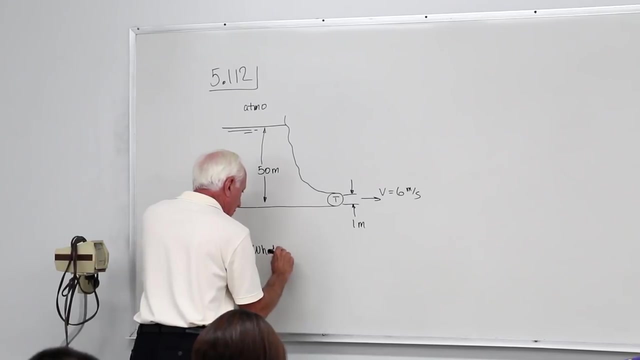 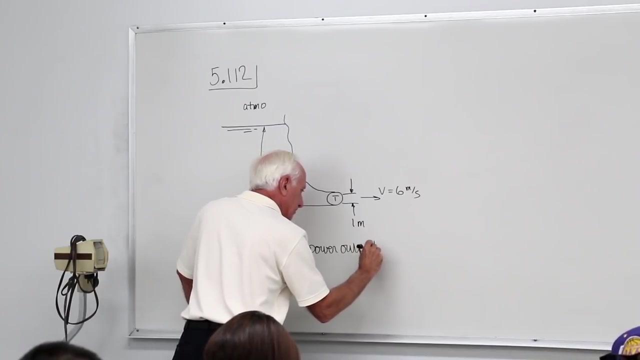 Superb, Okay, And this is a lake or something. atmosphere here. And the problem says: Make sense, What's the maximum power output of the turbine? So what is the maximum power output? Okay, Okay, so if I want power output, I would probably use this guy. 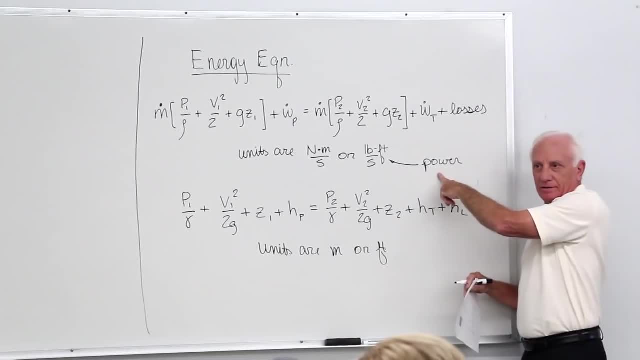 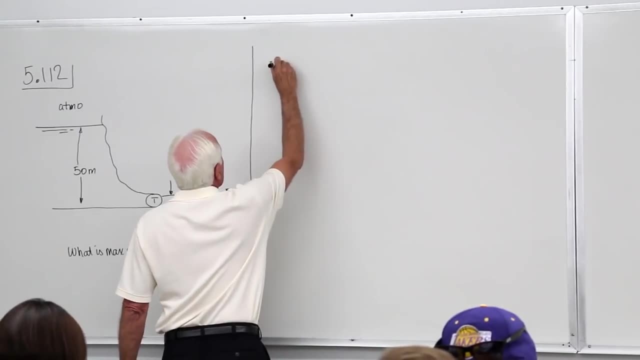 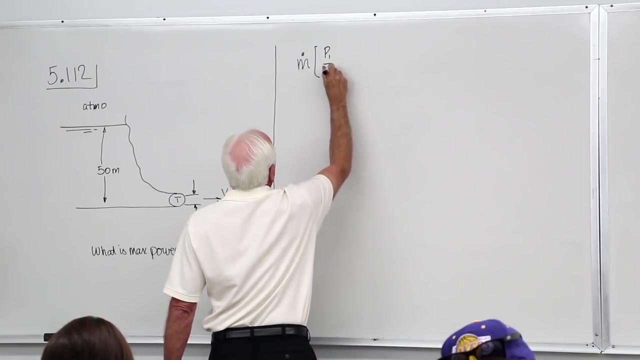 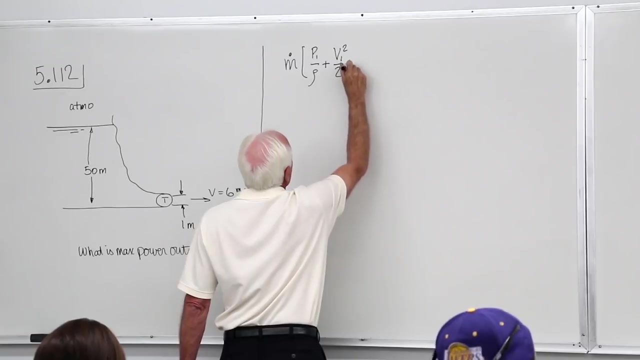 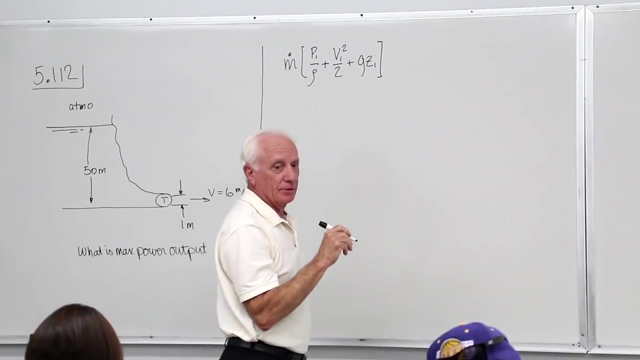 because these terms are in power, So I'm going to use that one. Okay, M dot P over rho. V1 squared over 2. GZ1.. There's no pump, so drop the HP term out. or W dot P. 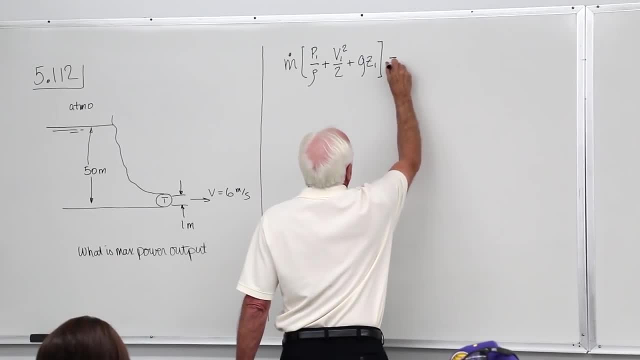 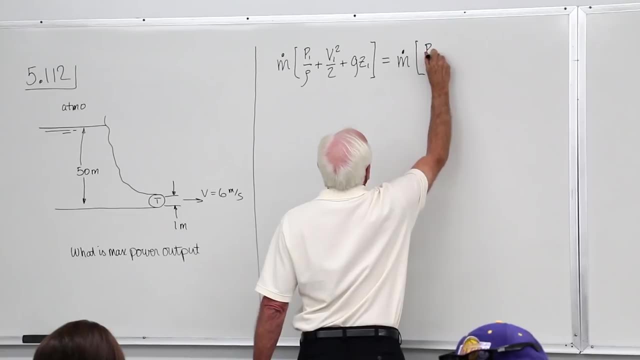 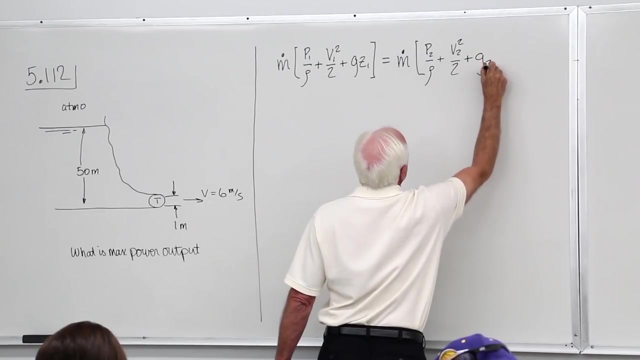 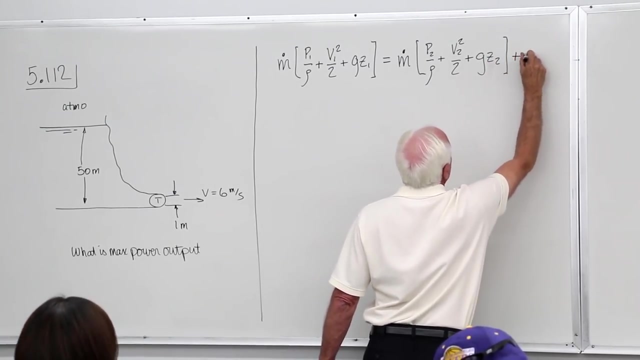 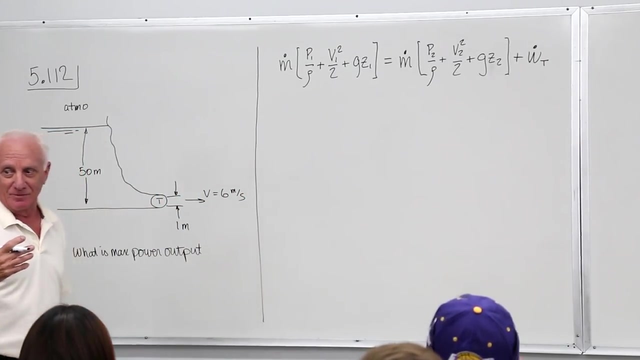 Drop out W dot P. Equal M dot P2 over rho V2 squared over 2. GZ2 plus W dot turbine: get it through the turbine, leave it in And, of course, if somebody asks you for the maximum work output. 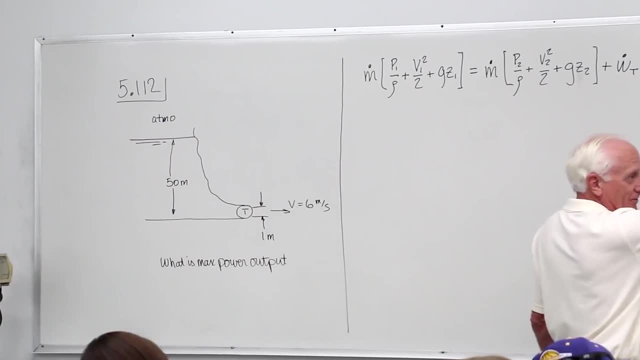 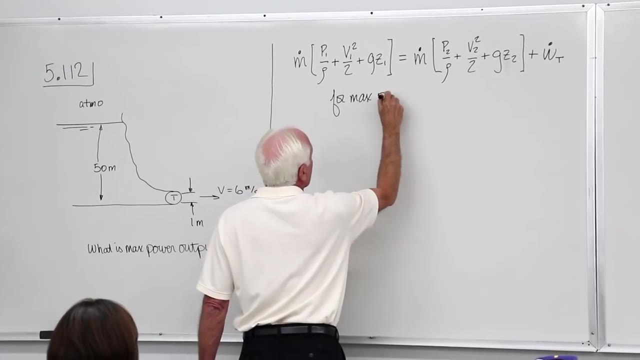 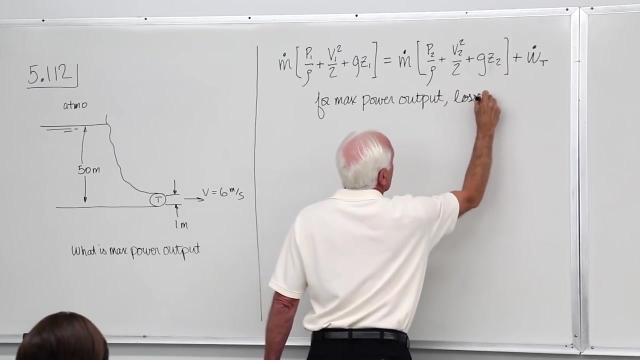 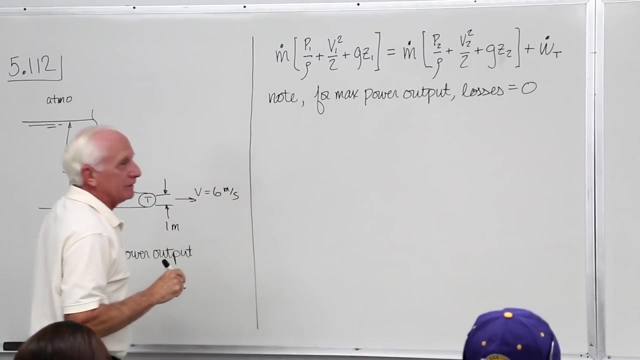 of the turbine. they mean the losses would be zero So far. max power output: Okay. Losses going to be equal to zero, Okay. so there it is. Now you have to pick out where 0.1 and 0.2 are. 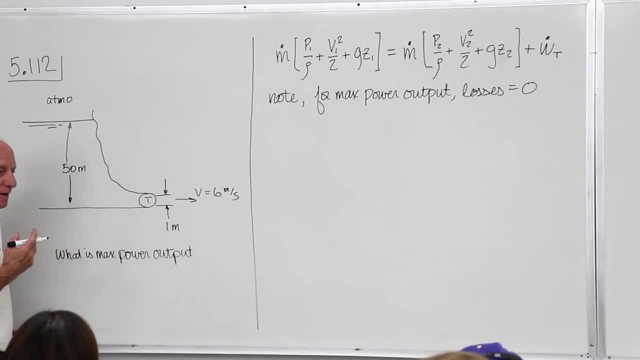 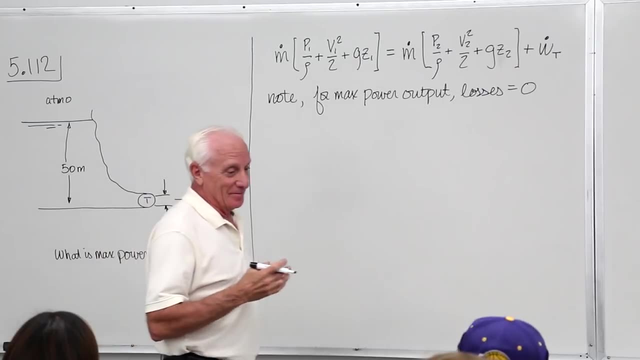 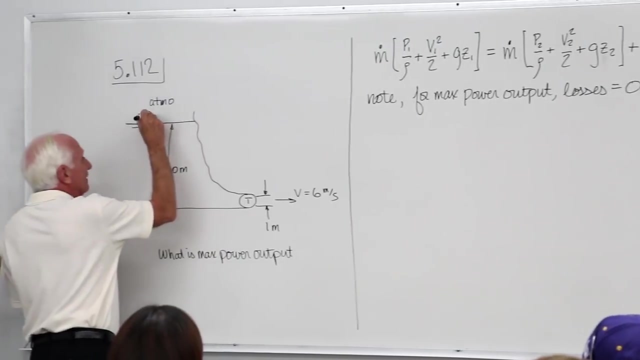 If you want to draw a control volume, you can. You don't have to necessarily. Don't forget, the energy equation is sometimes called the modified Bernoulli equation. So you know, if you want, you can go ahead and put 0.1 up here and 0.2 down here. 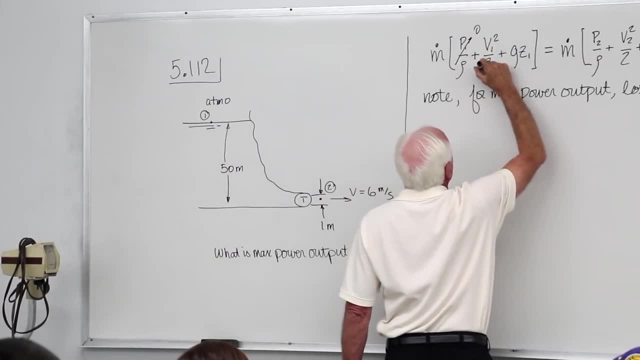 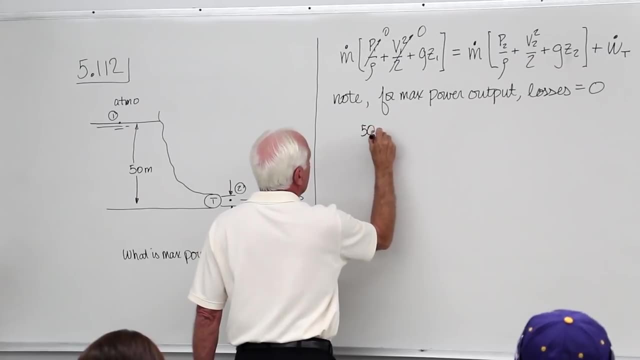 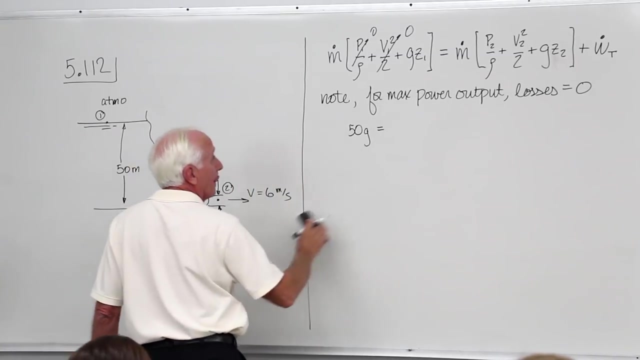 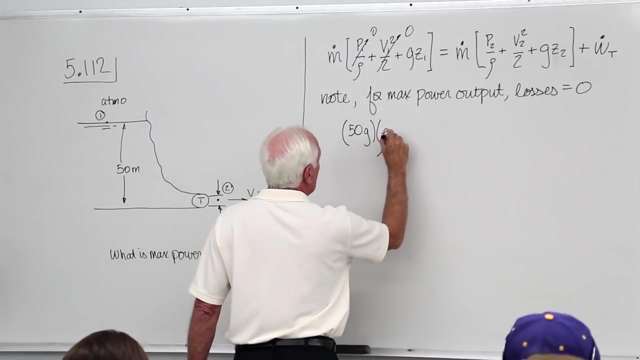 P1, atmospheric, zero V1, zero Z1, 50.. So 50 G And that's equal to R1.. Let's put our M dot. Let's put our M dot. M dot rho A V. 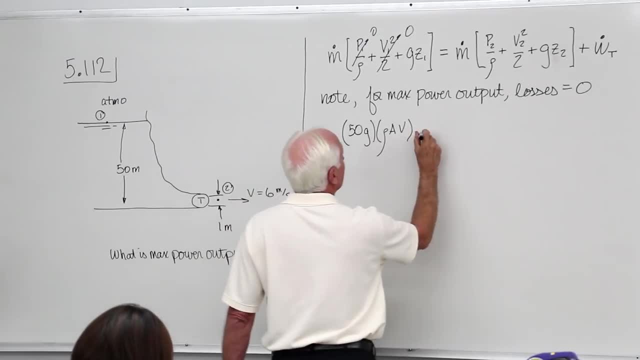 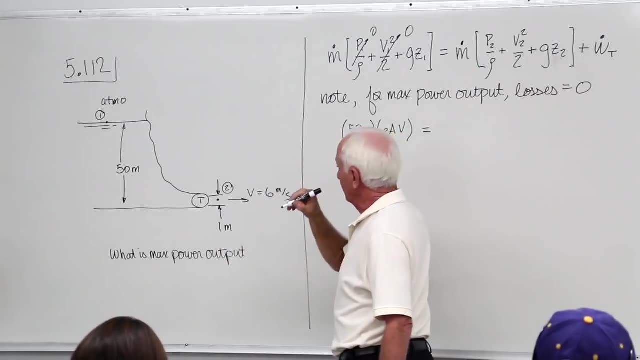 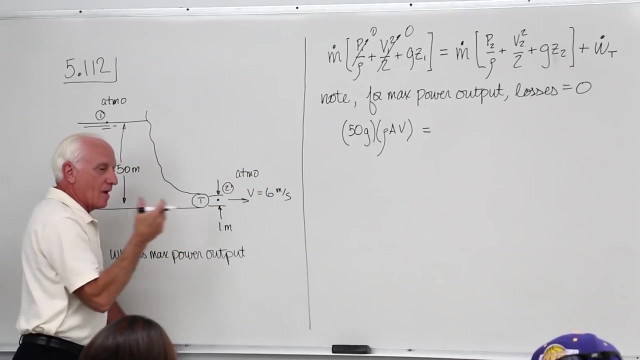 And here equal M dot rho A, V, P2 goes out to atmosphere, output atmosphere. The picture didn't show that, but you know the turbine exhausts out to it, The stream river down here, So it's out to atmosphere. 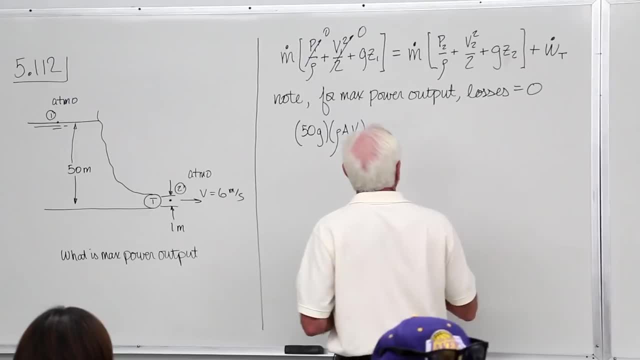 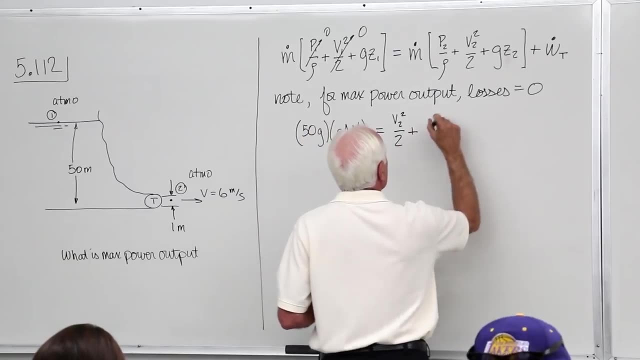 V2 is 6 given to us, So we have V2 squared over 2.. Z2 is zero. My data is at the turbine, So Z2 is zero And Z1 is 50.. And Z2 is 50.. 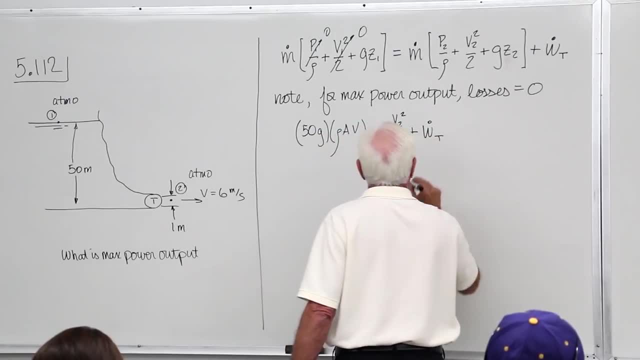 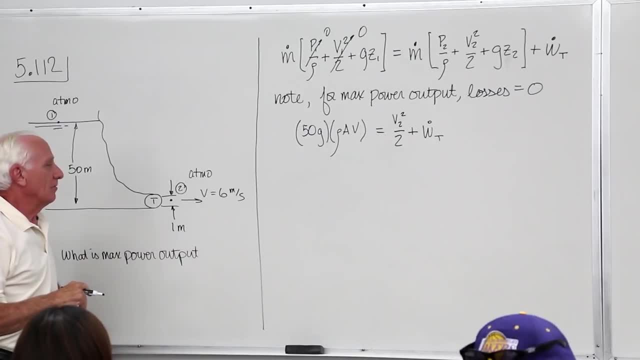 It's a 1,000.. Do I know the velocity? Yeah, it's six. Do I know the area? Yeah, it's pi D squared divided by four. Pi divided by four. Do I know G? That's 9.8, 1.. 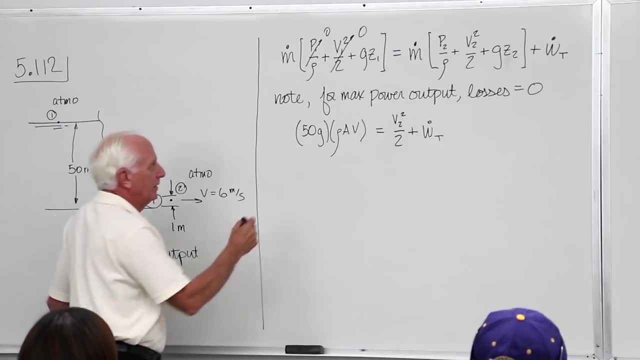 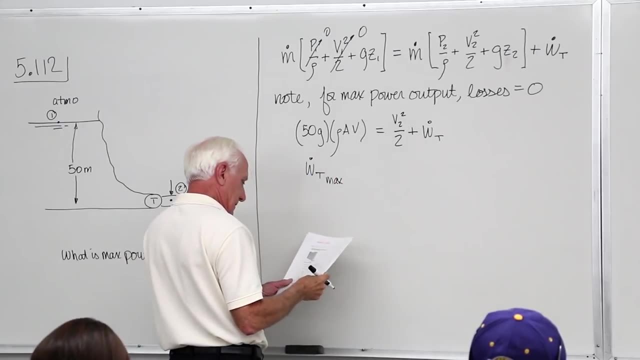 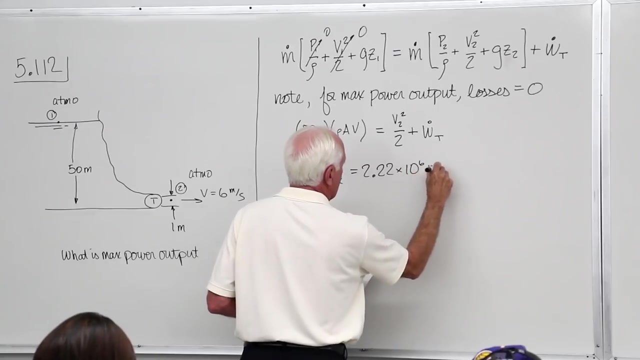 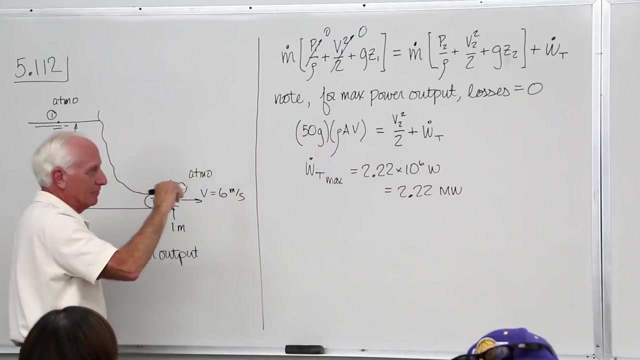 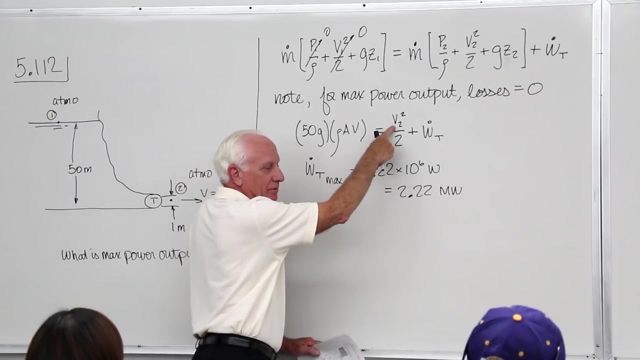 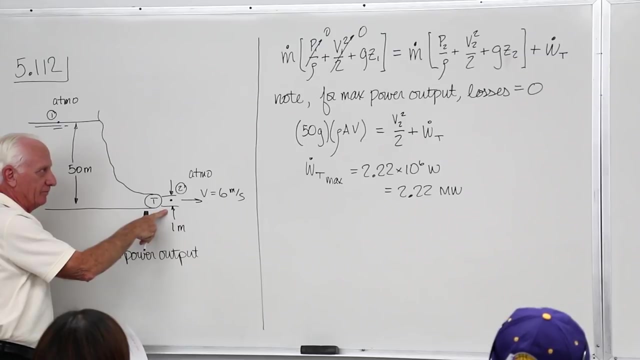 Problem solved: W dot turbine max. Great thanks, Bye-bye everyone. that's max is 2.22, 2.22 megawatts. That V in the mass flow rate is that same V, V2,? okay, Because where do I find the mass flow rate Where the stuff leaves? 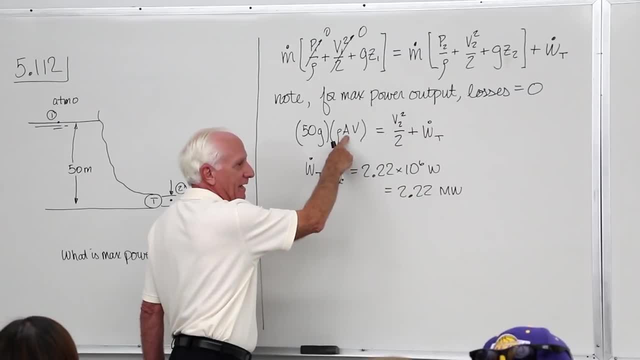 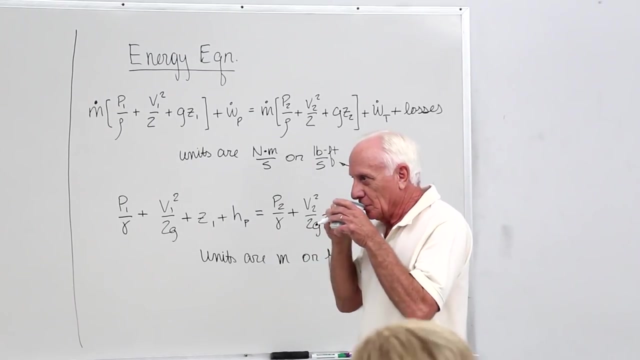 So that V is that V2.. That A is A2.. Okay, so that's the simple case where the losses are zero. When the losses are zero, it makes life easy. So what happens to that M-dol on the right? 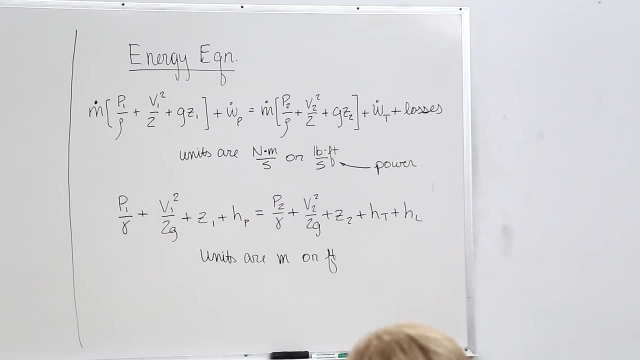 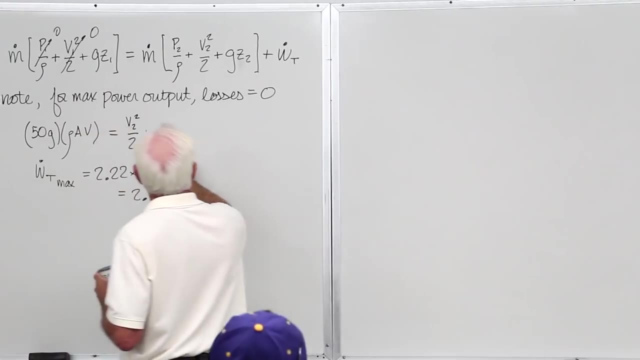 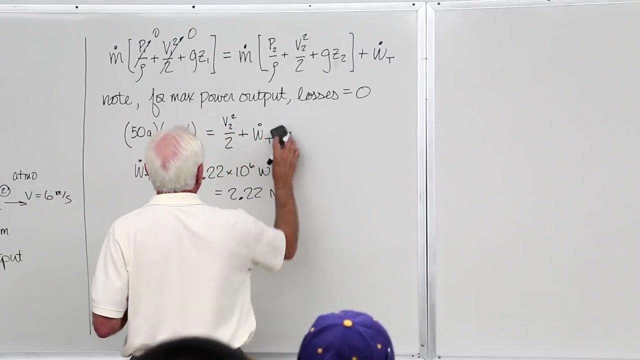 Which one? This guy? Okay, the GZ is there. Oh, yeah, we have the V2 leaving there, don't we? Well, I got there there. Which one are you talking about now? M-dot? Oh, the M-dot. Oh, okay, got it, got it, got it. Thank you, thank you And that. 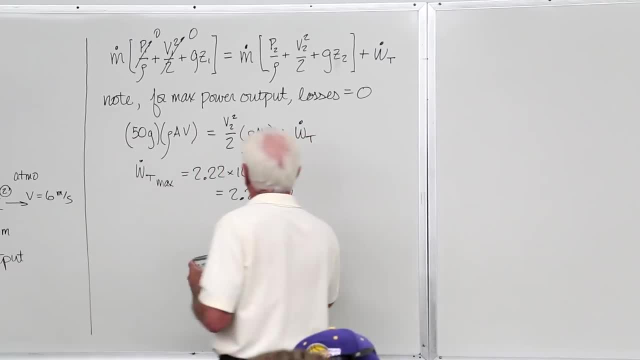 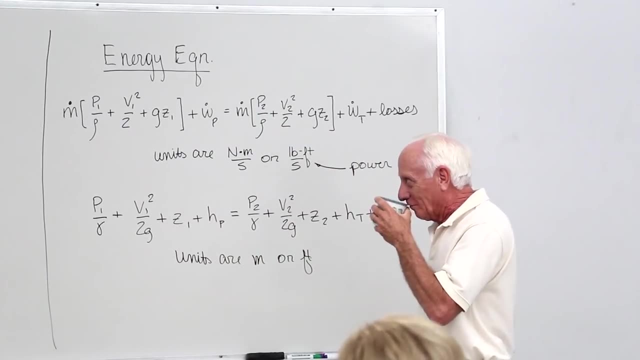 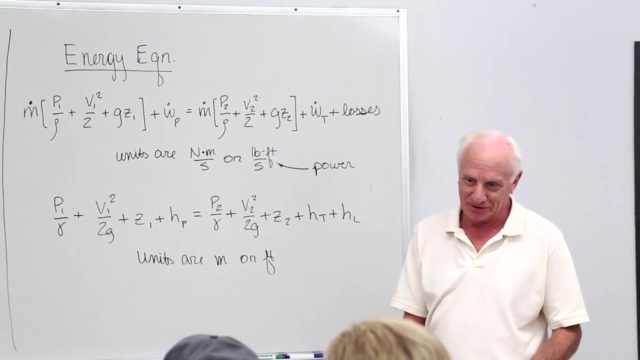 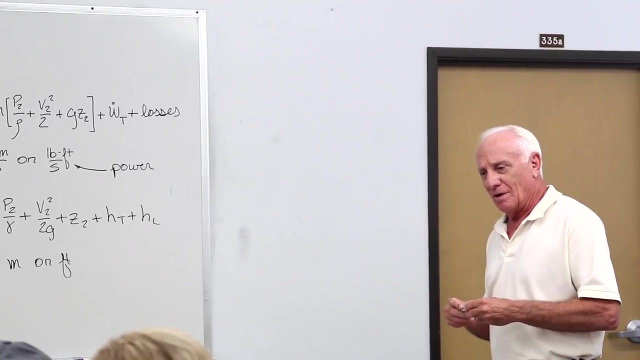 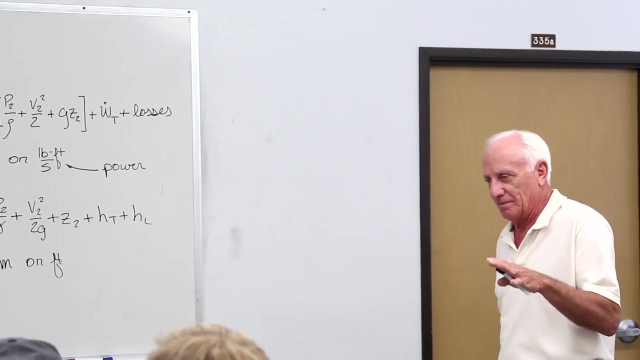 is plus times W dot T. Didn't change the answer, though. I just read the quote after: Thank you, though. Okay, so the maximum you could hope for: you'd hope for 2.22 megawatts, You're not. 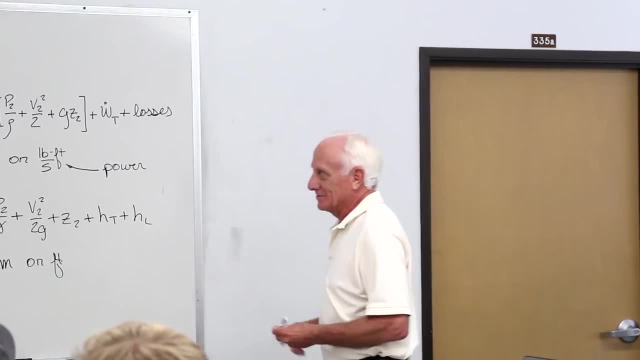 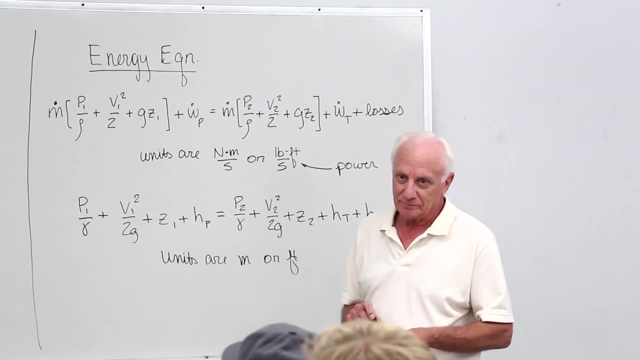 going to get it. but how close can you get it? Well, you've got to consider losses for that. Okay, sir, Uh-huh, Kind of a dumb question, but so V2 would be 6 meters per second. What about V? 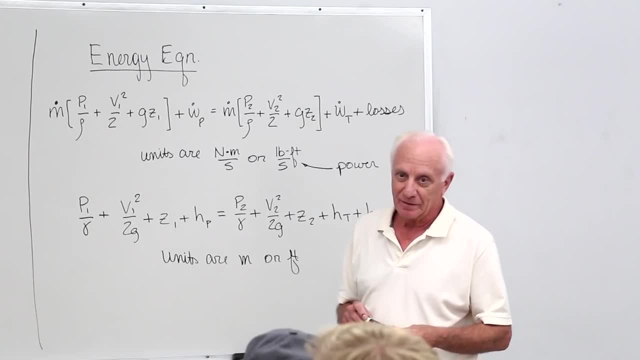 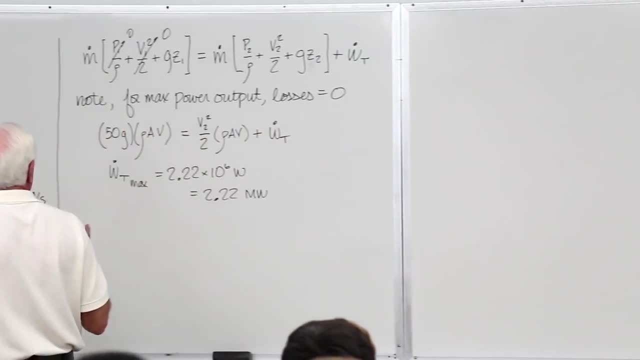 What would that be? Well, which one V. in that term there's V, and then there's V2.. That's right. So what would V be? The terms A and V or M-dot. Here's where that V would be, where you want to find that V. That's right, That's. 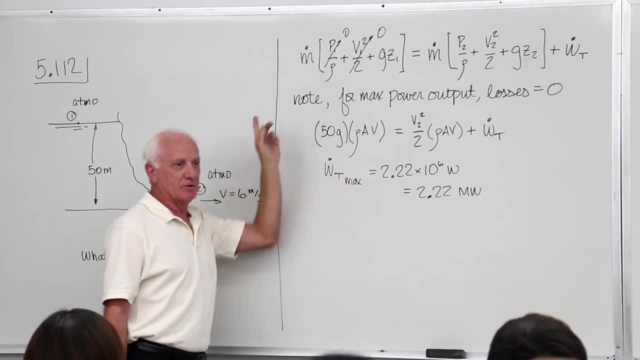 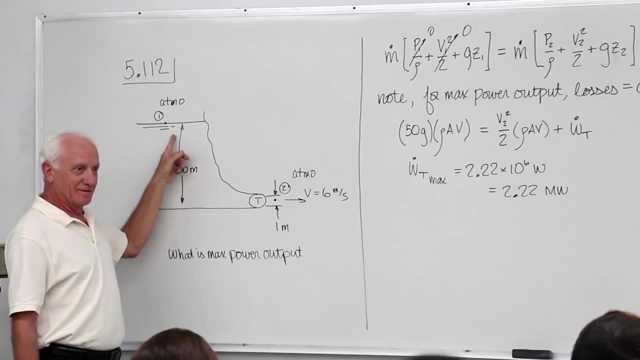 where you want to find that M-dot. So you tell me where do you want to find M-dot? Look at the picture. Where would you find M-dot? Up here at the free surface of Lake Havasu? Or down at the turbine exit? Oh, at the turbine exit. 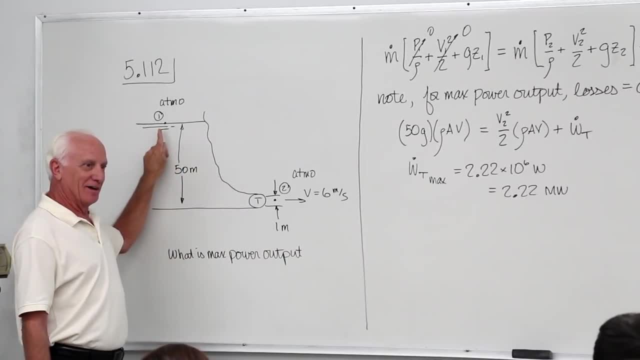 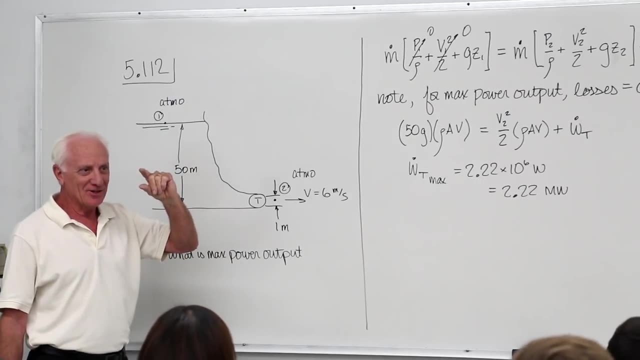 So it's the same. What's the mass flow right here? Does the level of Lake Havasu drop? Of course it does. How much, I don't know. a quarter of an inch, A one inch in an hour Do we know? 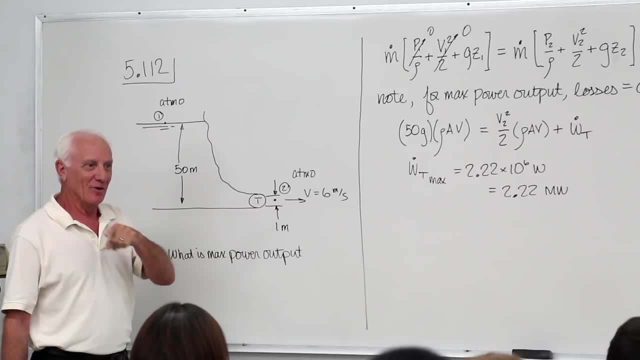 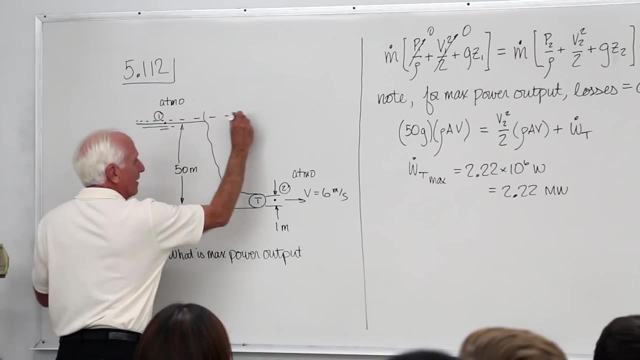 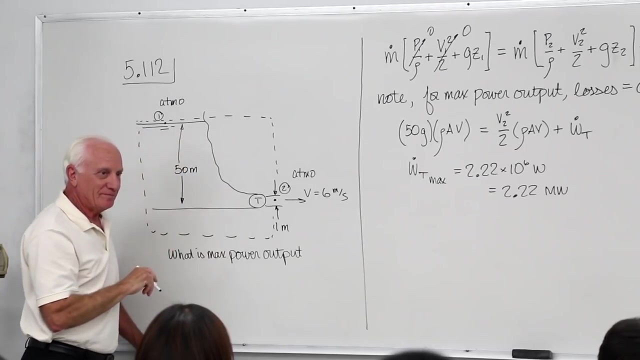 that We don't know that. So what do we take Where we know it And where do we know it At the turbine exit? If you want, don't forget, this is a control line. Alright, go ahead and draw your control line Now up here. take row A V, Row A V right here. What's? 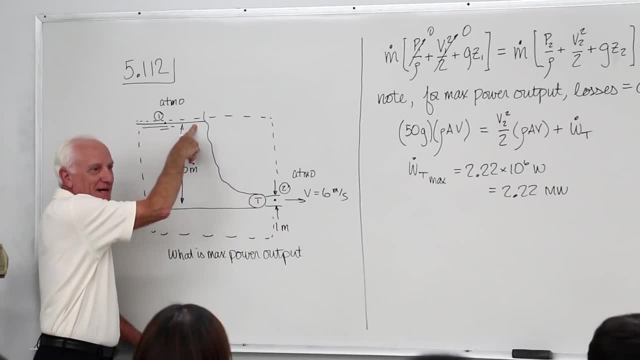 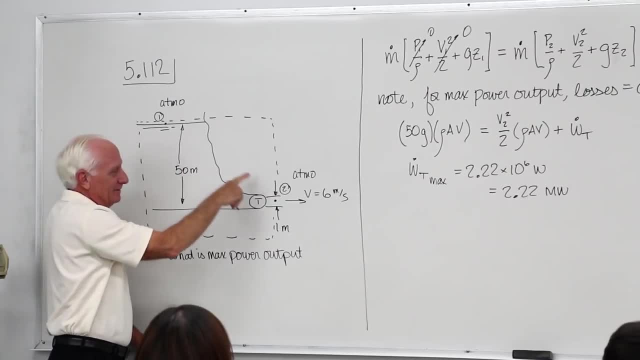 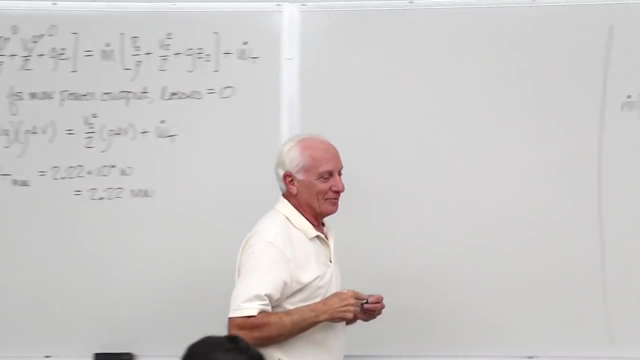 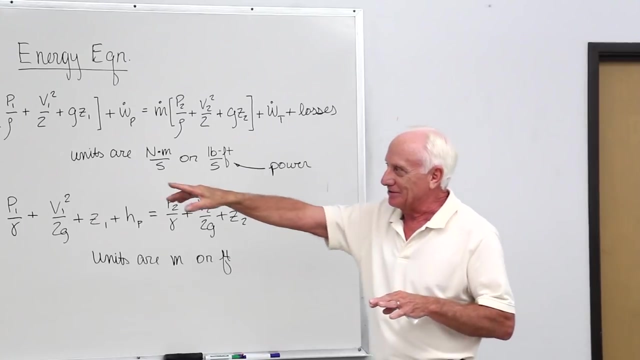 Do I know that? No, Do I know the area here? Yes. Do I know the velocity here? Yes. Take this one. We know that lake is really dropping a little bit, you know. but we're not going to look at that lake because that lake is a lot of uncertainty in it. We know what's going on at the turbine exit. That's why we look at the turbine exit. The velocity in m dot, then, is the velocity at the turbine exit Alright, 5,123.. 5,123.. 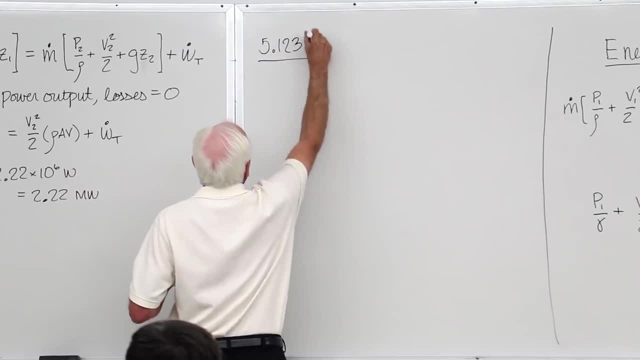 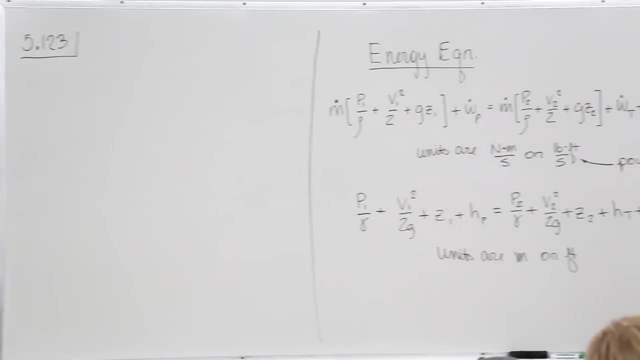 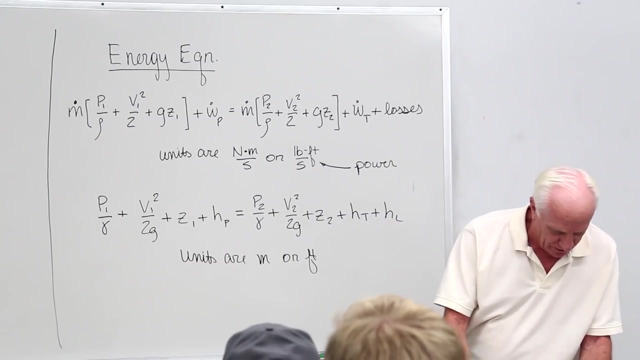 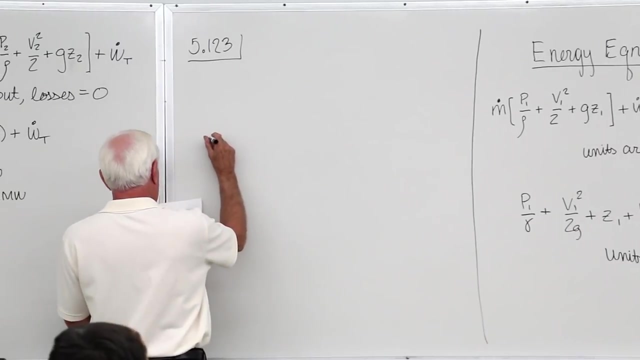 Okay, So 5,123.. Let's look at the picture in the textbook here. Okay, Water is to be moved from one large reservoir to another at a higher elevation, as indicated by the picture. I'm going to make the picture look like this. 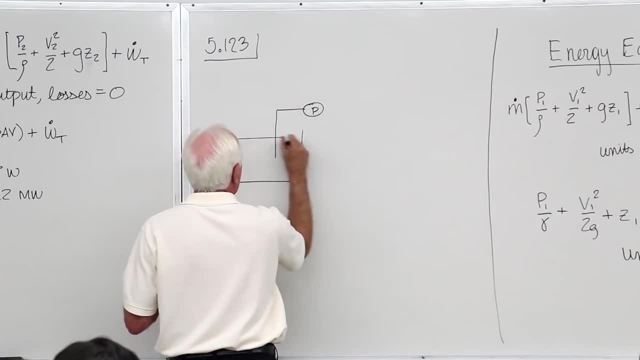 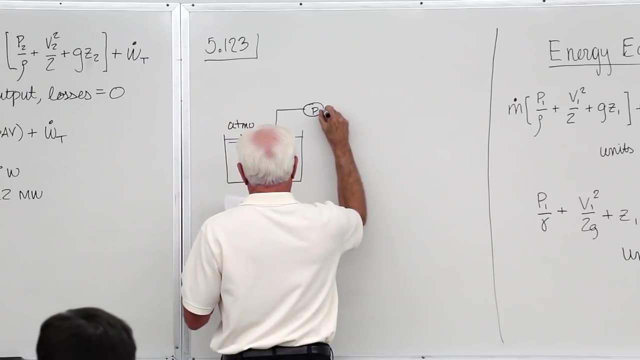 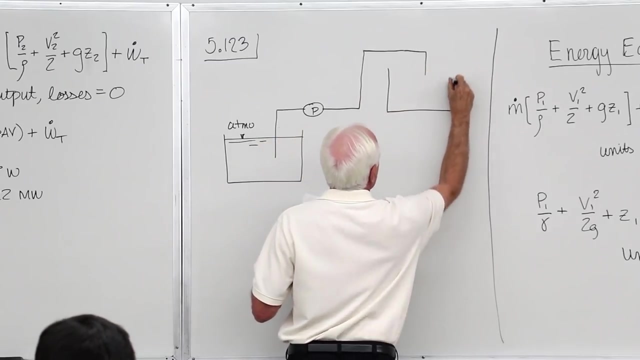 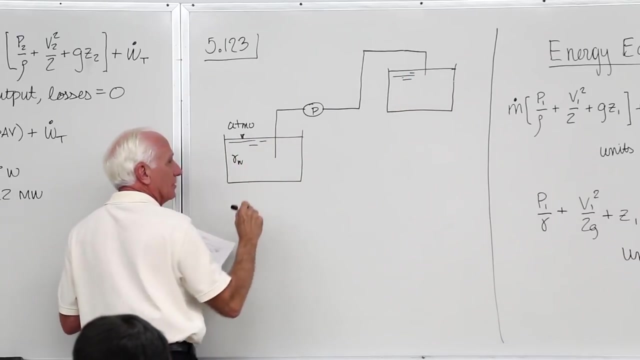 So that's essentially how the picture looks, And, of course, we're pumping the water out of the lower reservoir. Okay, So that's essentially how the picture looks And of course, we're pumping the water out of the lower reservoir. 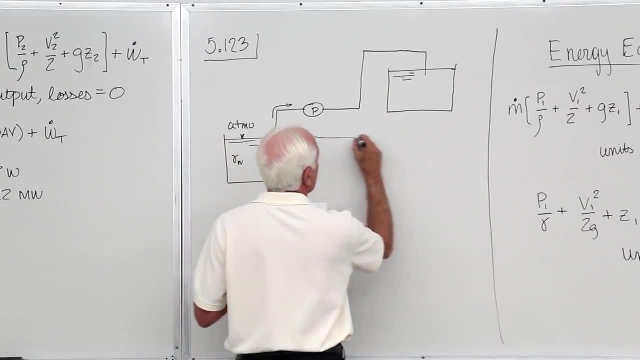 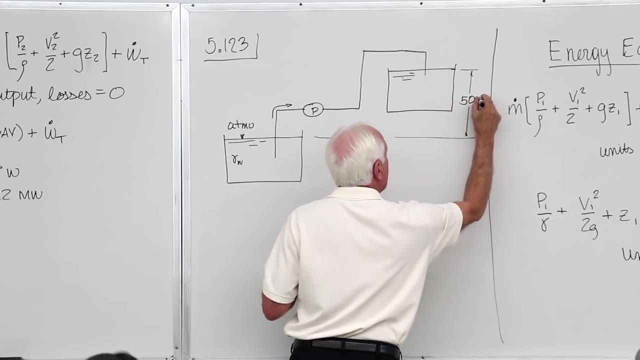 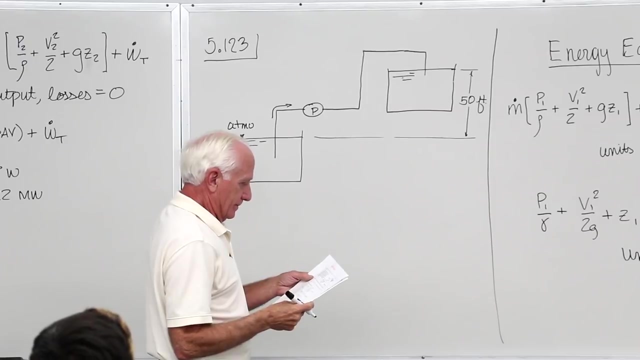 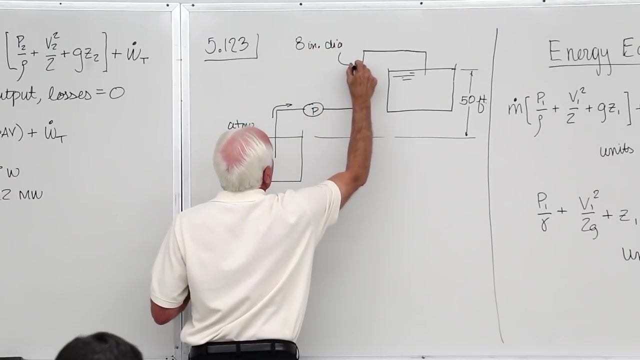 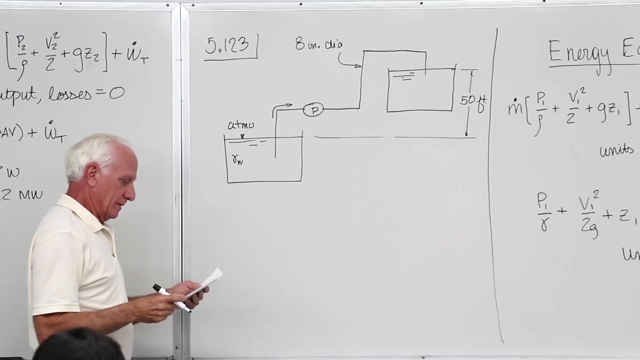 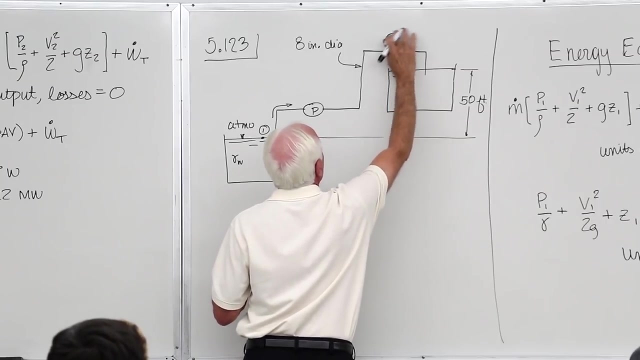 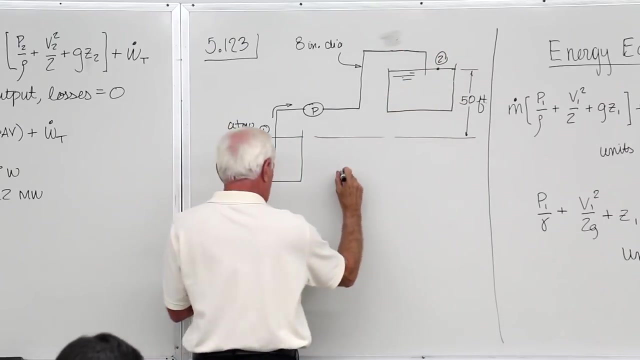 Up to the upper reservoir, 50 feet difference. Okay, Alright, 8-inch inside diameter pipe, 8-inch diameter. the losses he tells us where points one, point two are. so the losses from point one to point two: there's point one, there's point two, that's not there, point two. so losses H, sub L. 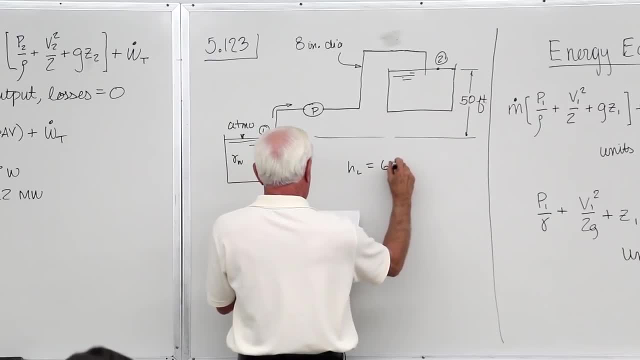 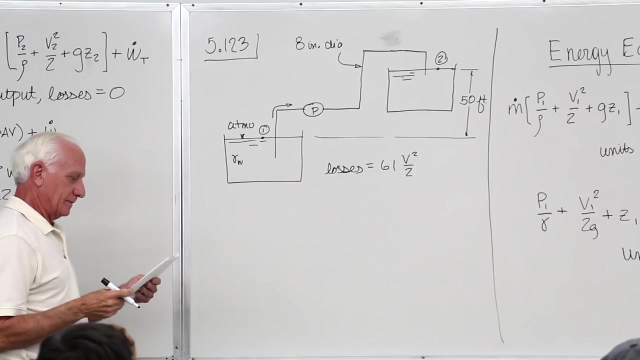 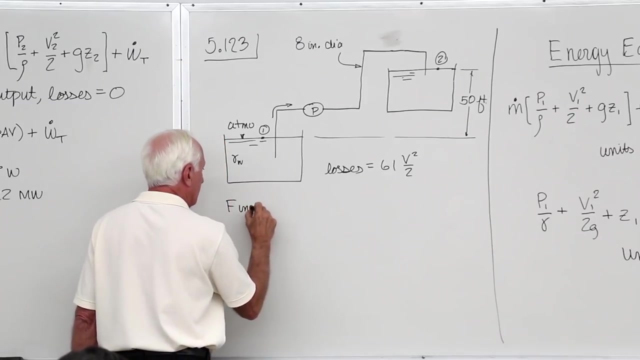 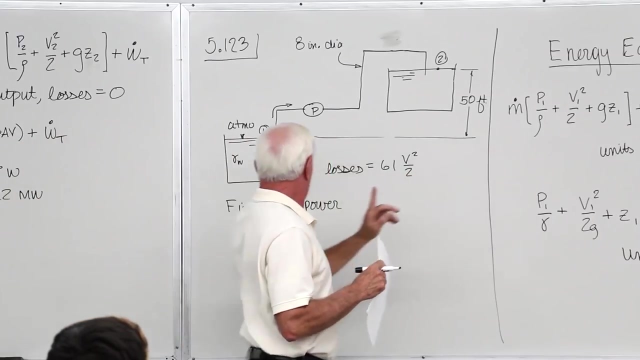 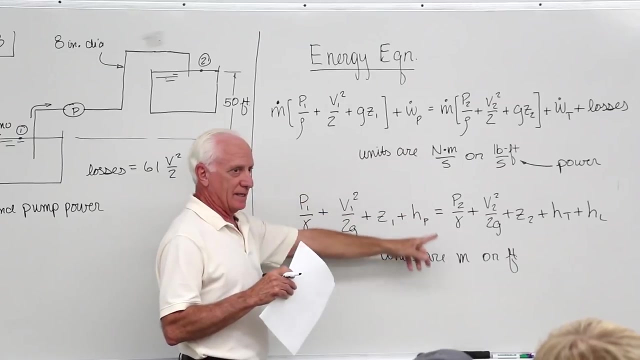 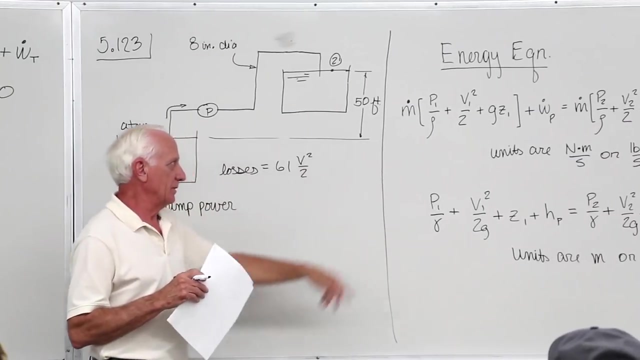 61 B squared over 2. okay, okay, find the shaft power required to do this. so find the pump power. fine, though he could, uh, once the maximum power output double 112. we chose the power from here. energy equation: what's the pump power required? we want to find the power form of the energy equation. nobody asked us to find the heck of the turbine or the head, the pump, so this one is probably not the one you can use. that's the one you can use. 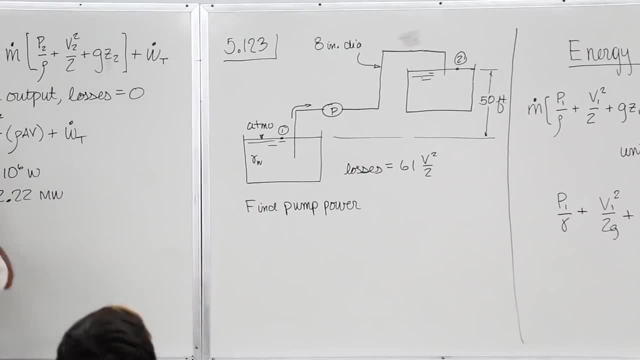 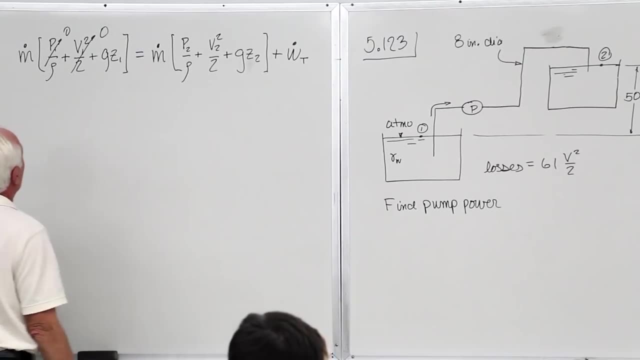 okay, let's start now. look at this here. we want to look at the turbine. so this wind had enough power that were ready. you just pulled it, paint it out and put it back in the opening circuit. let's start up here again on free surface. one pressure, zero, velocity zero. 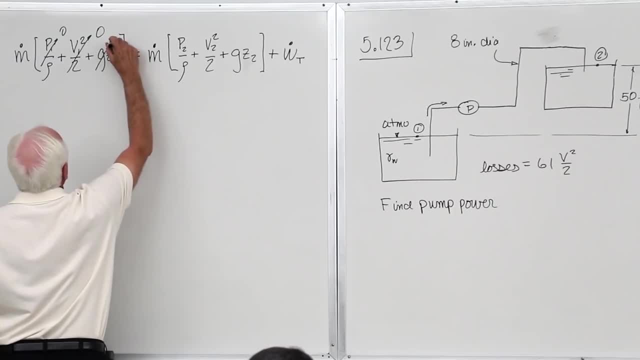 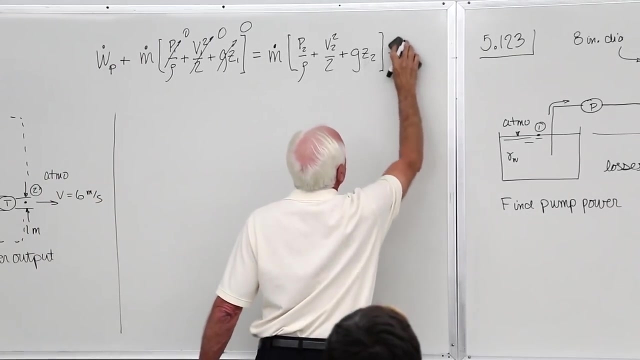 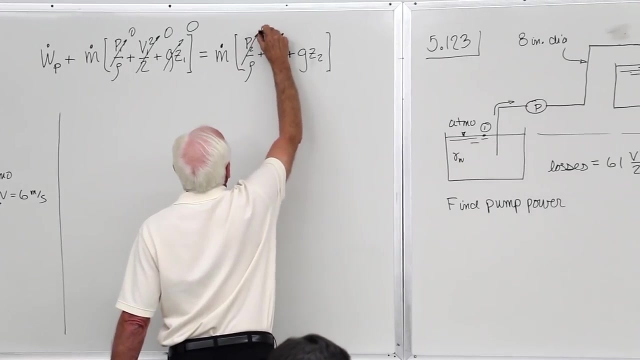 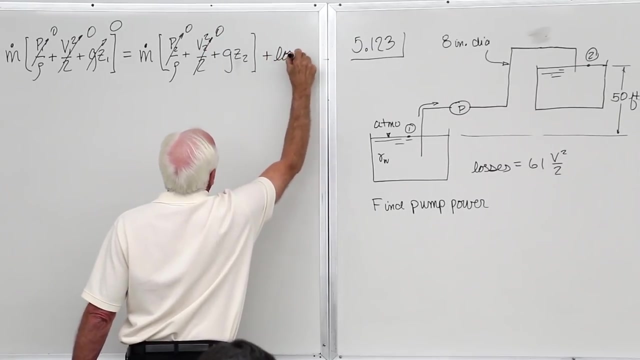 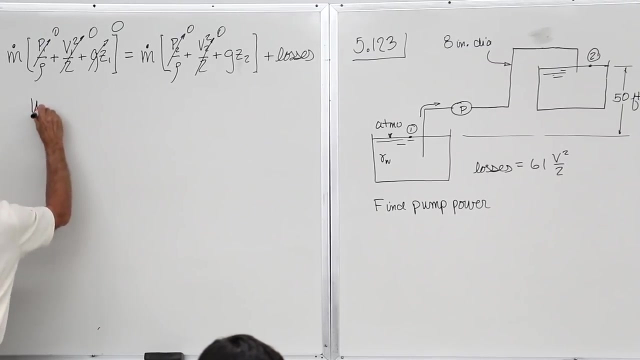 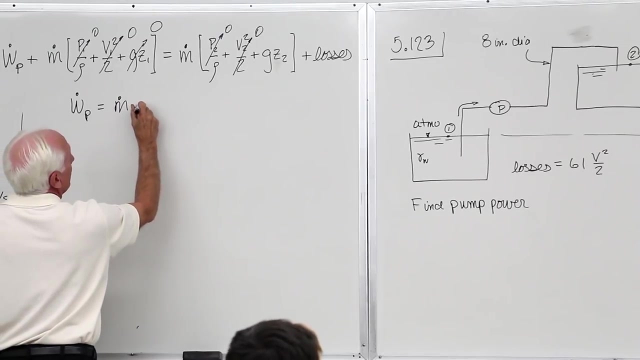 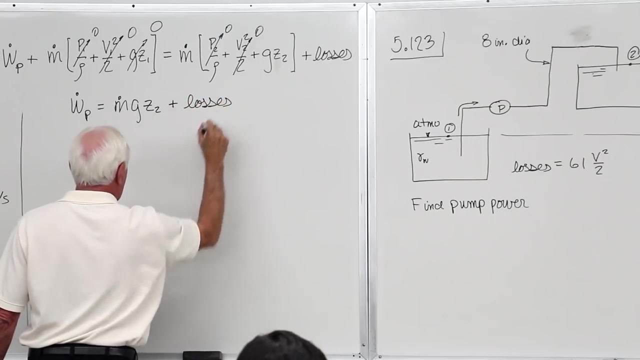 Z zero, HP, W dot P. there's no terminal. W dot T, zero reservoir to pressure, to atmosphere, zero of B to zero, plus zero losses. okay, Z to 50. so W dot pump is equal to M dot times, G Z 2 plus losses. now you told me that the losses are 61 B squared. 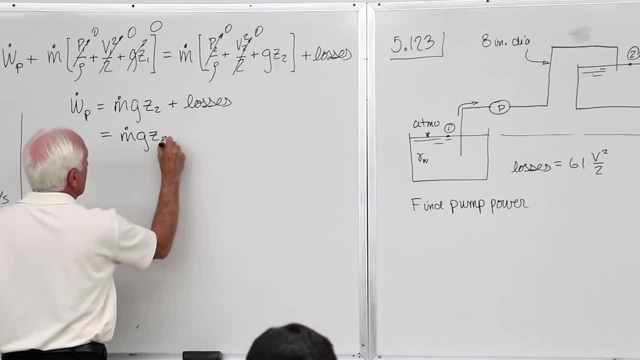 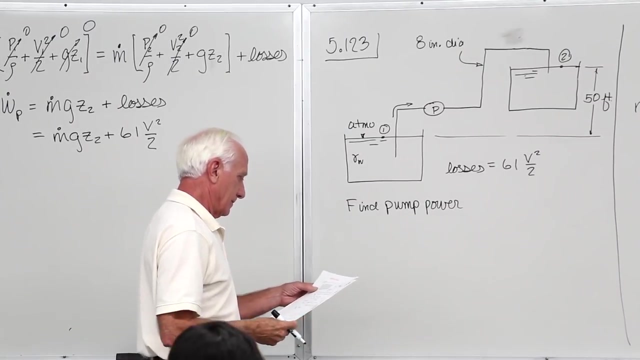 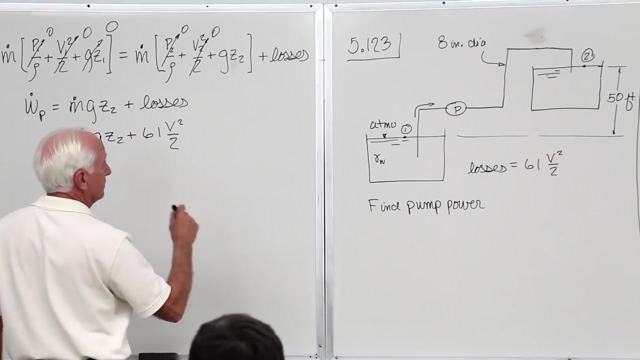 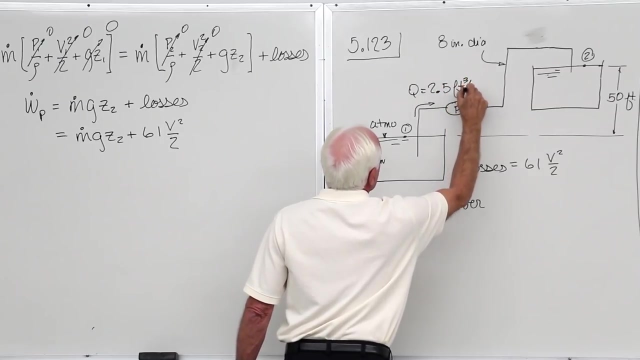 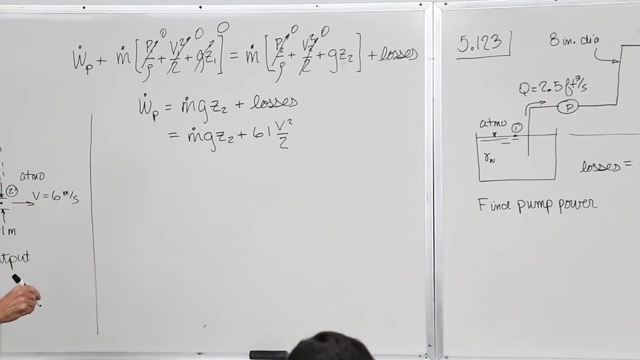 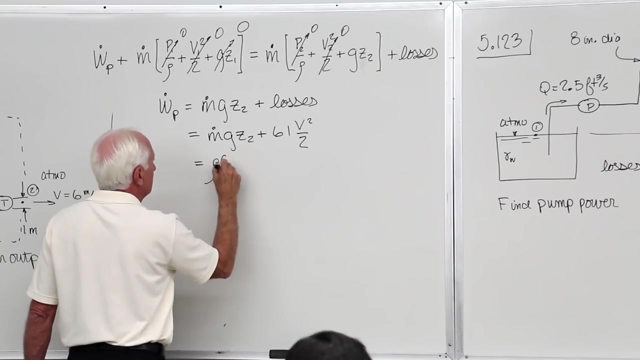 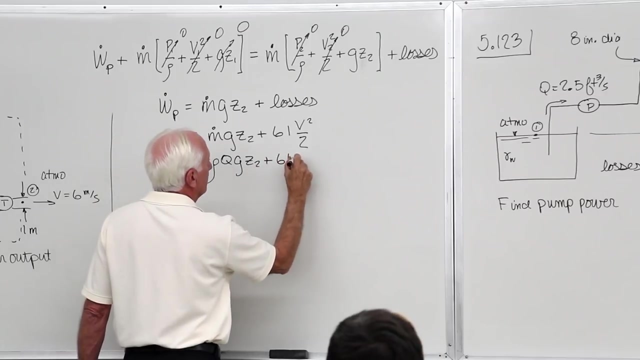 okay, okay, power required: 2.5 cubic feet per second is Q. you, you, Pues, that's how much water is water. that's how. That's how much water you want to pump from the lower reservoir to the upper reservoir: 2.5 cubic feet per second. This is just s own water. so you P-Min 3 and Menu 12 by mM dot is Rho times Q плюс 61 P squared over 2, where V is equal Q over A, and Rho times q plus 61 V squared over 2, where V is equal Q over A. 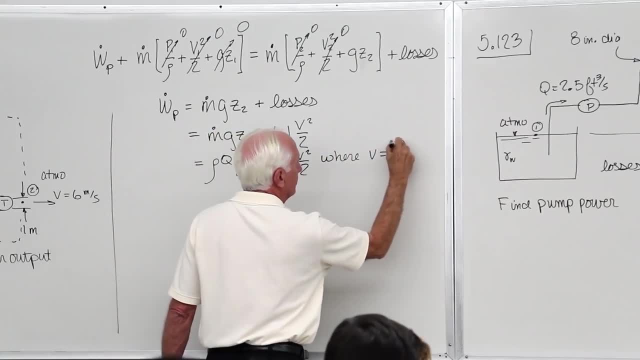 vale. yeah, That's tight. that's how much water you're going to pump from the lower reservoir to the upper reservoir. 2. M dot- herbs. M dot is Rho times Q plus 61 V squared over 2 inches, plus 61 V squared over 2 when V is 2 times the denominator. 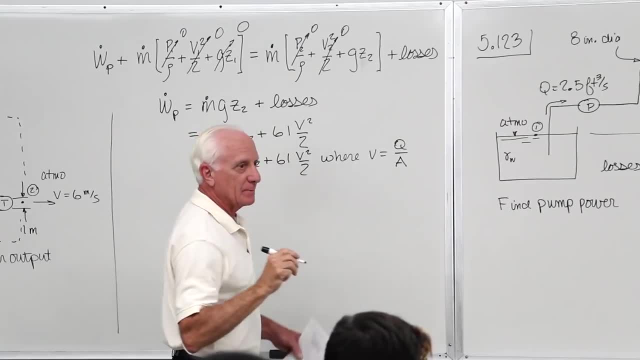 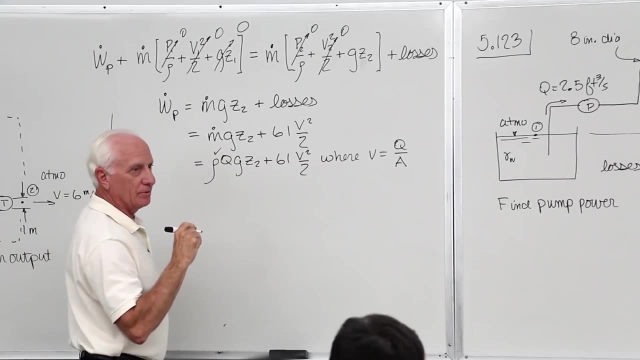 Q over A. Okay, Do I know rho? 1,000.. Do I not 1,000? in this case, put in slugs? we're in British gravitational now Slugs. do I know rho? Yes, Do I know Q Given Do. 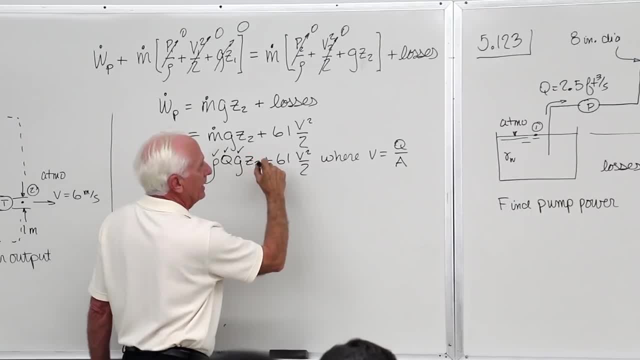 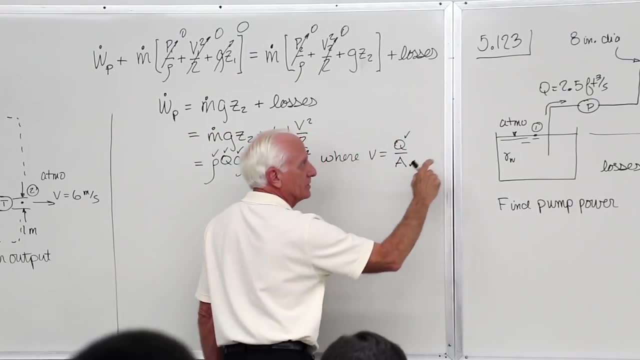 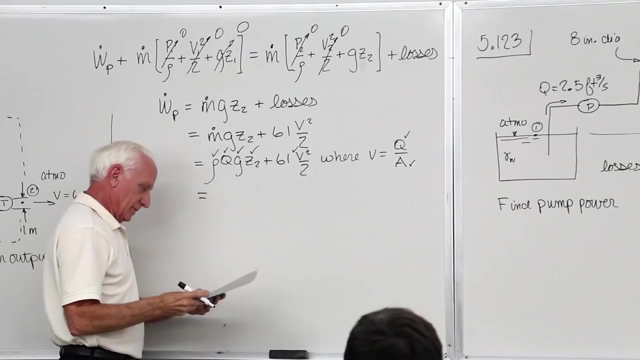 I know G: 32.2.. Do I know Z2? Yeah, 50.. Got it. Do I know Q? Yes. Do I know A Pi over 4 D squared? I know D- Got it. Got it. Everything is known. Put it all in there and you get. 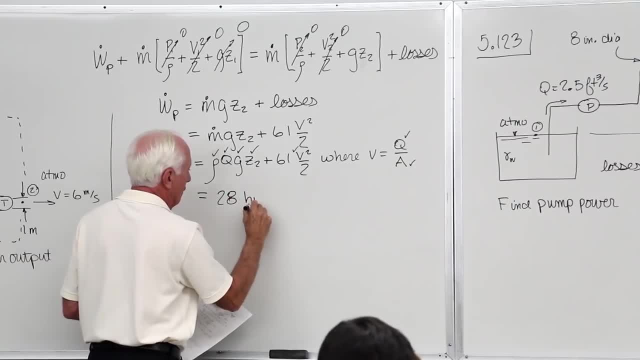 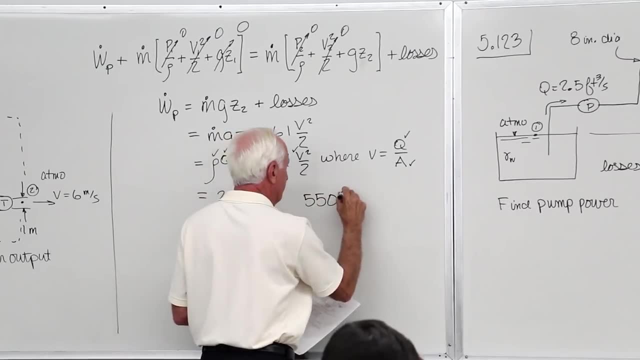 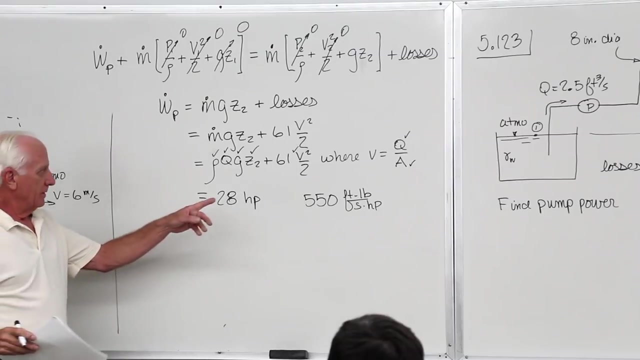 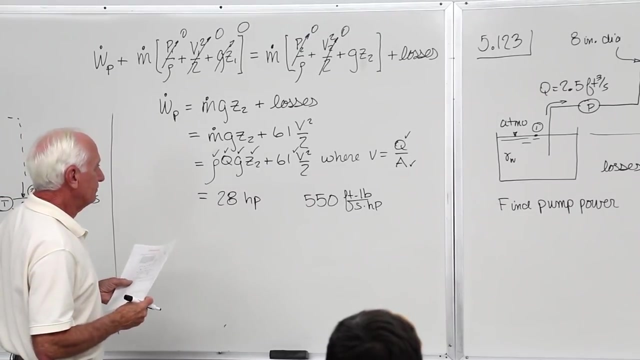 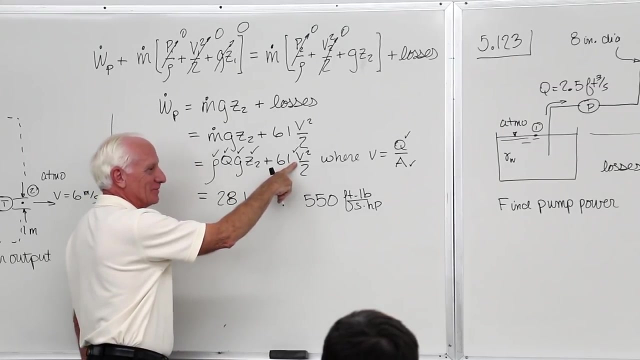 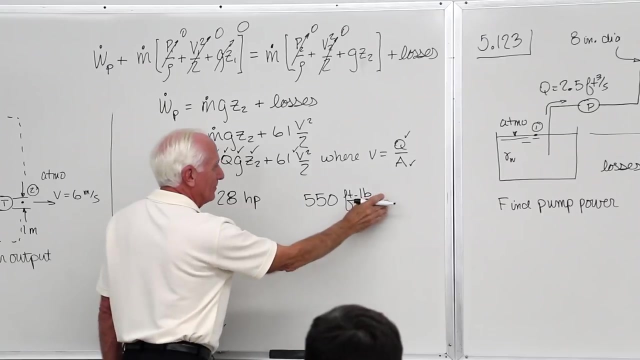 28 horsepower Conversion factor. This guy's going to come up to be foot pounds per second. Foot pounds per second. okay, Remember, remember again. What's this guy here? This guy here is square feet, Square feet, Perfect Feet squared per second squared. Okay, That's the same thing as foot pounds. 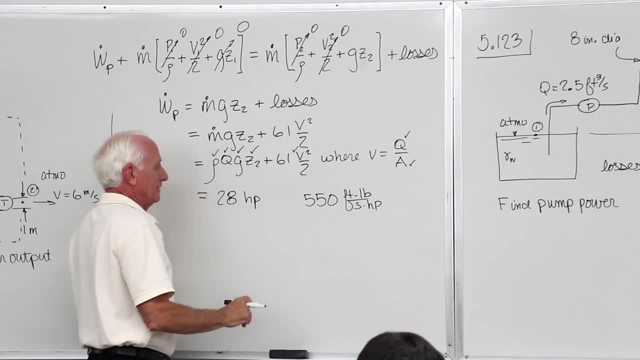 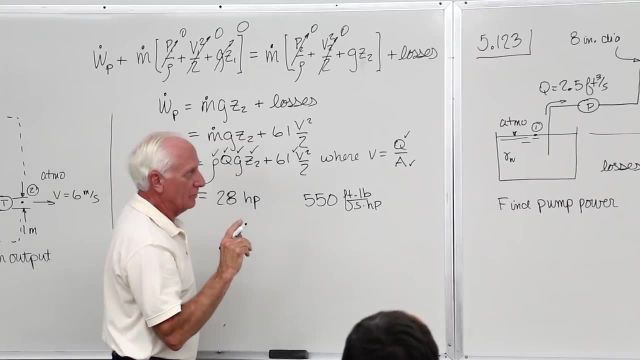 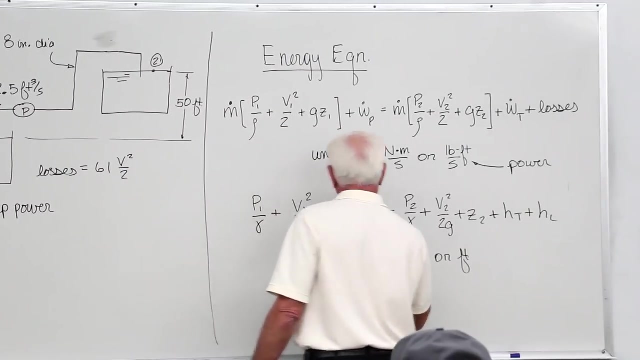 per second. Okay, Divide that number you get up here. Divide this number here by 550.. Be careful too, Don't get confused. There's two HPs and boy. you better watch your P's and Q's, Okay, Because one stands for horsepower and one stands for head. You better make sure you. know what the subscript, what not the subscript? H sub P is the pump head. HP stands for horsepower, So just be careful. It can be confusing again when you're under stress of an exam. Okay, Okay, So he gave us the losses. Nobody gives you the losses. You're the engineer, You're. 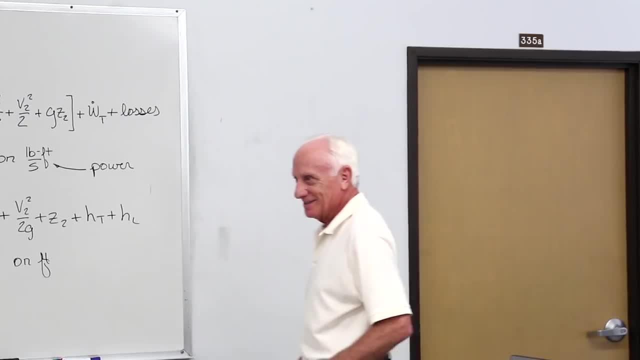 supposed to find them. We'll do that in about 10 days or so. So we'll find those losses, But for right now, we're going to do it in about 10 days. Okay, Okay, Okay, Okay Okay. 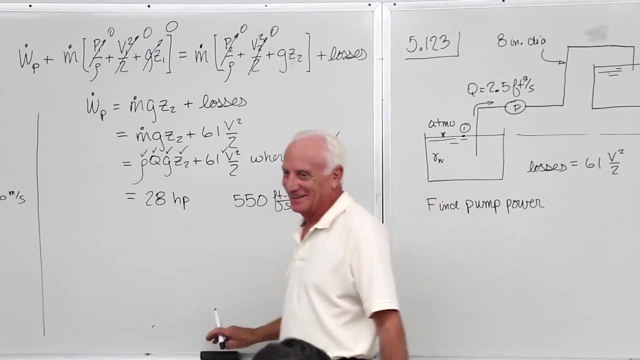 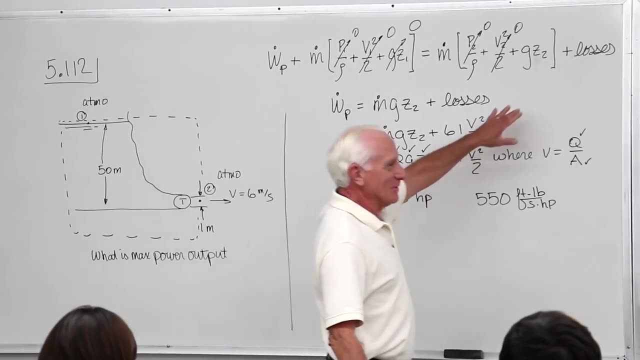 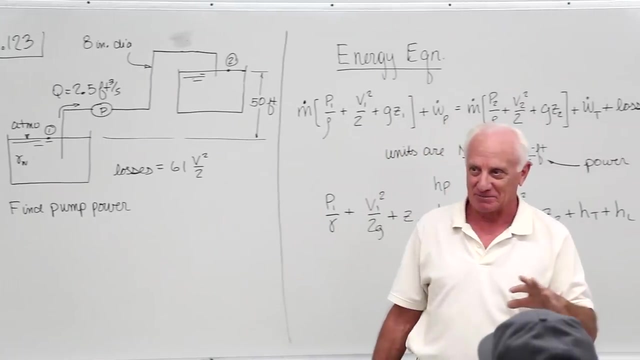 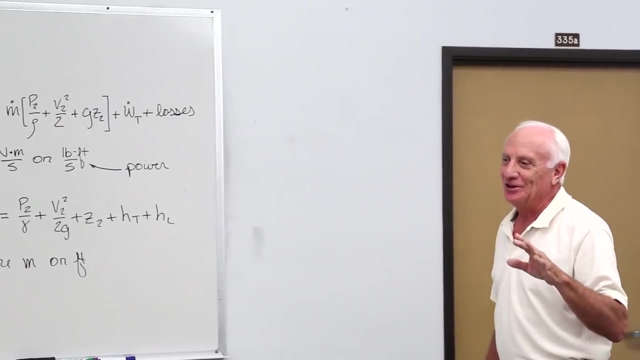 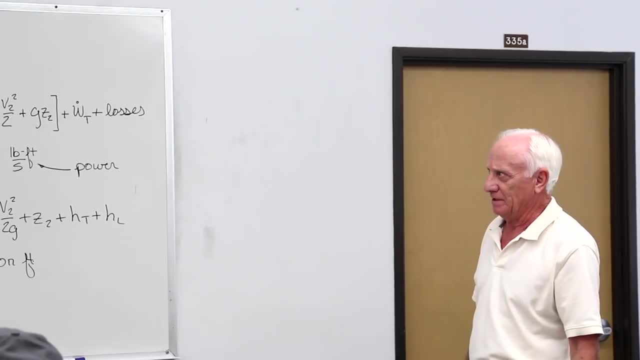 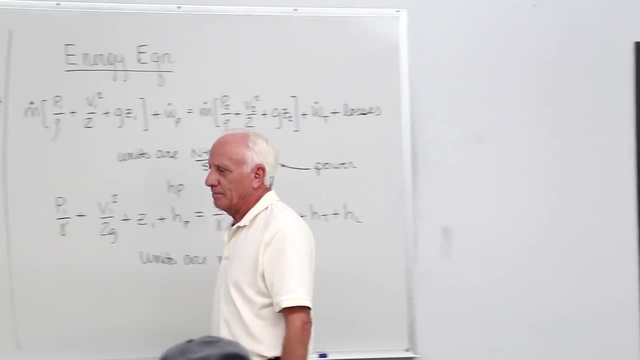 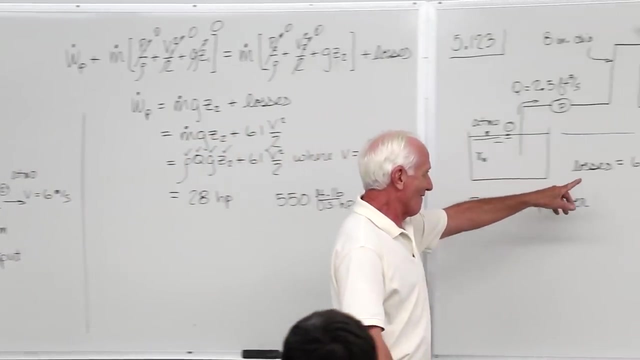 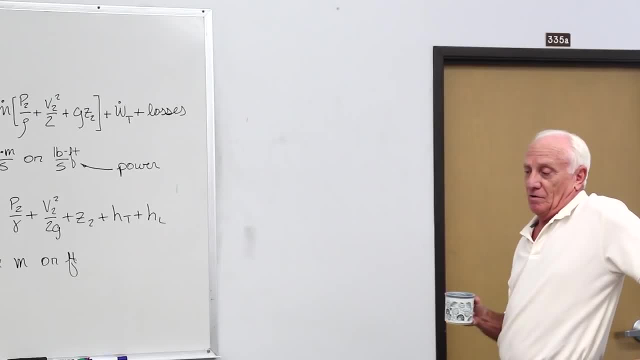 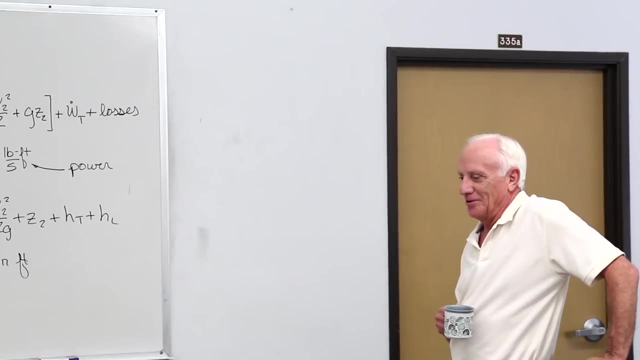 What's the pipe made of? How long is the pipe? You think a one-mile piece of pipe has more loss than a one-foot piece? Of course it does. It makes kind of sense. So yeah, all those things affect the losses. 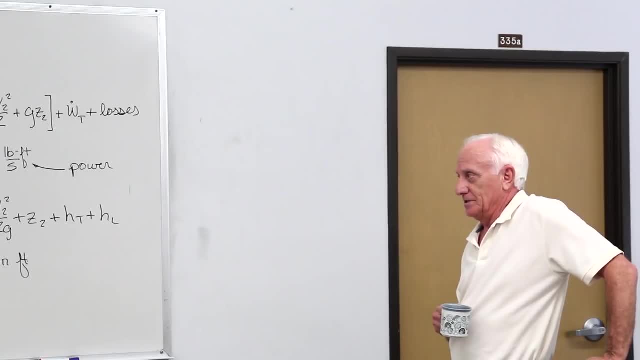 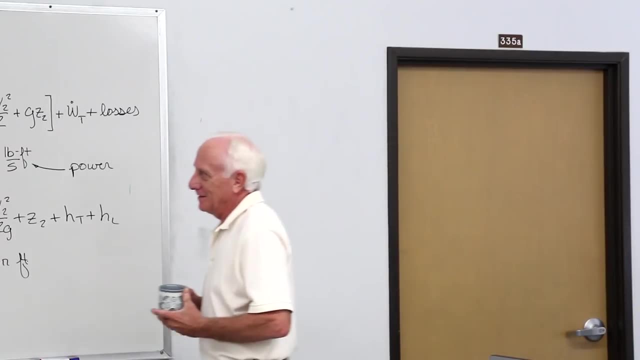 Are there right angle bends in there? Is there a swing check valve in there? Is a gate valve in there half open? All those things add up on the losses. So we're going to find out in about 10 to 14 days how we find an equation. 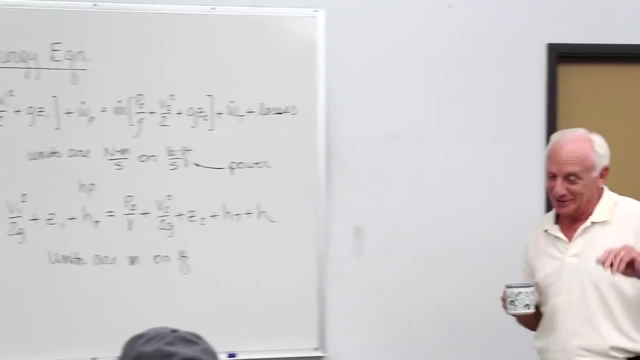 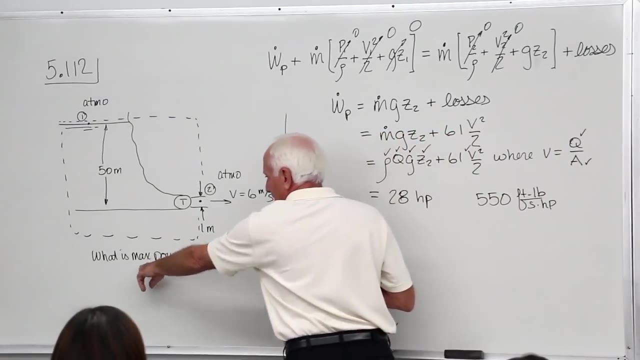 like that where it comes from. So for right now, though it's given to you. typically, What was the first problem given to you? The losses were zero. You have to understand that. Maximum power Output. What if this problem here says: 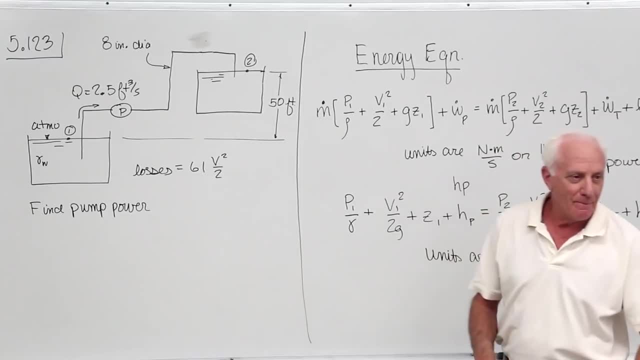 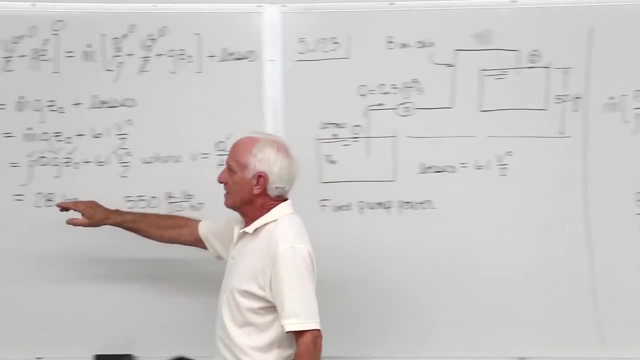 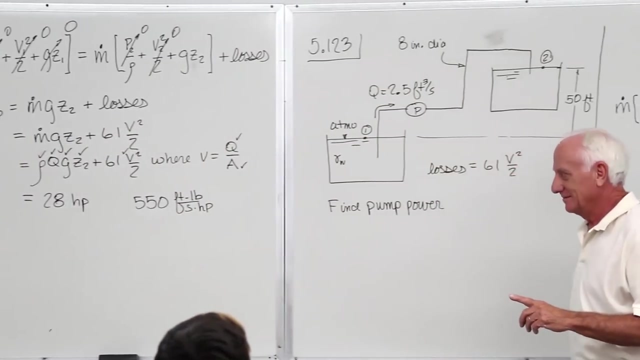 what is the minimum pumping required? The word minimum, that means the losses are zero. Minimum, What if the problem says the maximum turbine output, the losses are zero. But what is the word minimum and maximum? The minimum pump power required would be no losses. 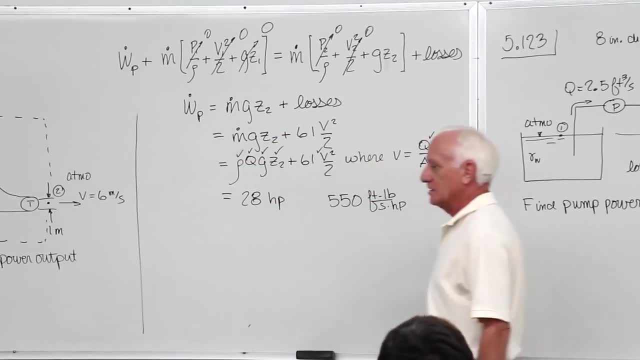 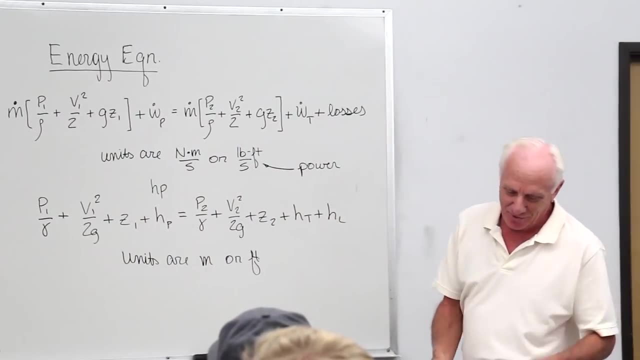 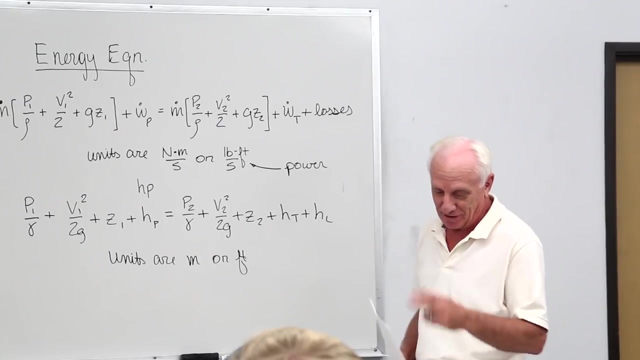 The maximum turbine output would be zero, But the word minimum and maximum means something Okay, so that's what your homework is all about And that's what's going to be due on pretty much on Wednesday, except for the first two problems that are in this set. 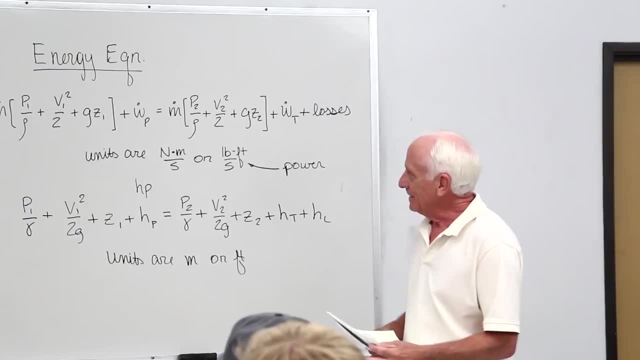 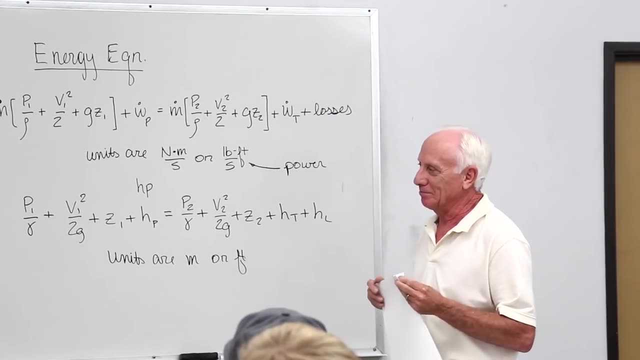 the last two problems in this set right here, Okay. so anything on that right now other than what's up there? Okay, there, if you've worked for Newly's, this is a pretty simplistic next step forward. You throw Really two terms in. 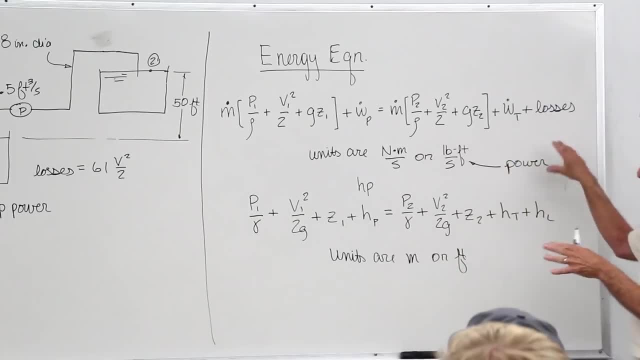 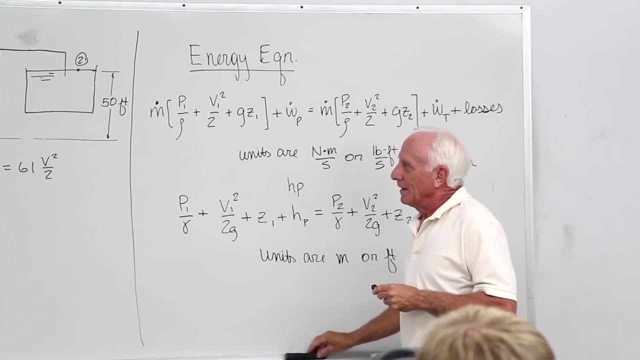 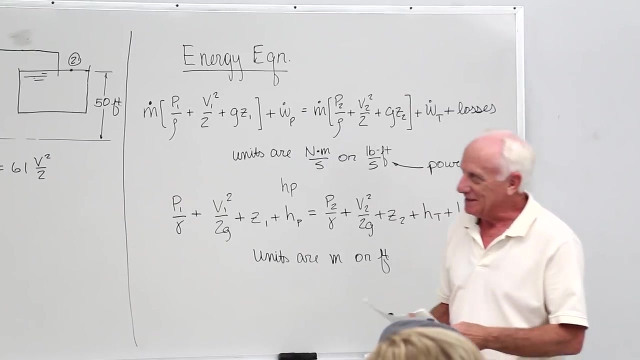 Power terms and losses. That's all you do is. that's why it's called a modified for Newly. okay, It's not totally new to you. Okay now, as we said, that pretty much is going to be the end of chapter five. okay. 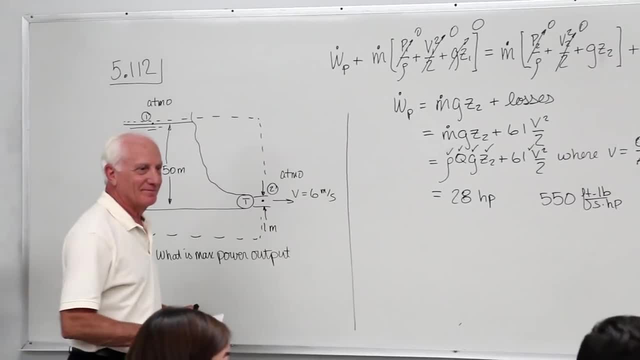 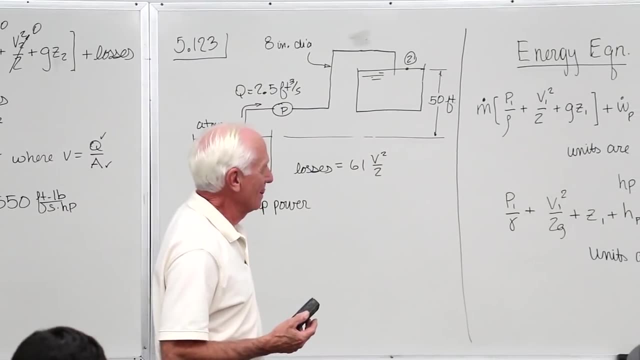 That's right. I know Just before we move on For energy, For energy equation, like we account for the pump and the turbine and so we have the losses, but for shaft work we'd actually subtract loss in there. 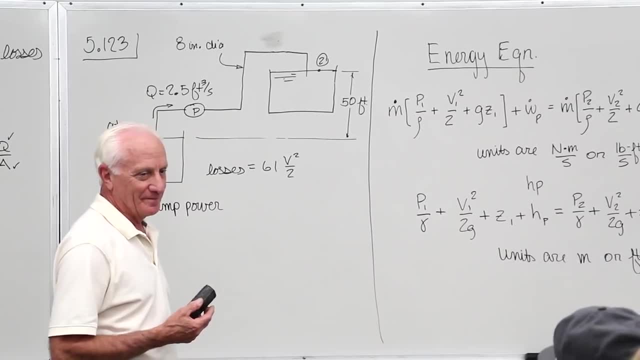 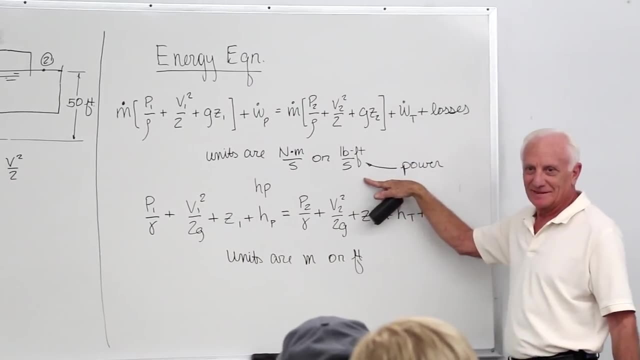 Where in there. No, when we do shaft work, I mean it's just in my notes, This is shaft work here, This is work for time. So that's what we're looking at, right, Because we might be wrong with it. 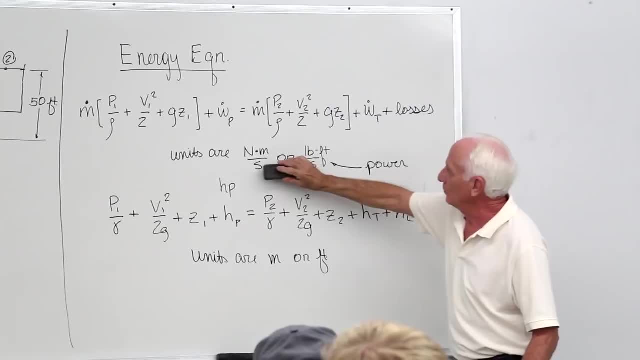 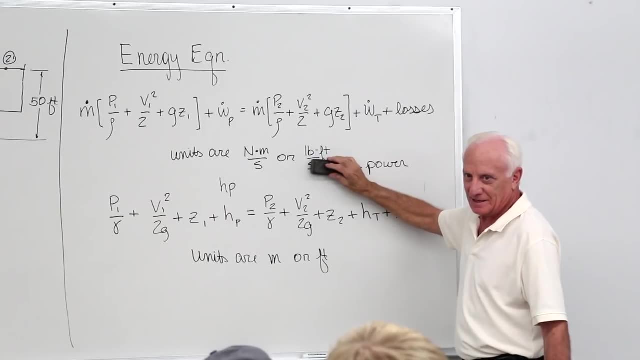 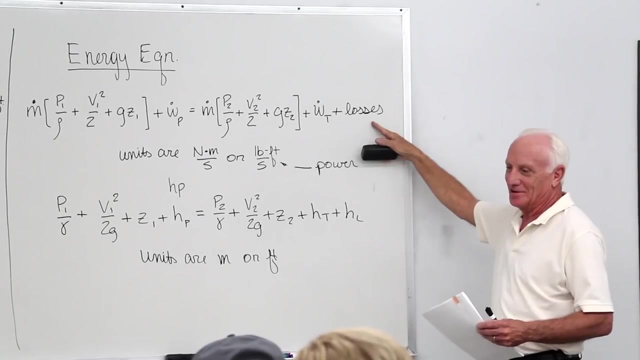 Yeah, yeah, no, This is shaft work. Work is Yeah, Work is pound feet. Force times, distance. Force times distance divided by time. is power Loss after loss. Okay, losses Are the losses in the piping network connecting points one. 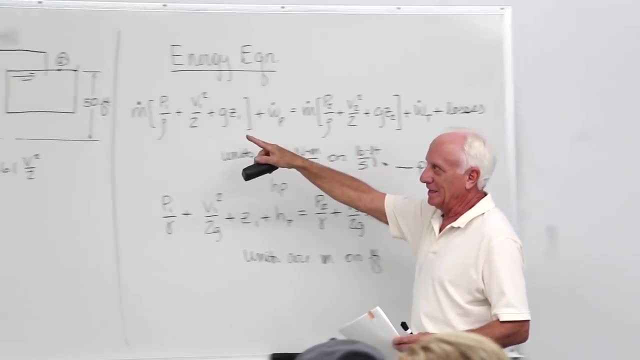 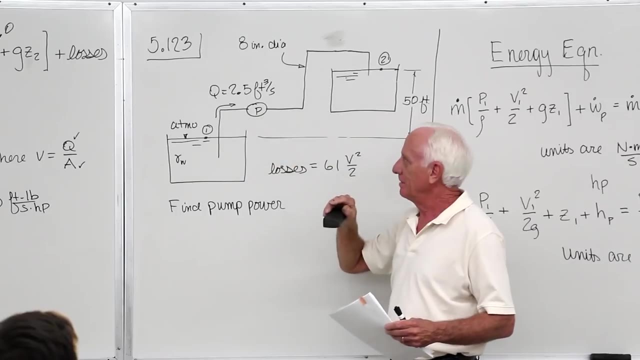 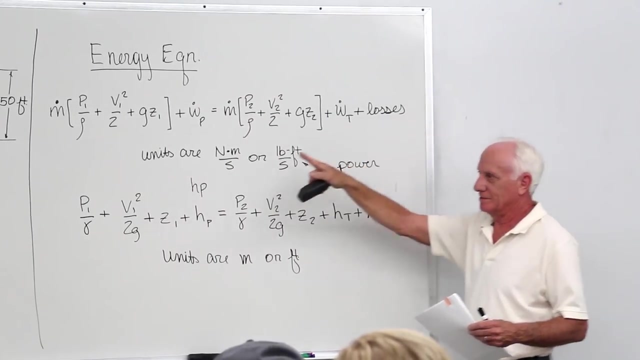 and point two in my diagram: How many elbows are there? How long is this pipe? What's this pipe's diameter? What's this pipe made out of? All that stuff there? It goes into this loss term, right here, This loss term. 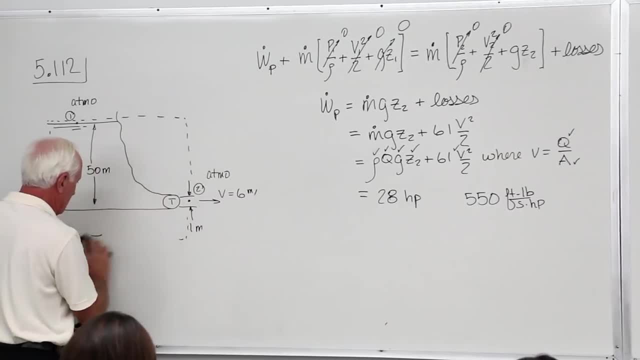 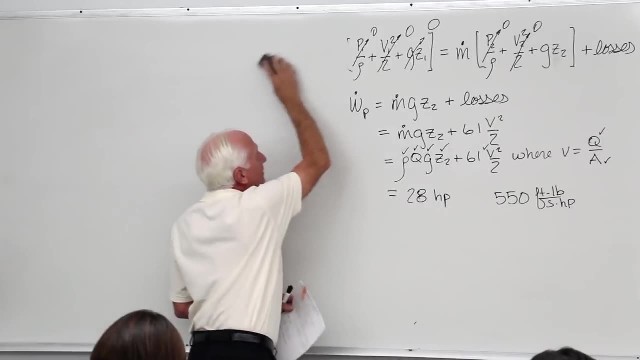 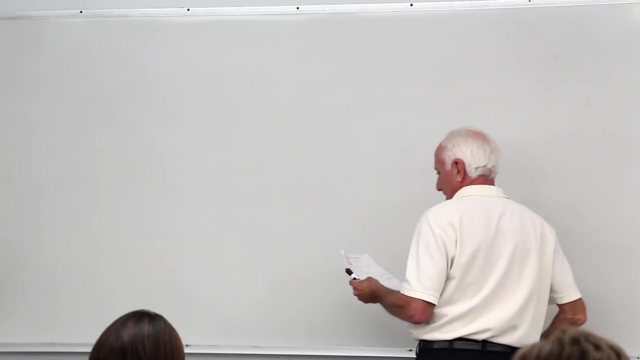 Okay, we're going to briefly touch on chapter six before we get into the last chapter in our course, which is chapter eight. We cover that after the midterm, All right, so let's take a look at the first part of chapter six. 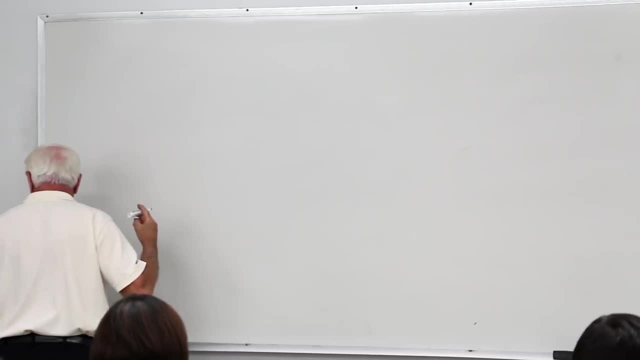 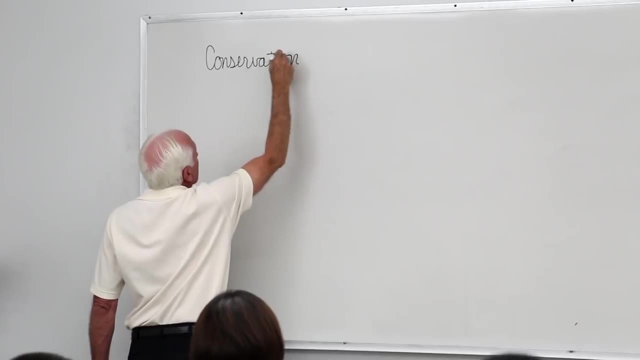 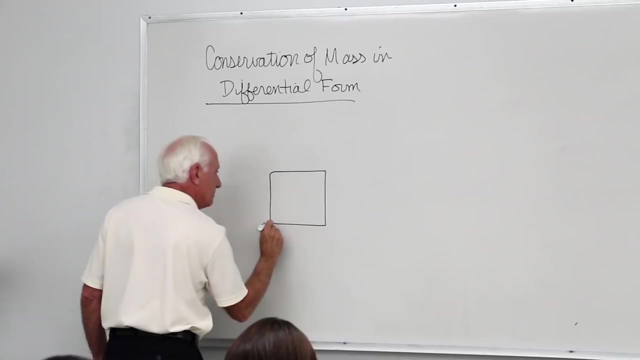 We go back to conservation of mass, Conservation of mass In differential form. We start out with a small element of a fluid. The element is dx, length in the x direction and dy in the y direction. okay, In the middle the velocity is assumed to be u. 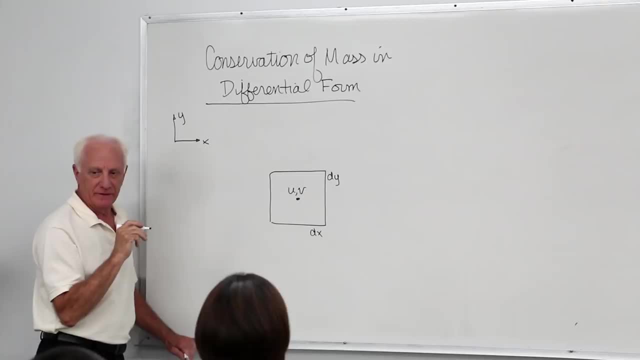 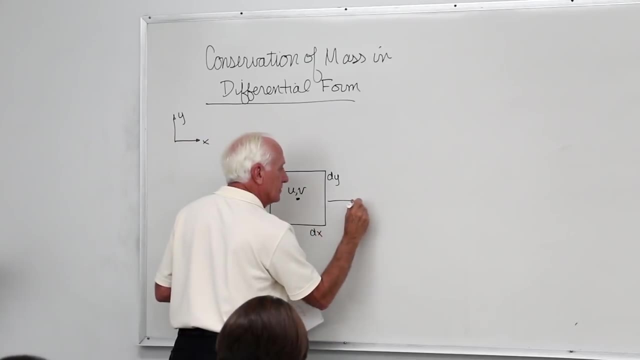 in the x direction, b in the y direction. We talked about little u, little b. On this side we have mass coming in Here. we assume mass going out On the bottom. we assume mass comes in. We assume mass goes out. 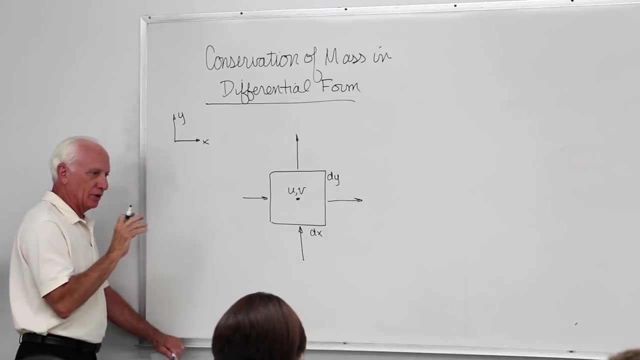 We're looking at the mass that goes in and out of this small little element of fluid: dx by dy. What comes in the left Rho times u, minus, because we went in the minus x direction- minus partial rho u with respect to x times dx by dy. 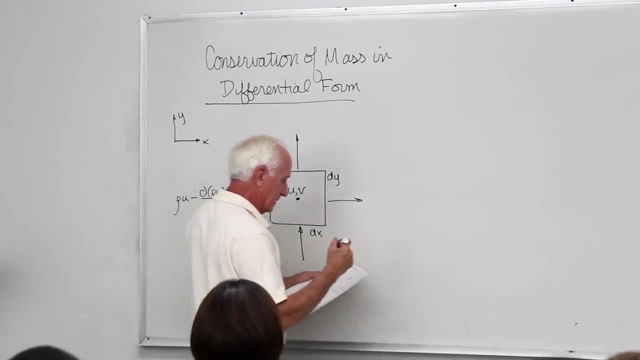 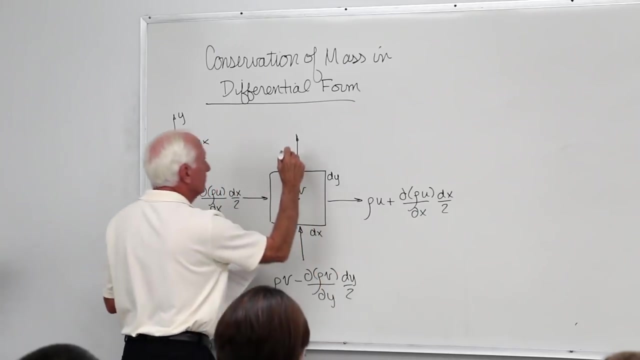 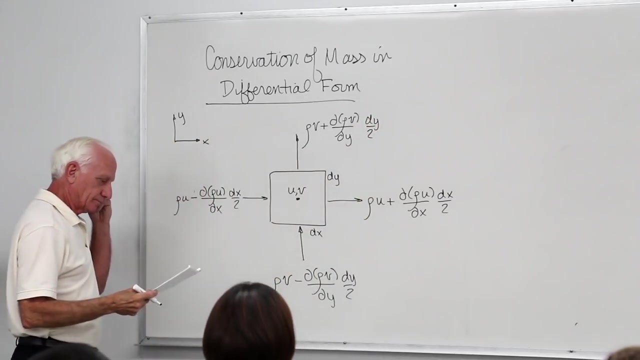 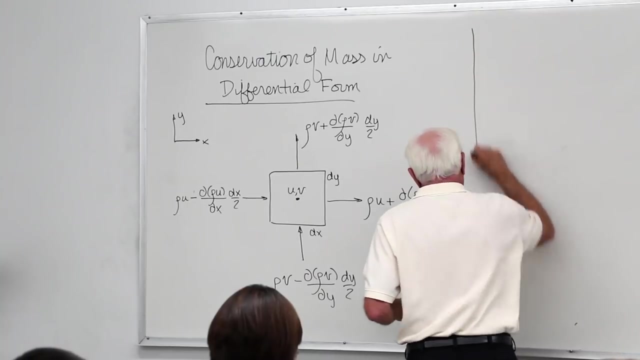 Over 2, I'll explain in just a minute, so hang on until I explain it. Rho u plus now. we went to the right, so it's plus. Now we do the bottom, You do the bottom, And then I'll just write down: conservation of mass. 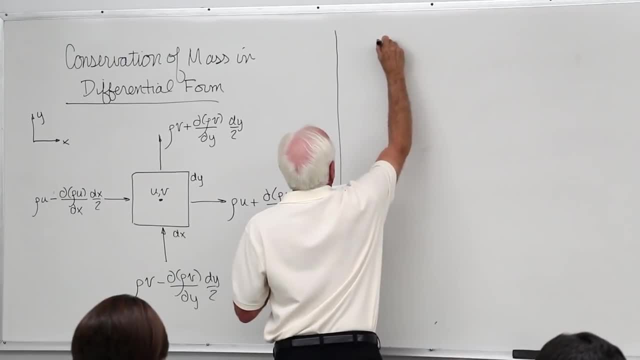 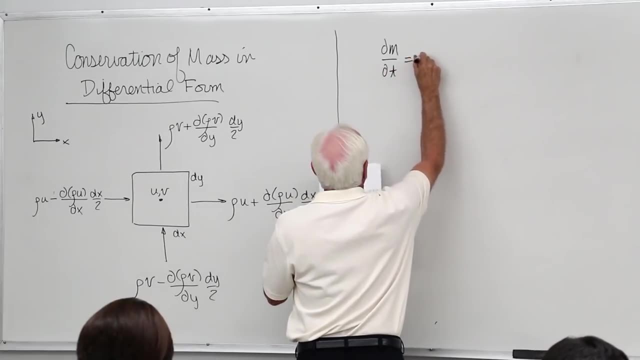 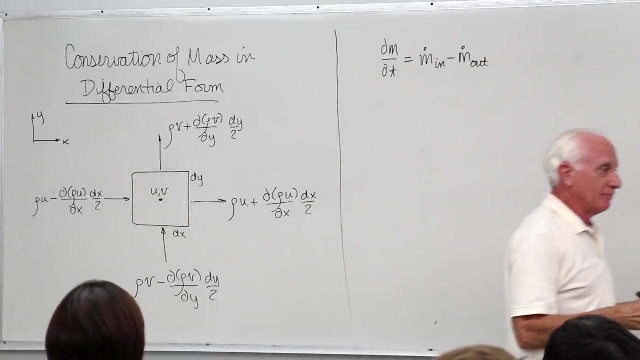 in simplistic terms, This is DMDT. What it says in words is the time rate of change of mass in that little element. 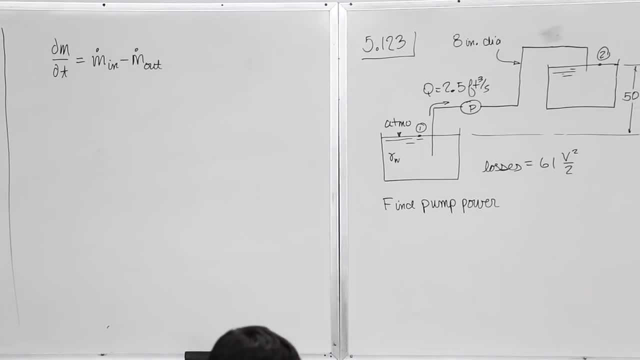 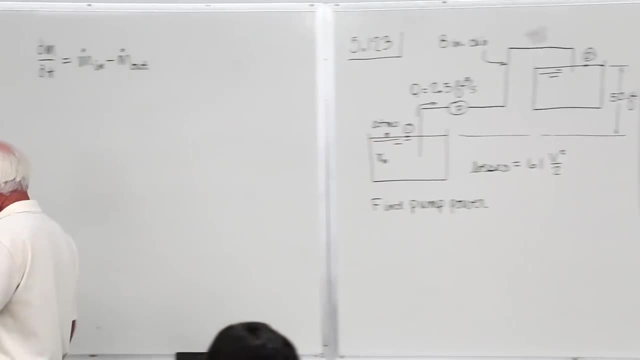 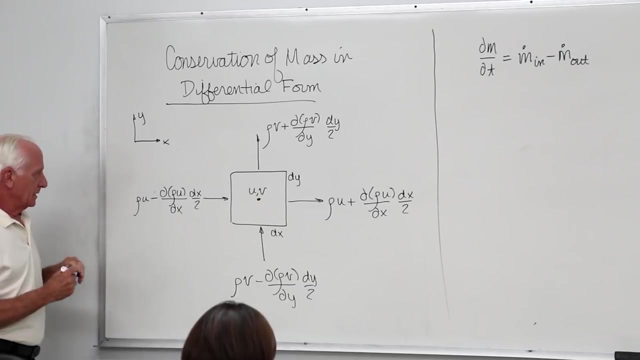 is equal to the amount of mass that came in, minus the amount of mass that went out. So what is this? rho times U. Okay, rho. what is MDOT? MDOT, rho A V. So if I multiply density times velocity, that's a big part of the MDOT. 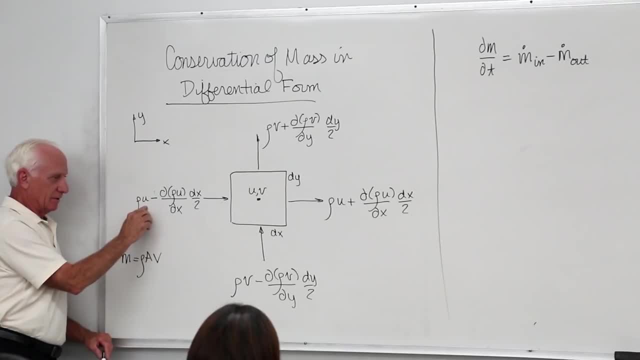 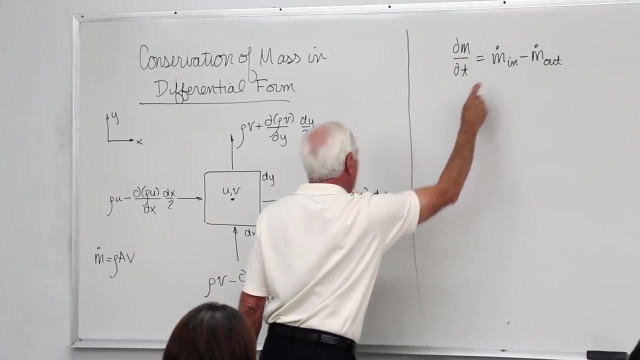 So this right here what comes in if I multiply it by the area that it comes in. this is the amount of mass that comes in in the X direction. This is the amount of mass that comes in in the Y direction. Both those terms are those two guys right there? 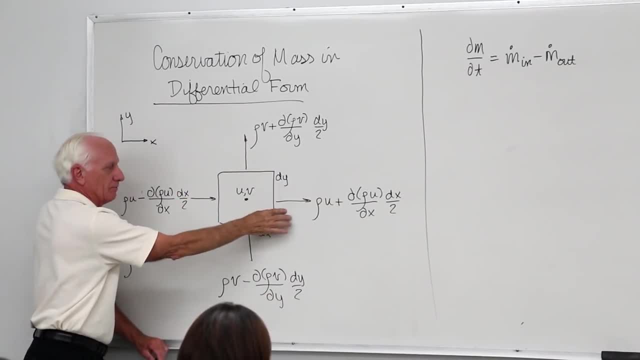 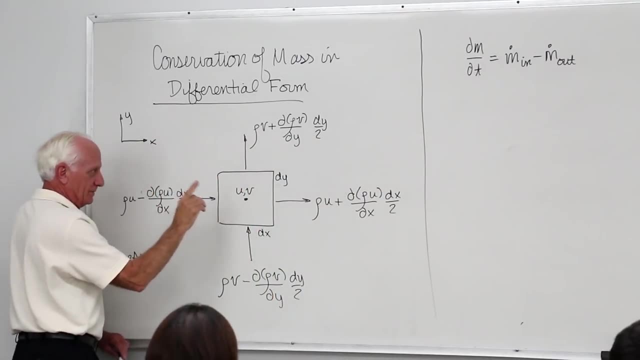 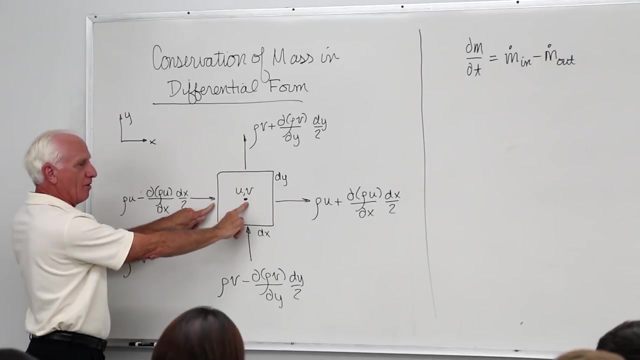 The mass that goes out out the top, out the right, Those two guys right there, these guys over here, Don't forget. now, this is the velocity U in the middle. What's the velocity U on my left fingertip? Well, how far did I go in the X direction? 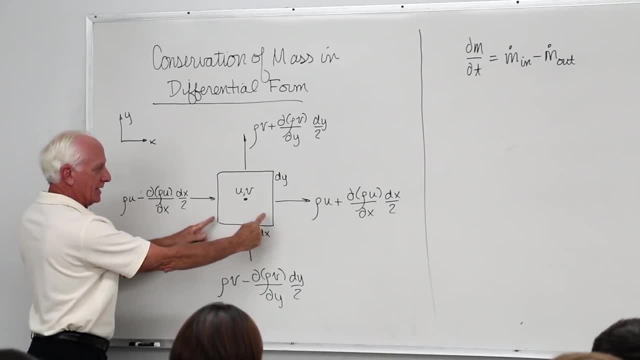 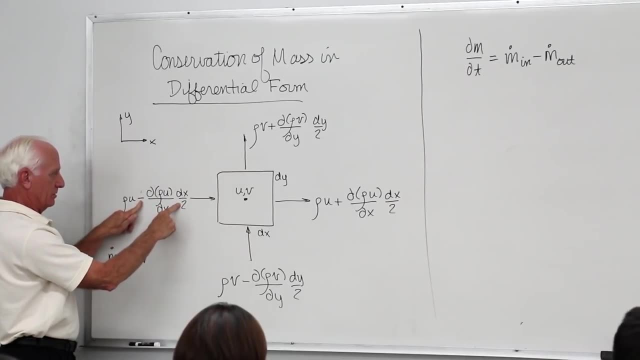 Minus DX over 2, this is DX. How far did I go over? Minus direction: DX over 2, right there, DX over 2.. So partial of rho U with respect to X, multiplied by how far I go over in the X direction. 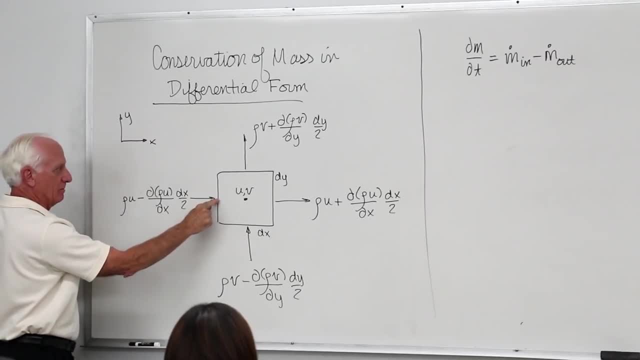 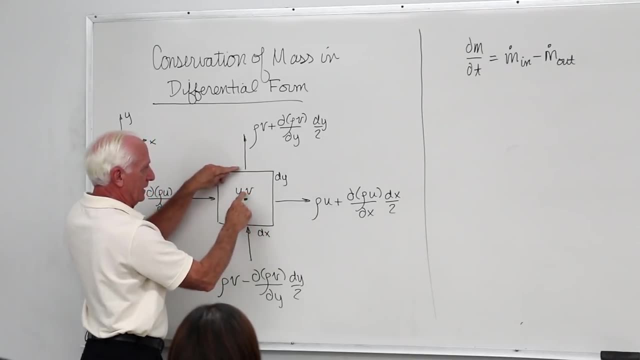 gives me the value where my fingertip is now, This gives me the value of mass flow rate where my fingertip is here, And so on and so on. This gives me this. This gives me that, This gives me this. Okay, so that's where these terms come from. 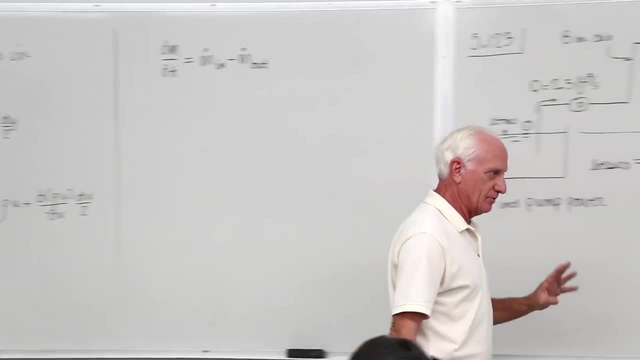 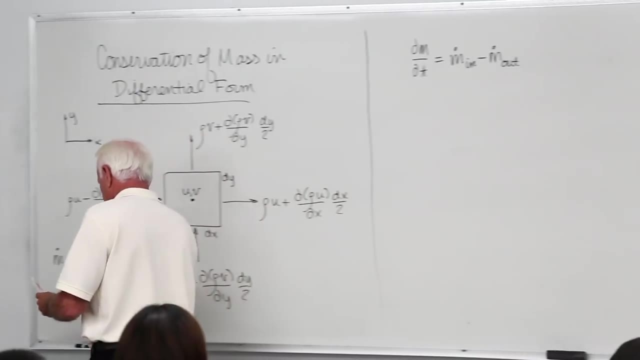 We don't know which way the mass is flowing. We do it generally. We just do it in general terms. It'll come out in the wash when we're done. Okay, so let's go ahead and plug in here now. DMDT. 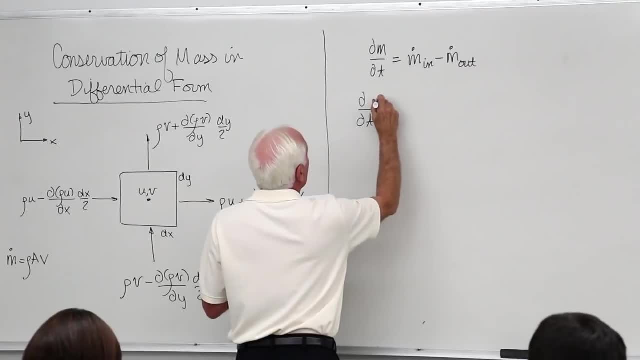 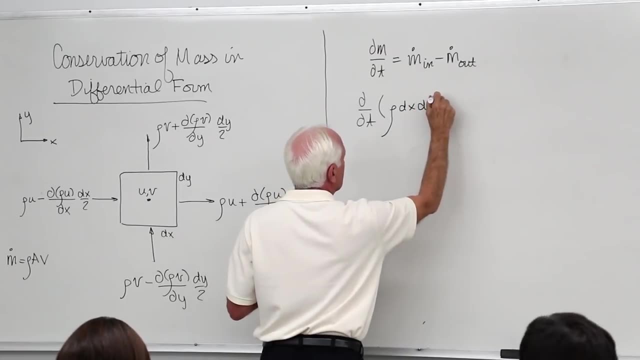 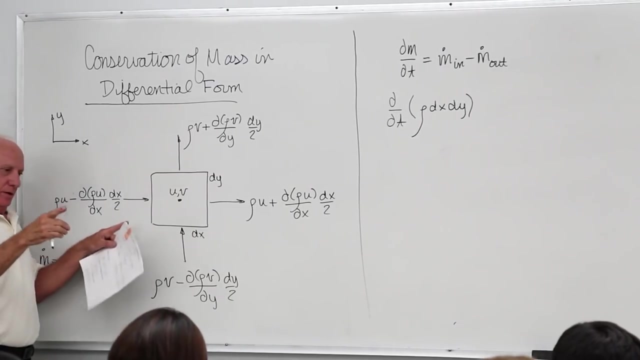 DDT. okay, the mass inside of there is rho VX VY. Now I'm going to assume, to make things simple, that it's one unit into the blackboard, One unit in here. So what's the volume? 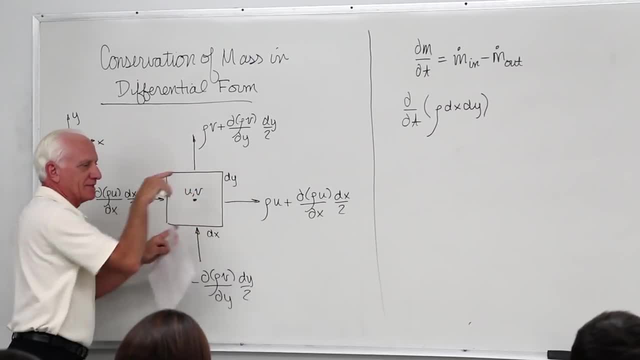 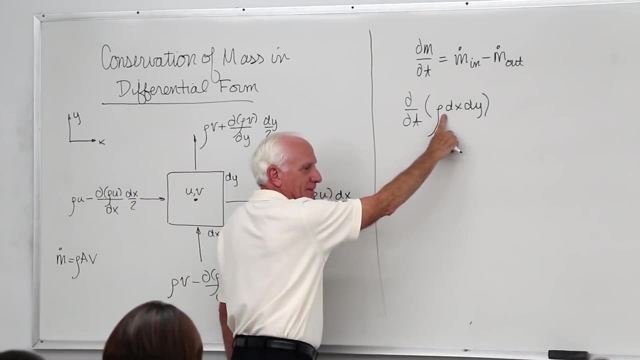 Into the blackboard. one Times DX times DY. that's the volume. One times DX DY: This is the volume. Multiply the volume by the density and what do you get? The mass. This is the rate of change of mass in that little element with respect to time. 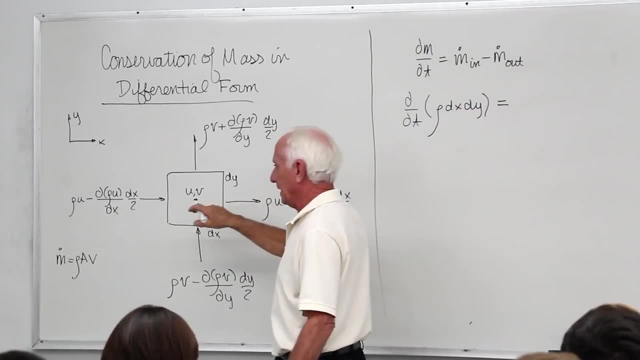 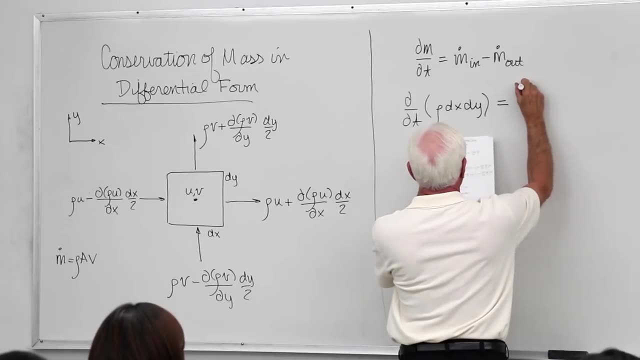 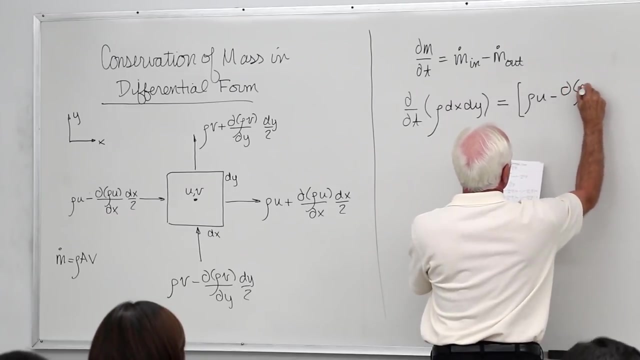 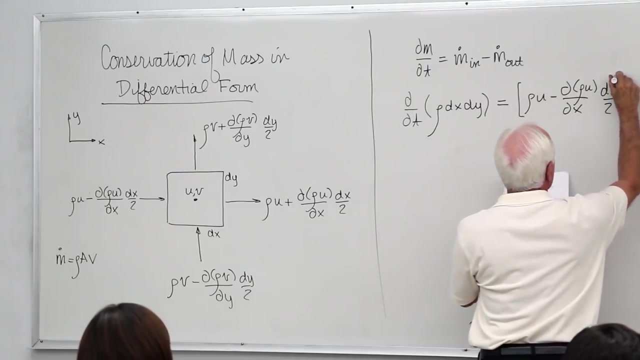 How did it change? Well, some stuff came in. Okay, here it is. That stuff came in. So here is what came in: Rho U over there, minus partial rho U with respect to X Multiply by DX over 2.. 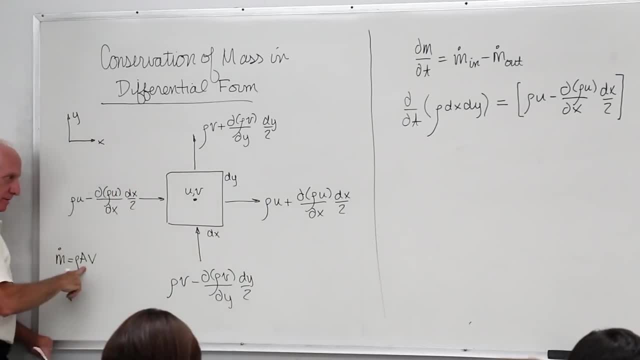 How big is that area over here? Don't forget. I need to put the area in because the mass flow rate is rho times V times A. There's rho times velocity. What's the area? DY times 1 out here. 1 times DY. 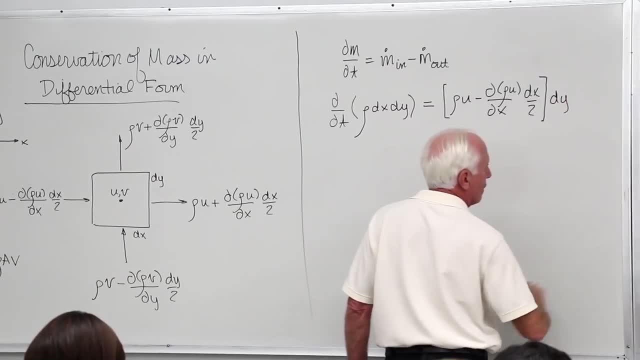 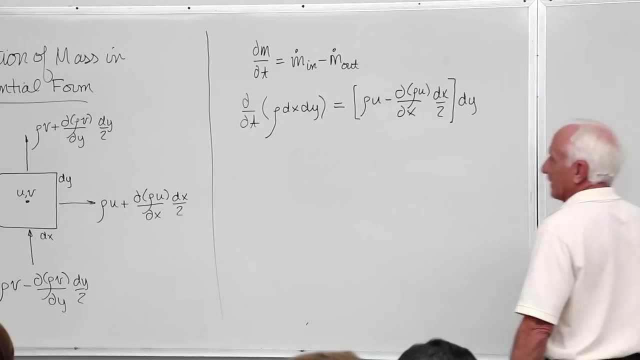 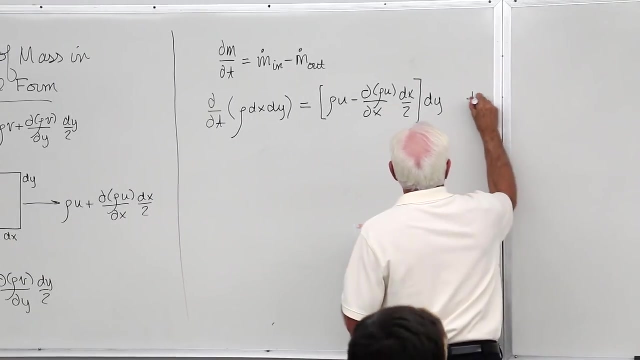 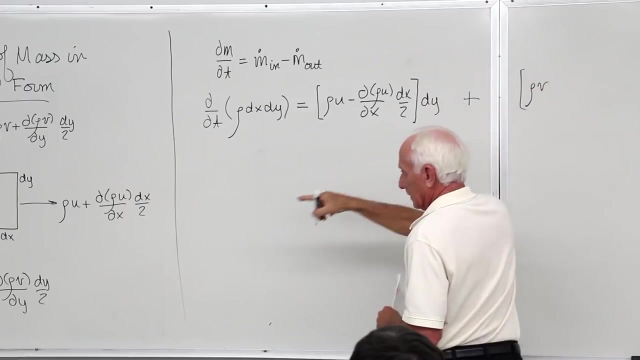 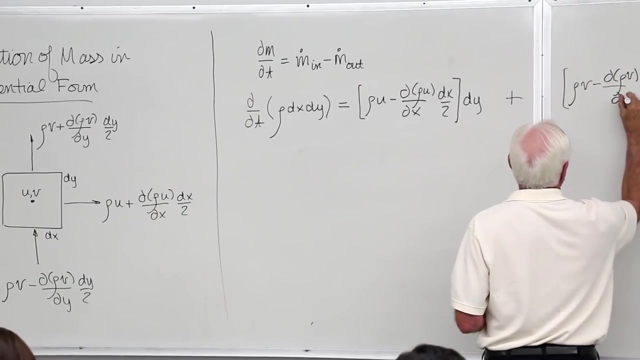 We won't show the 1 in here, so it's DY. Okay, that's one term. What else comes in Down there at the bottom? comes in Plus at the bottom: rho V minus partial rho V with respect to Y times: DY over 2.. 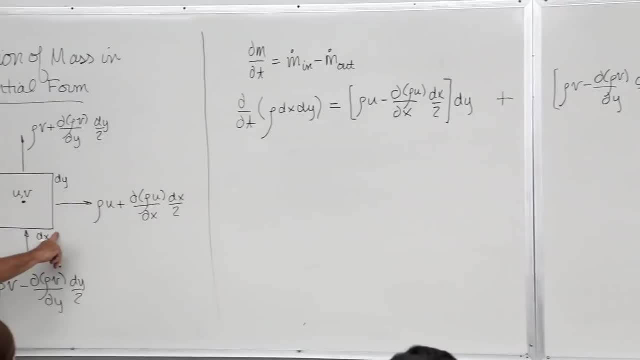 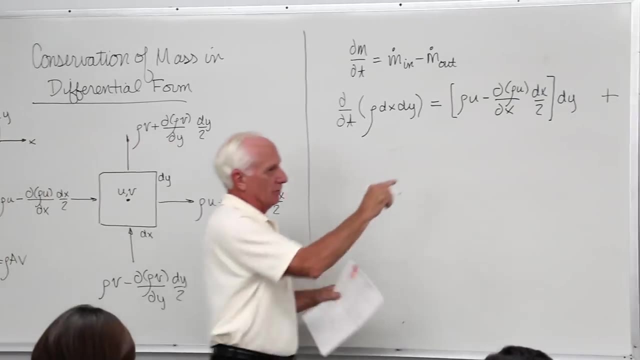 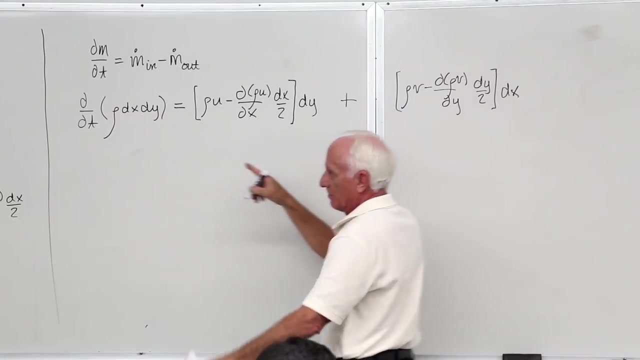 Okay, what's the area that that comes in from my fingertips? DX times what? 1. From the blackboard: DX times 1. So multiply this guy by DX. These two terms are the mass that comes in Now the mass that goes out. 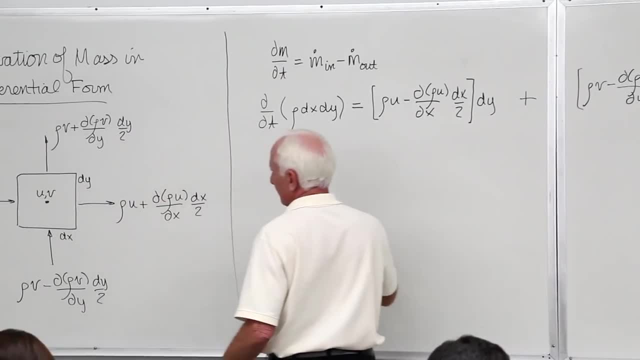 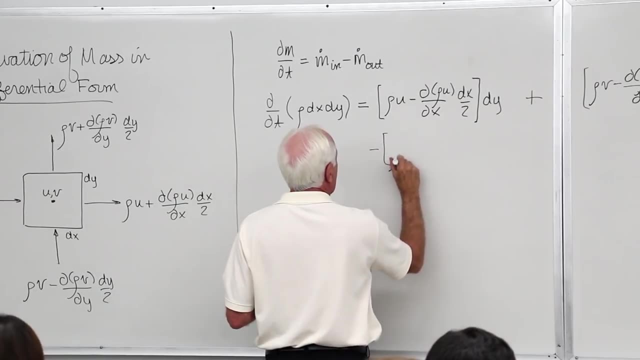 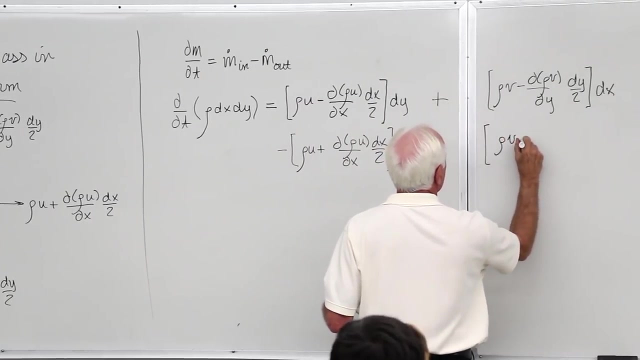 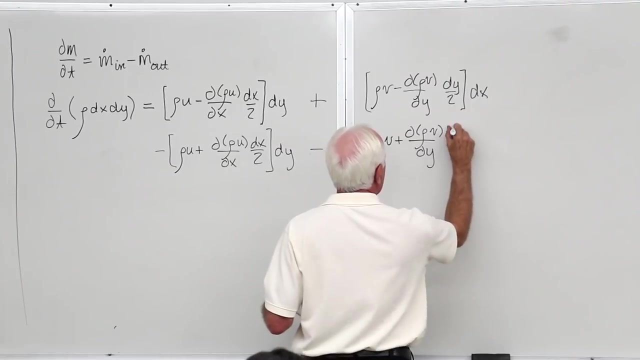 This one and this one. So when it goes out minus, sign right here, Minus the mass that goes out Rho U Partial rho U Same area. That's yeah, minus here too, Minus rho v. 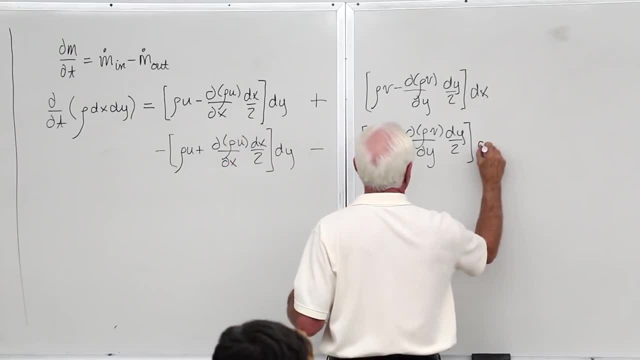 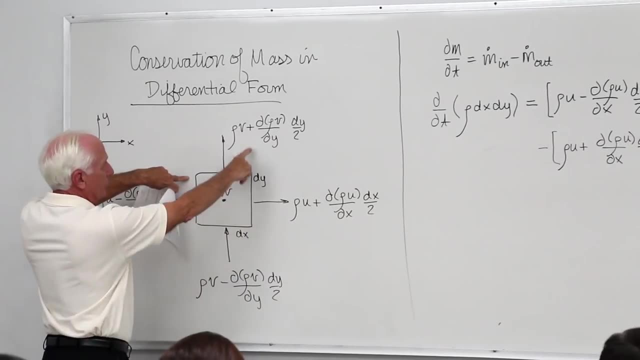 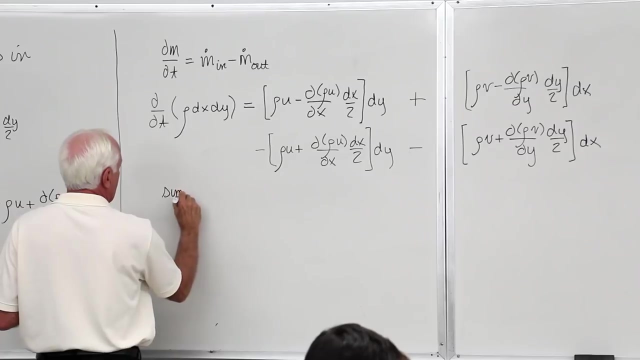 That area. that's y, that's x, That's this one up here, Plus sign, plus sign. Okay, simplify these guys right here, I'll tell you one right here. Here's a rho u, here's a minus rho u. 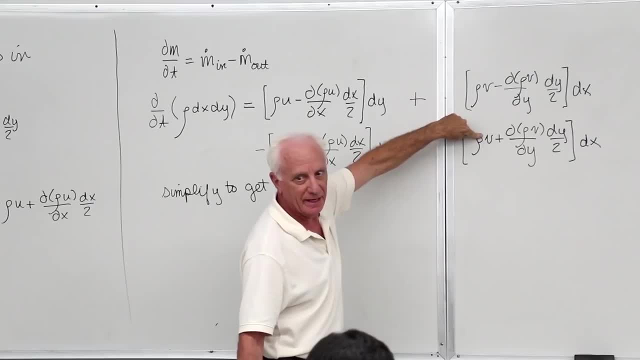 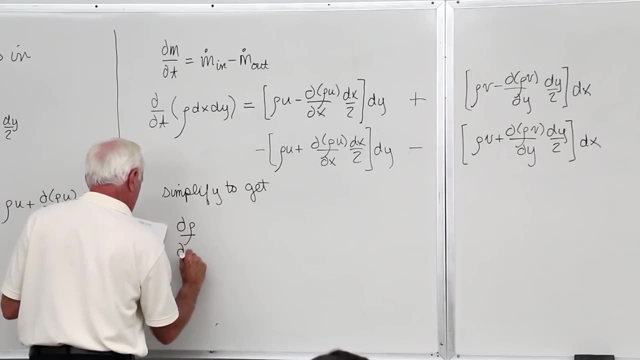 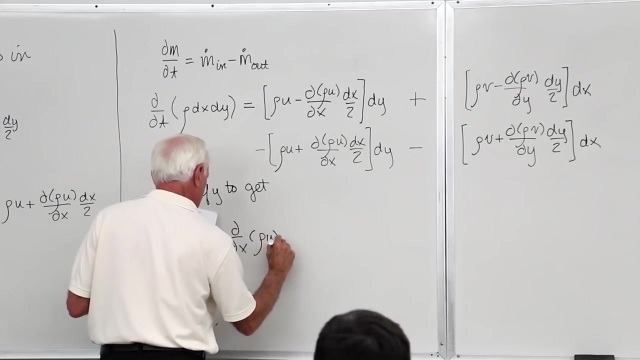 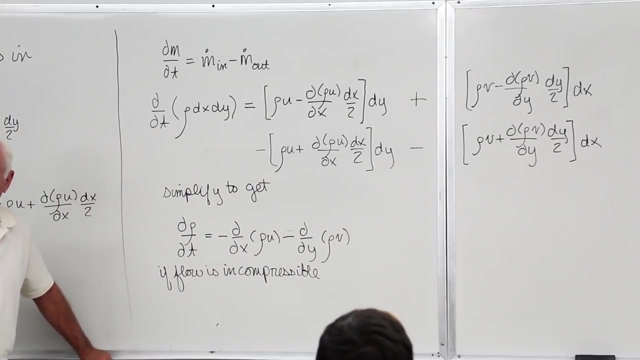 Here's a plus rho v, there's a minus rho v. Cancel them out. So you simplify it. to get this Now we can further simplify that if we say that the flow is incompressible, Density is a constant, Pull the density outside the partial sign and then divide. 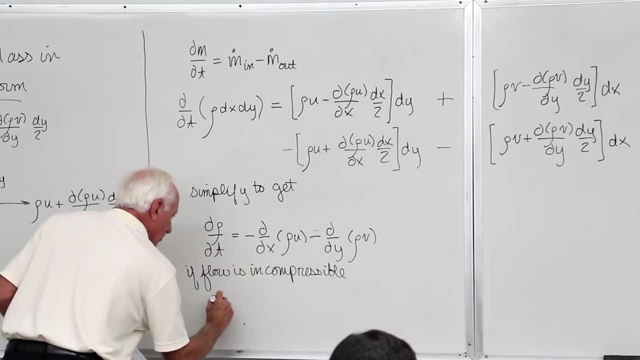 through this. It's not changing with time. so zero over here. First of all, make that guy zero. Now pull rho outside and divide through by 0.. Okay, And divide through by rho, Multiply through by minus 1, and you end up with. 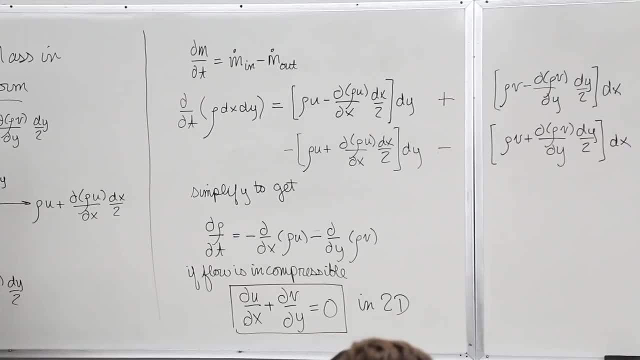 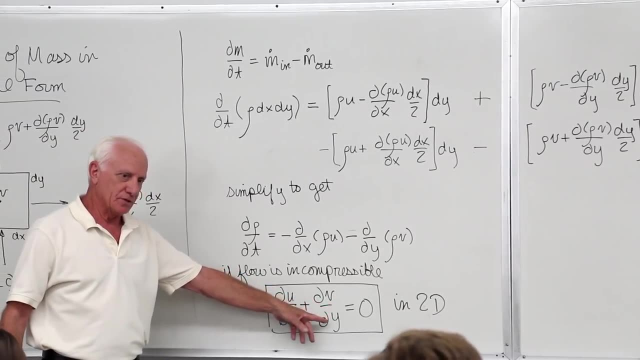 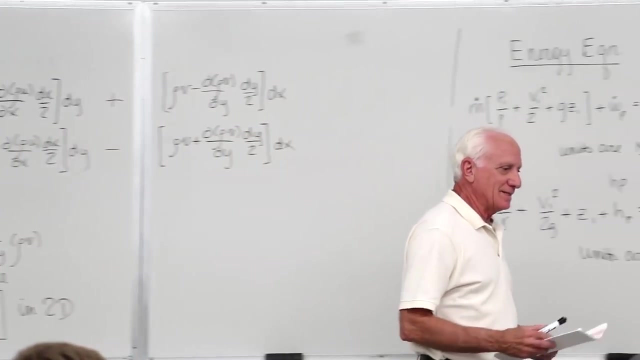 The conservation of mass written in two-dimensional terms. If you've got a 3-D case, you just add one more term, partial w with respect to z. What does that mean? That means at any point in the flow field, in an incompressible. 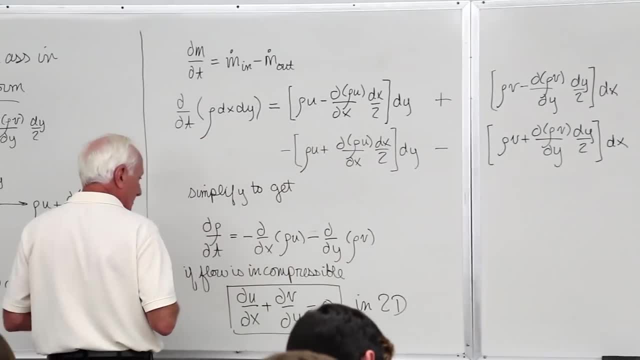 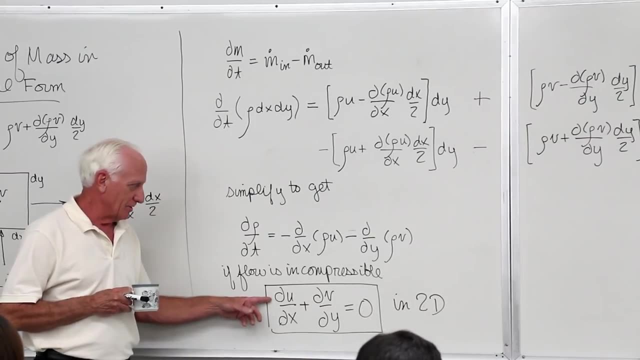 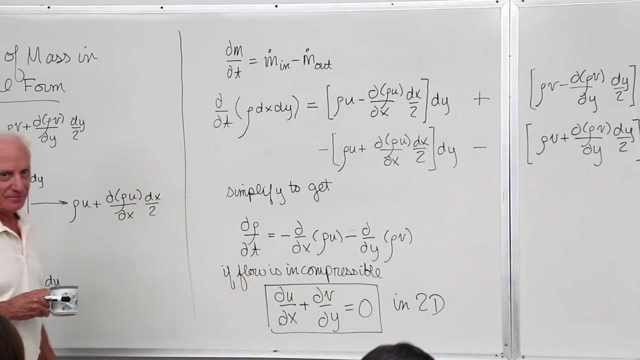 flow field at any point in the flow field for an incompressible fluid under steady state conditions. this thing must be satisfied. When you take the partial of u with respect to x and add it to the partial of v with respect to y, you better get zero or you haven't satisfied. conservation of mass. 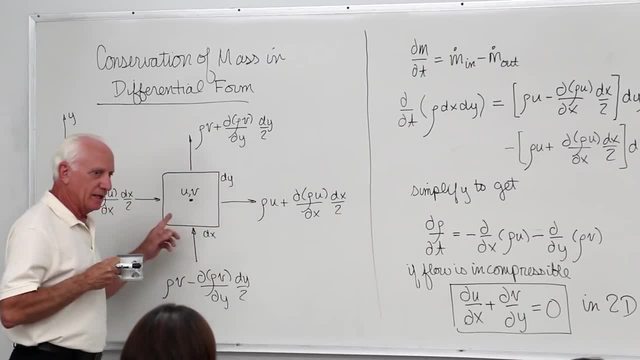 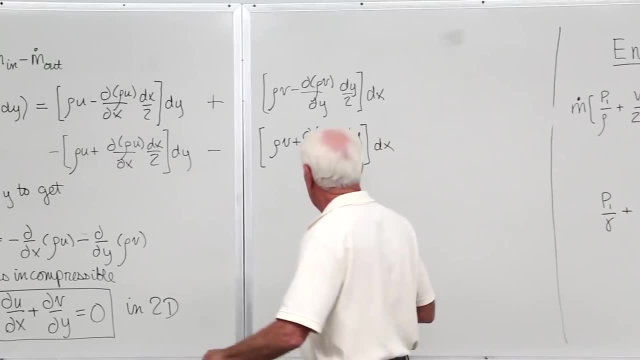 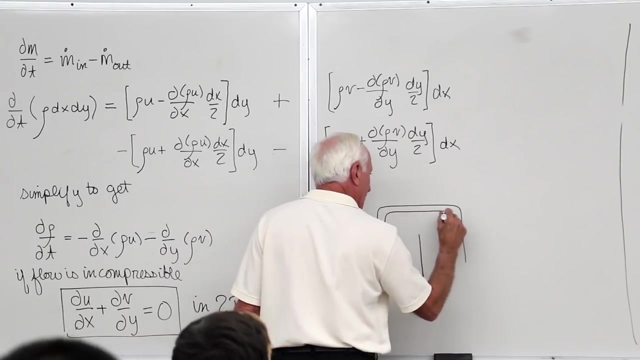 Where does this apply? At every point in the flow field. At every point in the flow field, it has to be satisfied. So if we had that Picture like this, and then there's something like this, and so on and so forth. 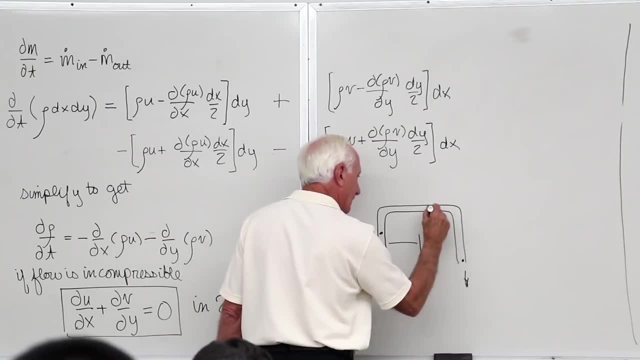 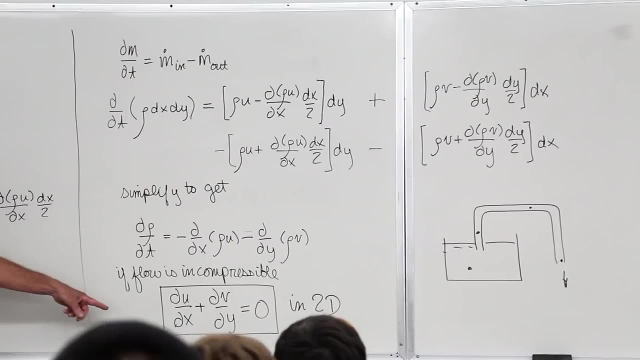 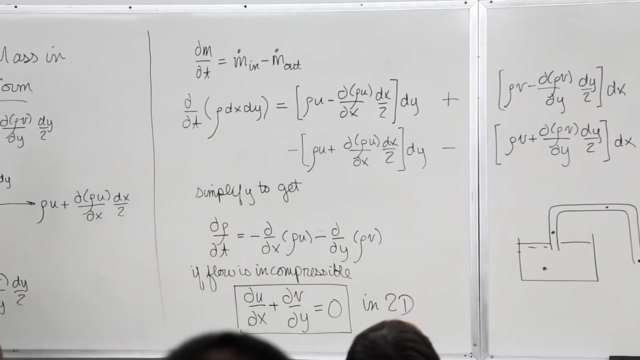 I don't care where that point is in the flow field. At every one of those points in the flow field that thing's got to be satisfied If it's steady state and incompressible Any point in the flow field. What's the difference in this guy and the one that we had in chapter? 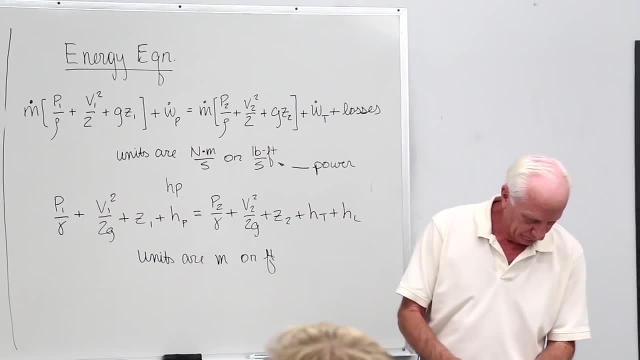 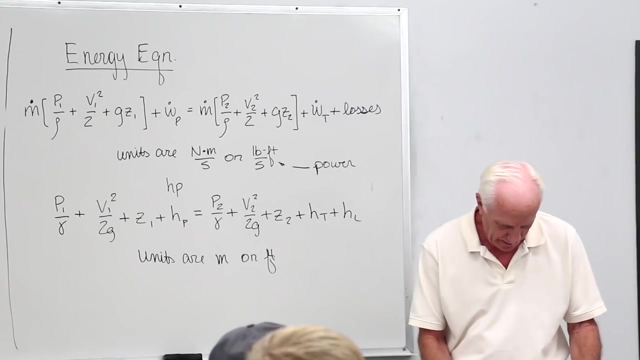 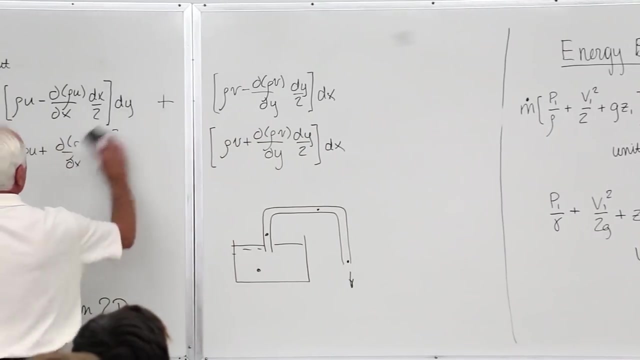 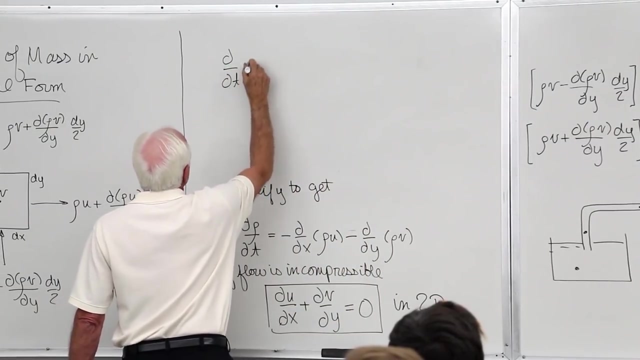 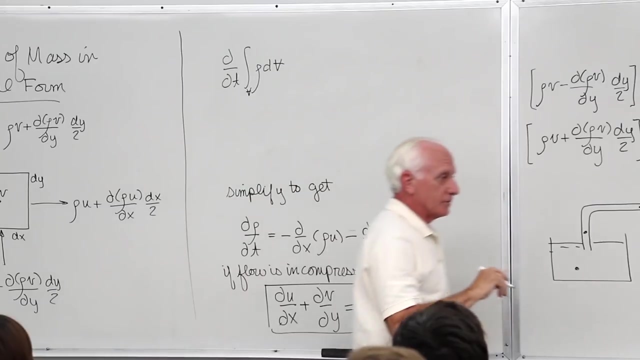 Five, Five. Let's go back to chapter five. Let's go to the first part of five. Here it is conservation of mass for our continental plane. We have fixed control volume. Oh, I'll just write it down Partial with respect to t rho dv. That was our first term and the second 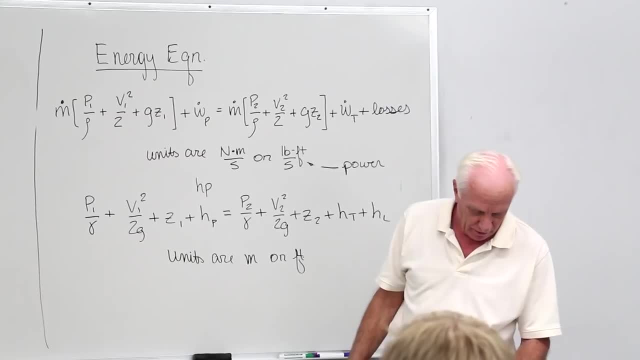 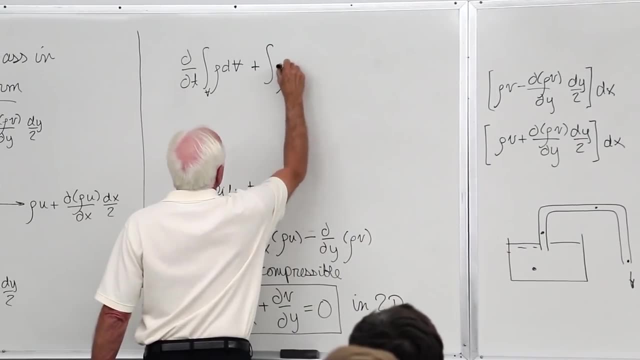 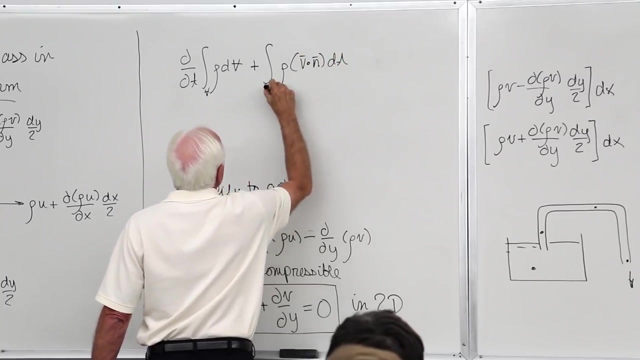 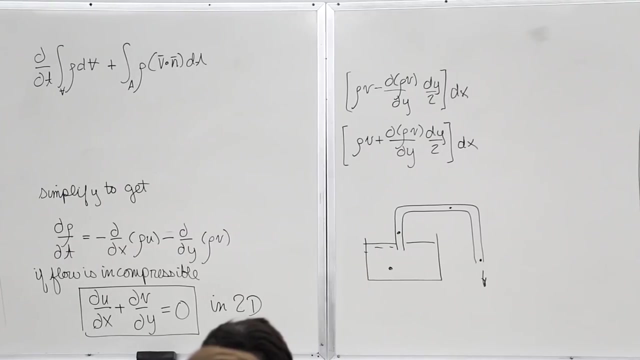 one was the convective terms, which were our rho rho v dot n and rho v dot v dot n d a. I think that was pretty much. Yeah. that was it for our conservation of mass, and that was zero. 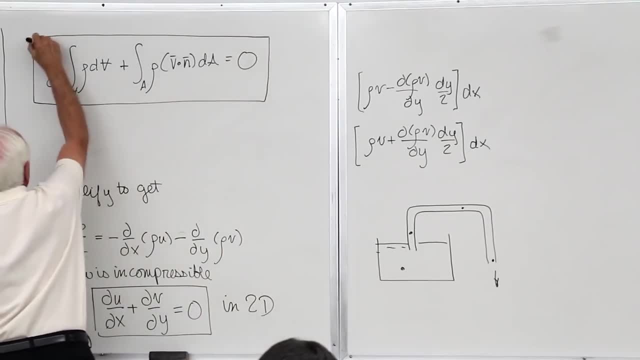 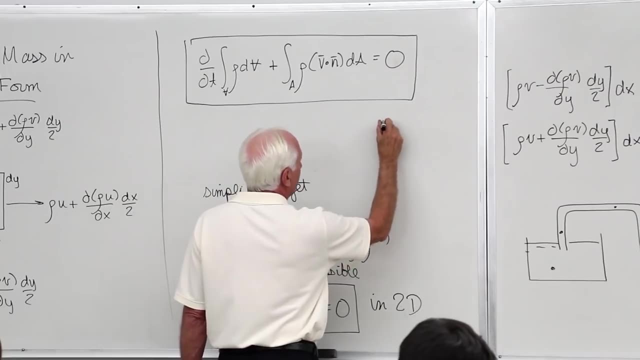 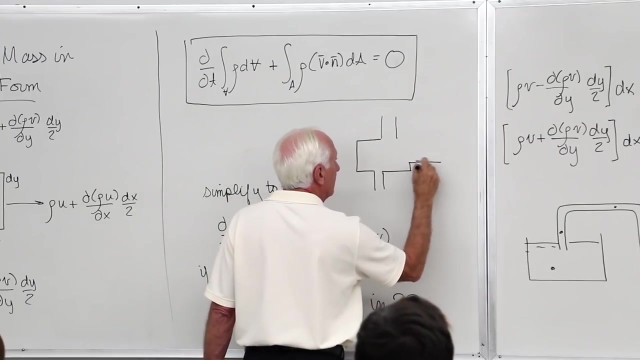 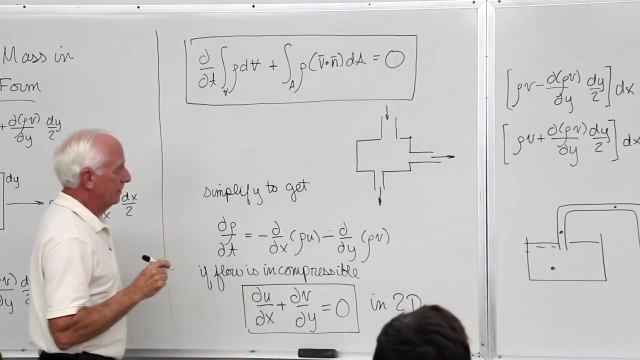 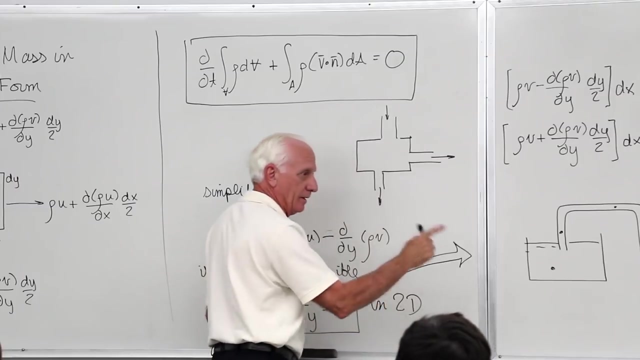 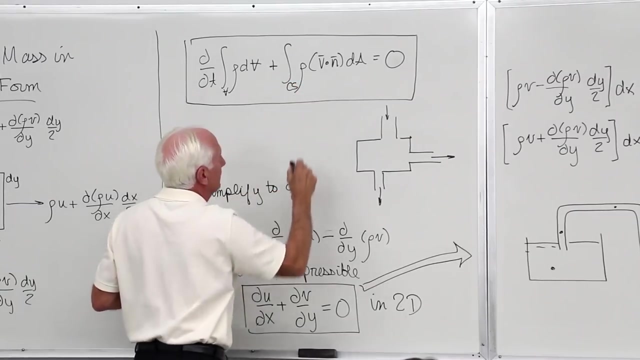 So, So, in this guy up here, if we had some fluid coming in here and going out here. This guy here, we apply at any point in the flow field: This guy here, This guy here. the first step you're doing in chapter five here with this equation: 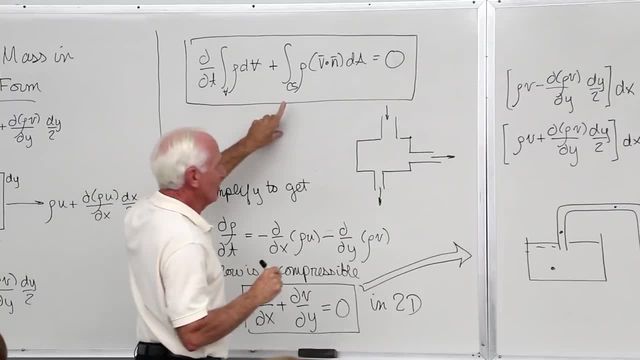 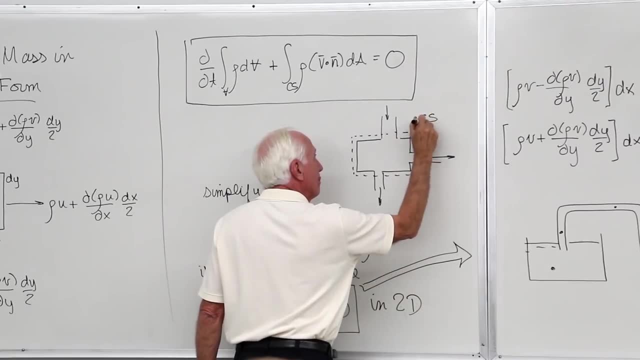 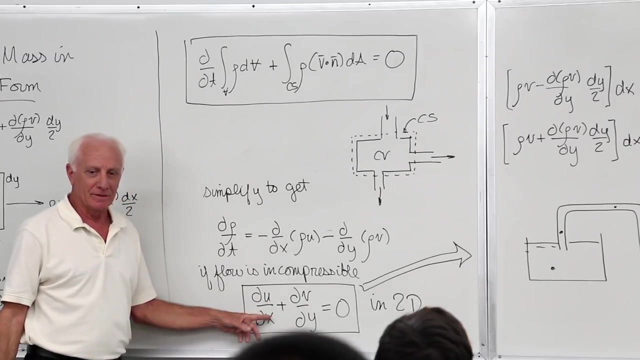 is: show me the control volume, Show me the control surface. Okay, I will. Okay, Over here I'm not talking about control volume and control surface. Over here I'm talking about a point in space and applying the conservation of mass to a very small point. 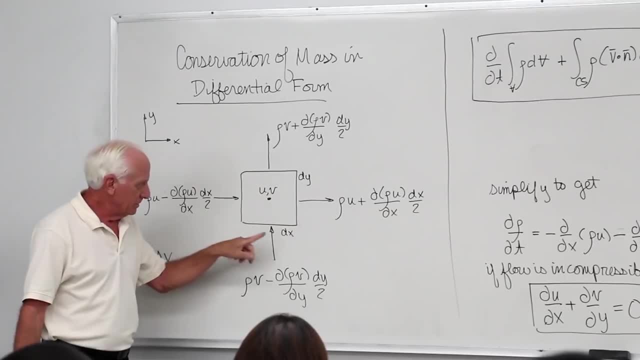 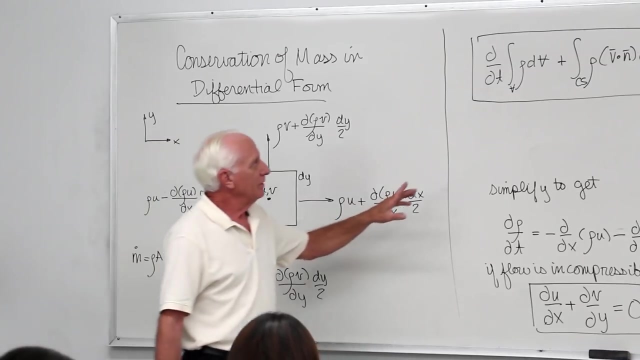 in space. This little. It's called a differential element: dx by dy- How big is it? dx by dy: How big is dx and dy? Oh, they're small, They're real small. That's calculus In the limit, you know. they go to zero. Yeah, So this guy, chapter five, you apply to that. 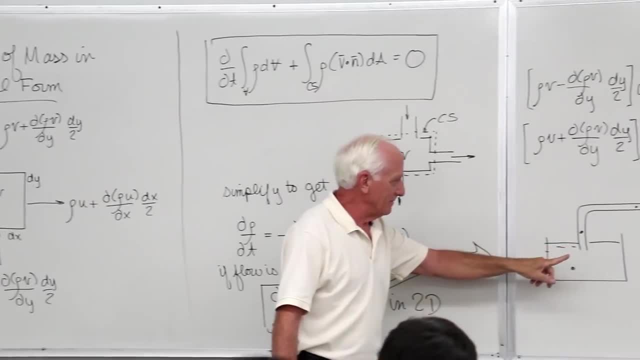 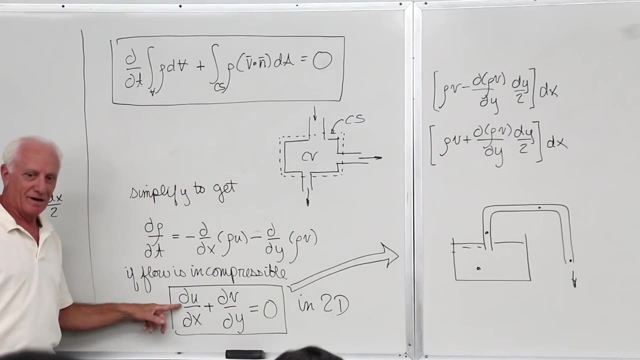 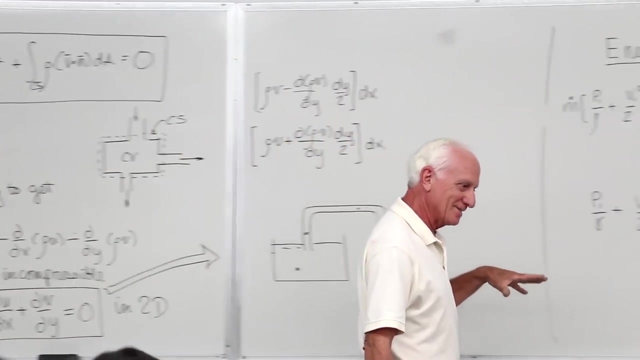 picture. If somebody says is conservation of mass satisfied right there at x equals three, y equals four, Try this guy right here and you can say yes or no. Yes it is, No, it's not. So they're different things, They're both. conservation of mass, One's applied to. 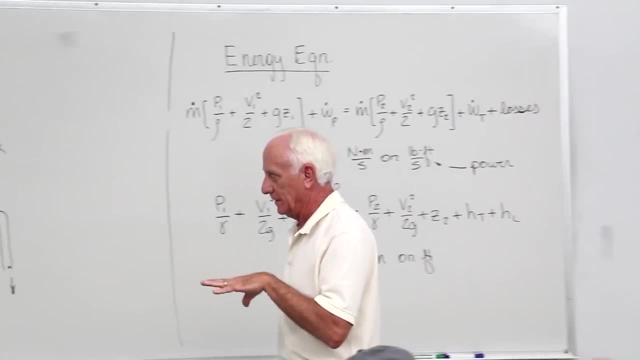 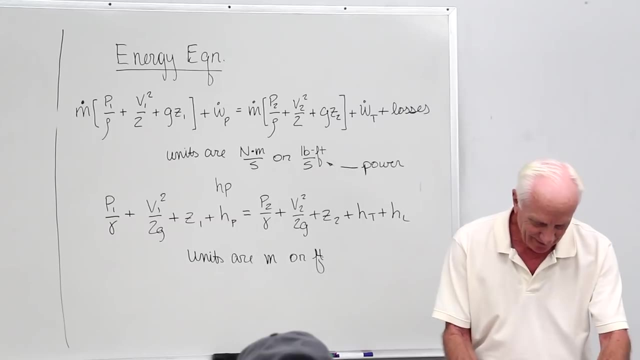 a control volume. The other one's applied to a point in a flow field. Okay, So let's take a look with that. then Let's look at problem 6-12.. For homework you have Okay, 6-12.. That's homework. 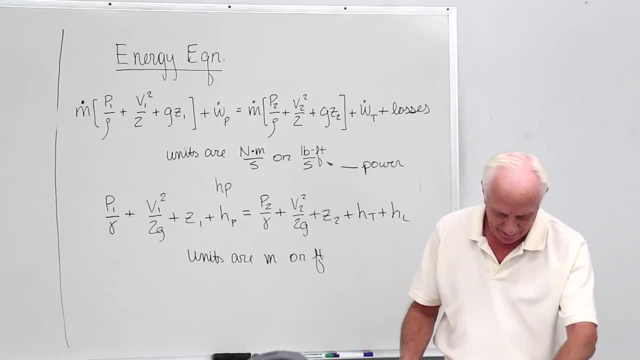 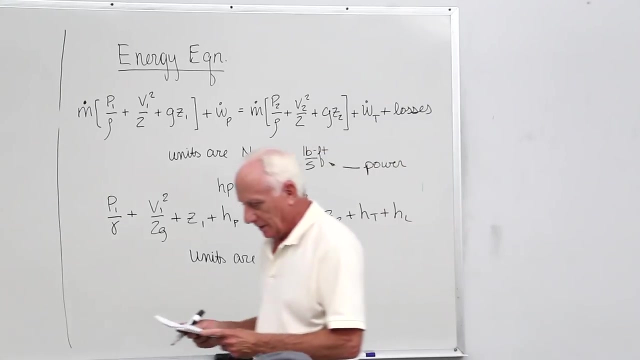 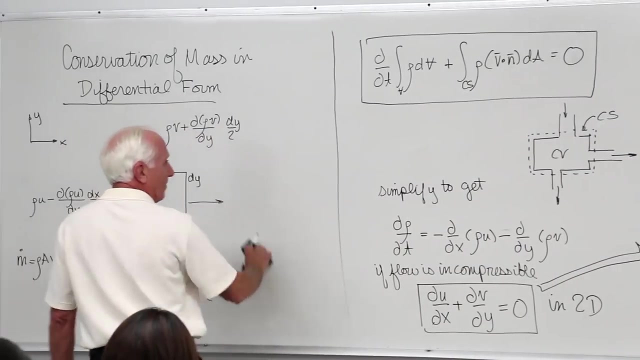 Maybe we lost kind of a simplistic one. Let's see 6-12.. Yeah, We'll do I think. yeah, Let's just go ahead and do 6-12.. I'll do that one. Okay, Let's see In the room. I'll put that over here. 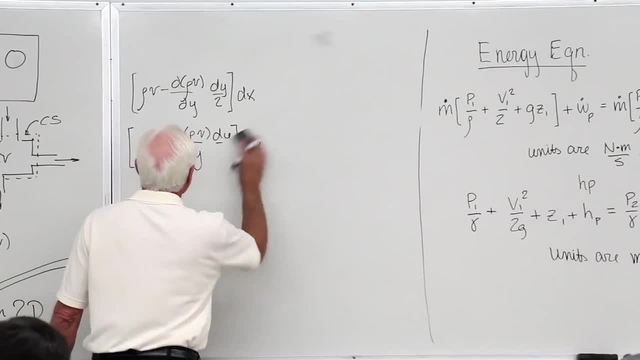 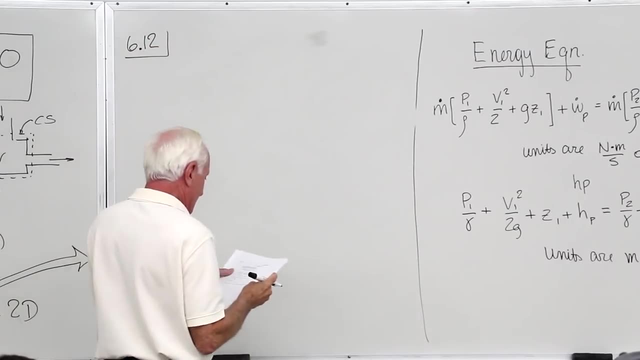 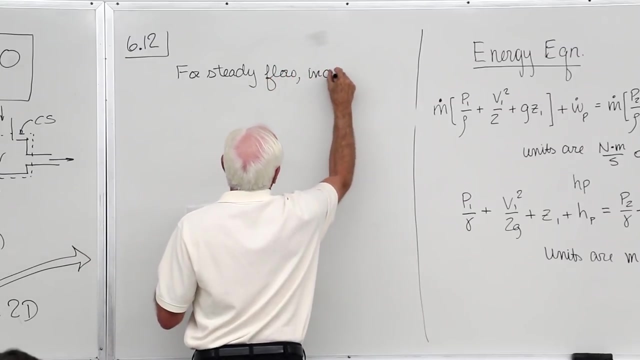 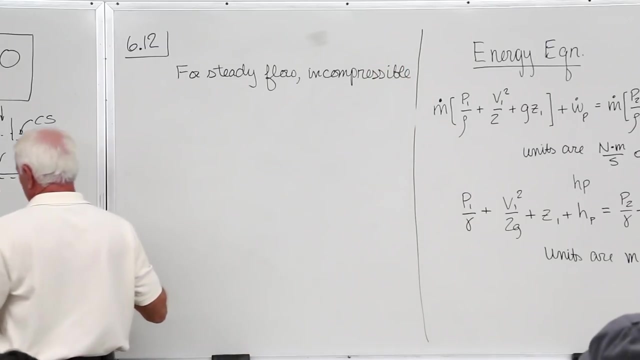 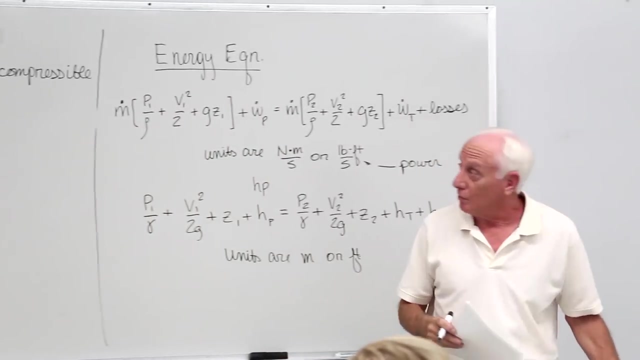 No, I'll put that over here. Okay, So for a certain incompressible, steady flow, Incompressible. We have u equal 2xy, given b equal minus x squared y. Let me go to 6-12.. Okay. 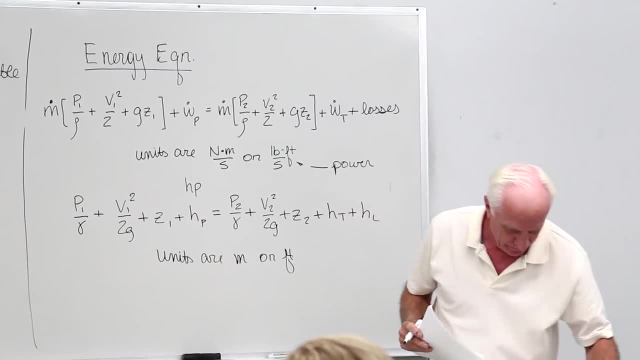 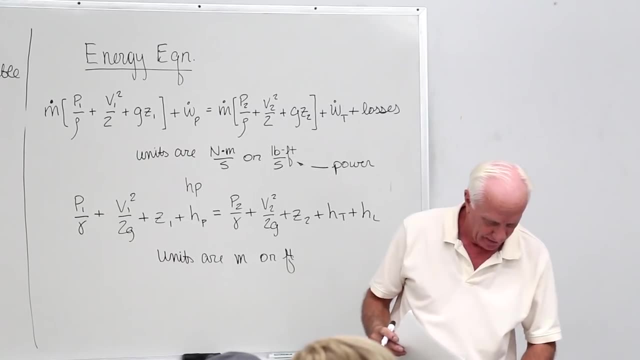 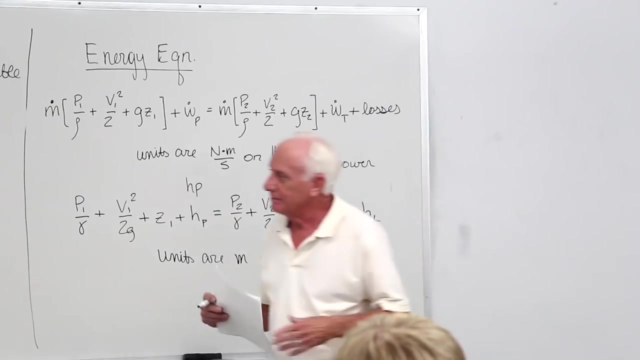 I'm going to look at that and make sure what I've got on there is what I think: 6-12.. Okay, Yeah, He gives us both of those. He puts w equal. I'll put it on there anyway. w is 0. 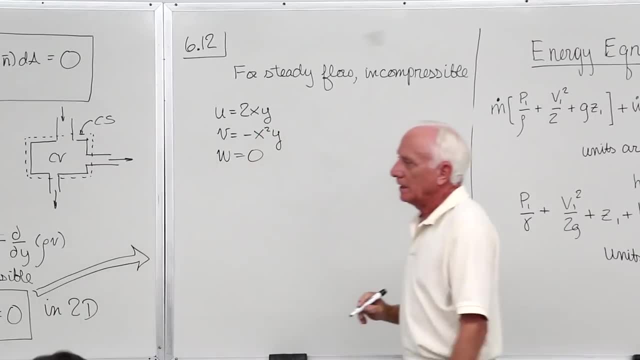 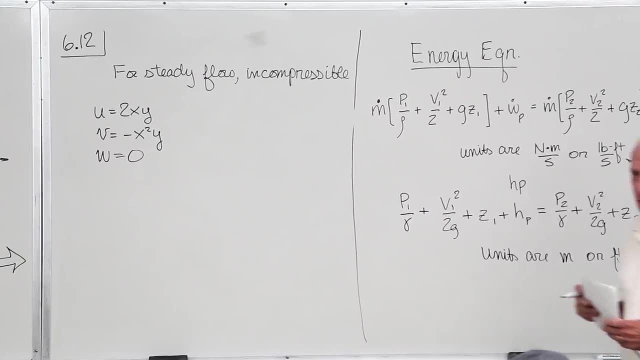 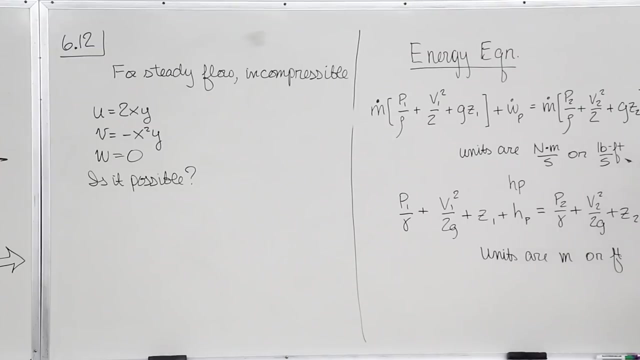 We don't need to. It's a 2D flow field. Okay Question: Is it physically possible? Well, of course we have to check. The first thing we're going to do is check conservation of mass. If that's no goal, it is not physically possible. 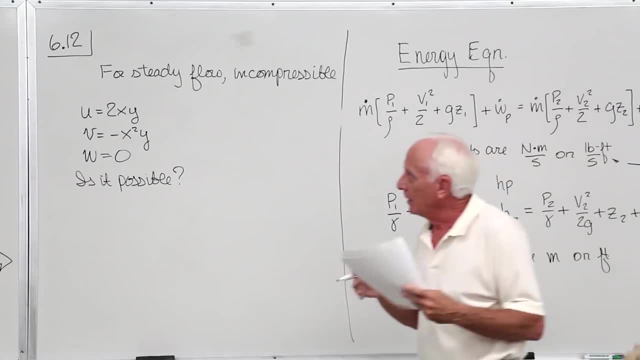 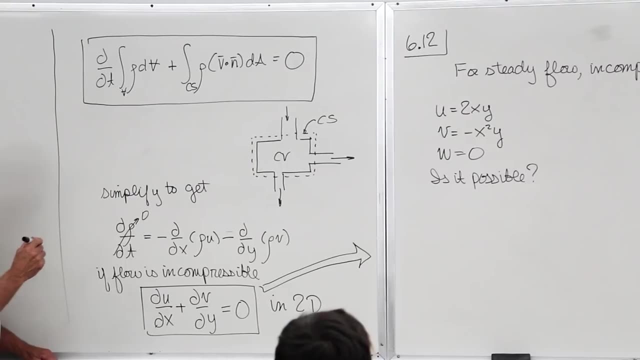 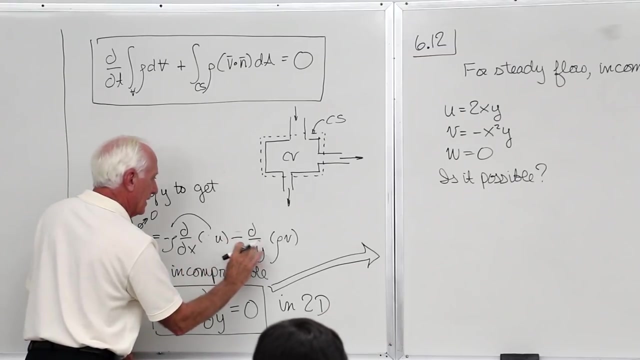 Okay, First of all, step one: It is a steady state. Yeah, He goes to 0.. Step two: Is it incompressible? Yeah, Pull the row outside. Pull the row outside. Now divide through by row. 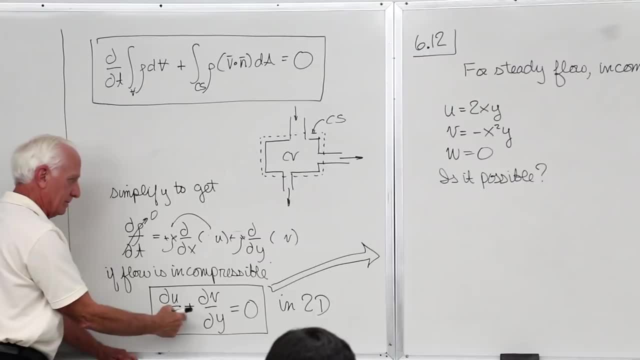 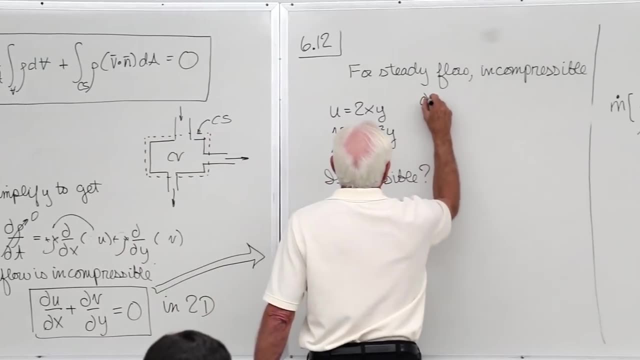 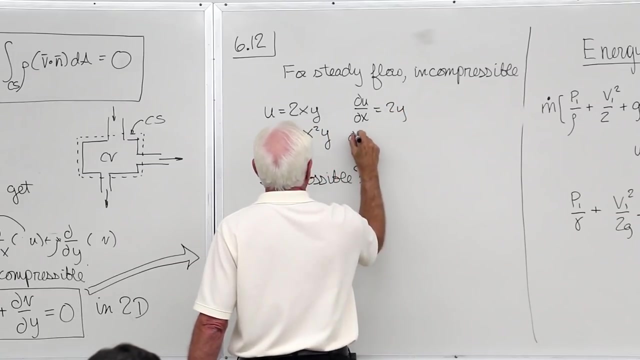 Multiply through by minus 1.. Plus plus. There it is Done. Okay, That's it. Partial u with respect to x, Partial b with respect to y. Question then: Is partial u with respect to x plus partial b with respect to y equal to 0?? 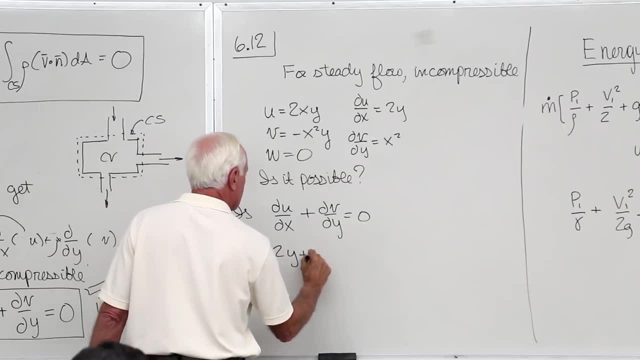 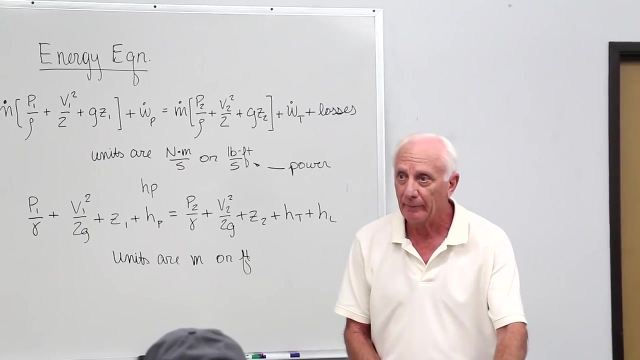 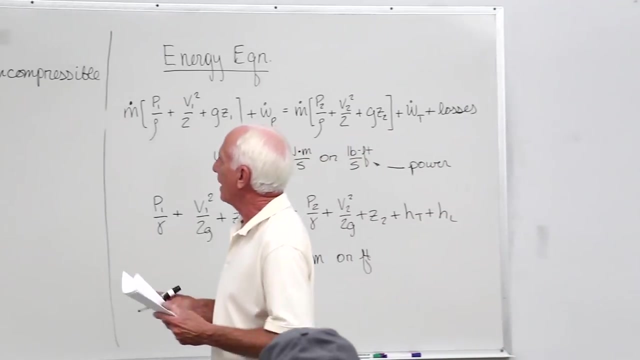 The answer is 2y plus x squared, equal to 0.. No, No, It's not physically possible. Yeah, Shouldn't bb and dy be negative? x squared Which one? Oh, I didn't see that in my assignment. Thanks, Yeah, Thank you. 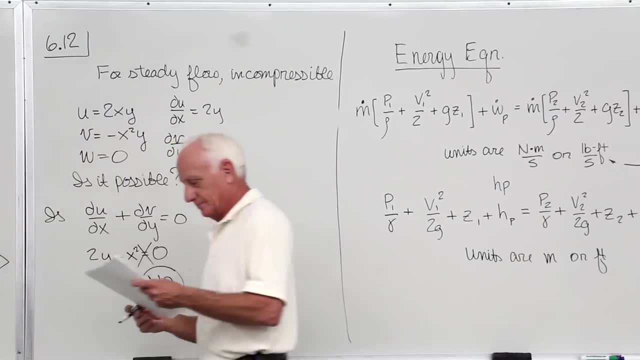 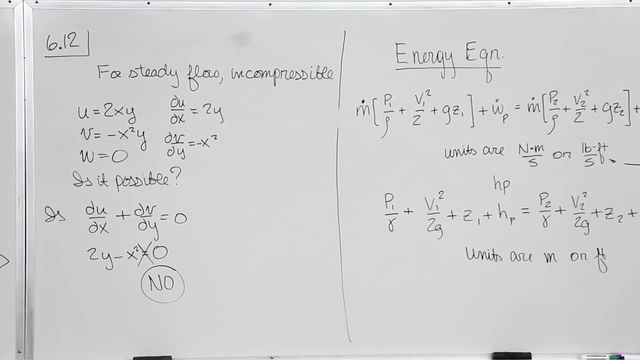 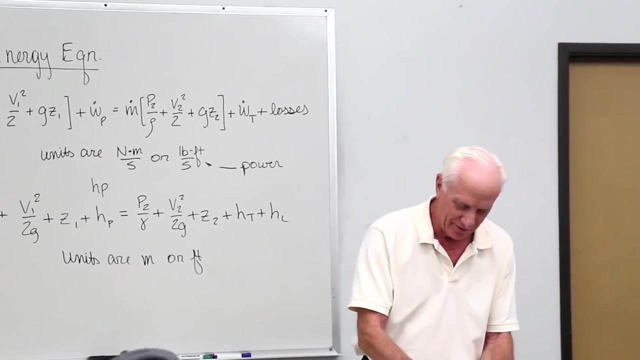 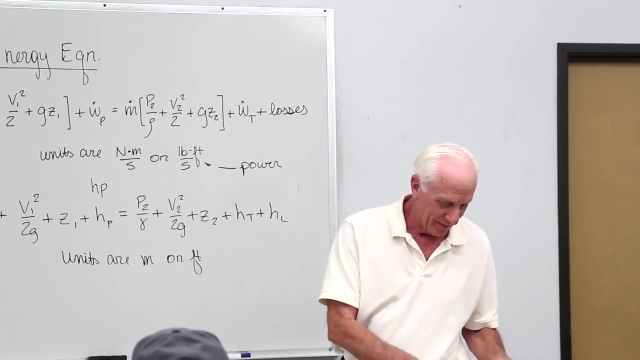 Where is the x squared? Thanks, Thanks, Okay. So that answers that question. It's pretty straightforward. It can be more difficult, of course It can be more difficult, But in our textbook, in the first Lewis course, it's pretty straightforward. 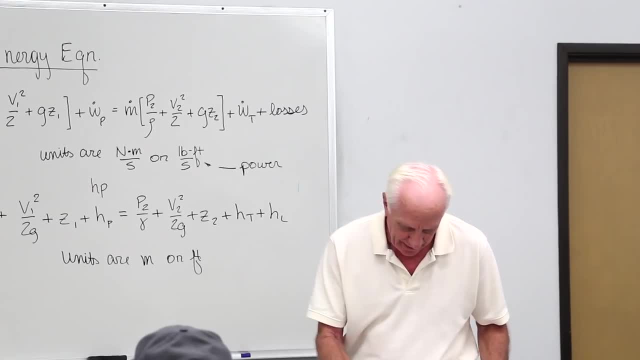 Okay, Now, I think that is all I have on that right now, And I think that energy equation, yeah, Okay, That's all I have on that. So let me just talk a little bit about the exam coming up so you can get prepared for it next week. 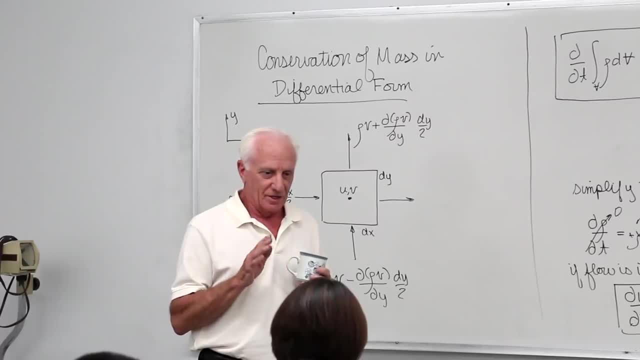 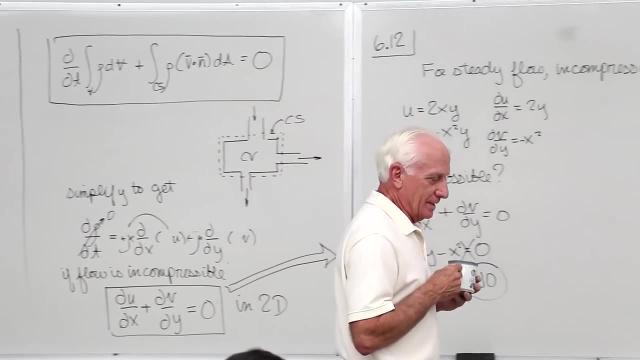 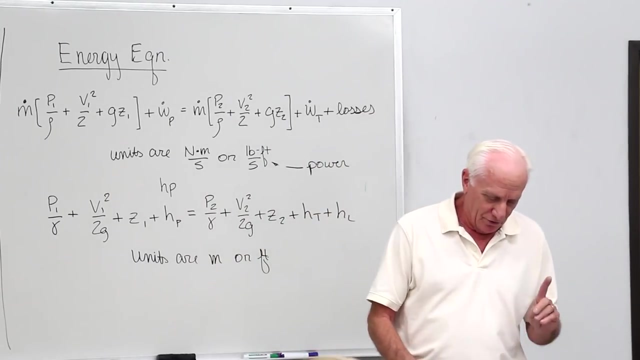 It's going to cover. as I said before, let's recall the first exam. The first exam was chapter 1 and chapter 2.. That was it So. the second exam starts with chapter 3.. Two main things in chapter 3.. 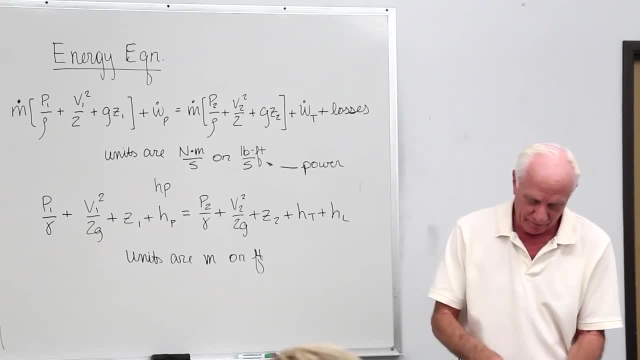 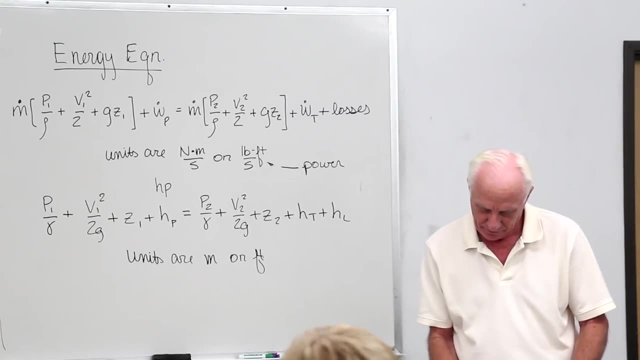 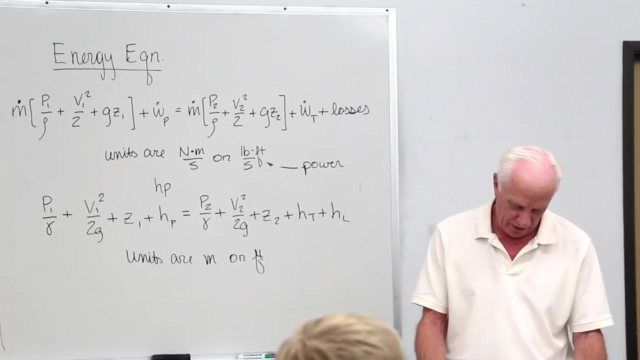 Let's just move real quick and see what those two main things are. Number one: we had F equal ma along a streamline and normal to a streamline Along a streamline. F equal ma led us to Bernoulli equation. We also have F equal ma normal to a streamline. 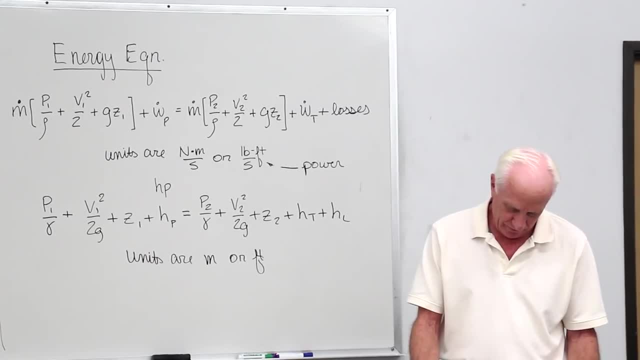 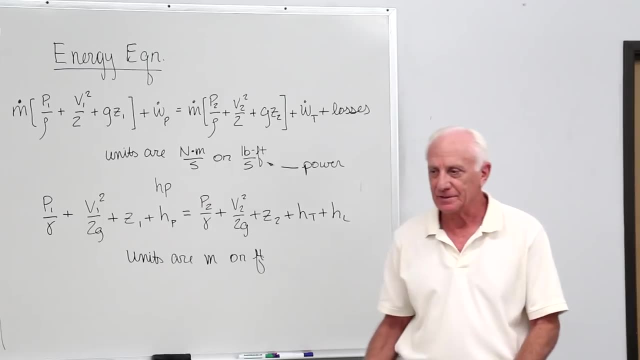 So those two equations, Or equations 3-7 and 3-12.. Okay, 3-7 and 3-12.. The second part of chapter 3, those two things. It talks about what kinds of pressure there are in a problem. 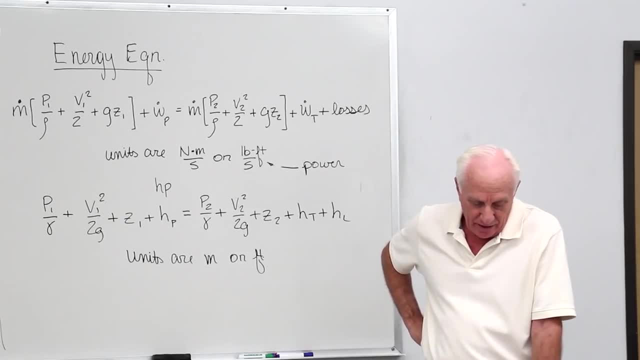 And we have it on the board: Static, dynamic, stagnation And total pressure. It's all defined in your notes, in the book too, And the rest of that chapter are examples of Bernoulli's Thirteen examples. Thirteen examples. 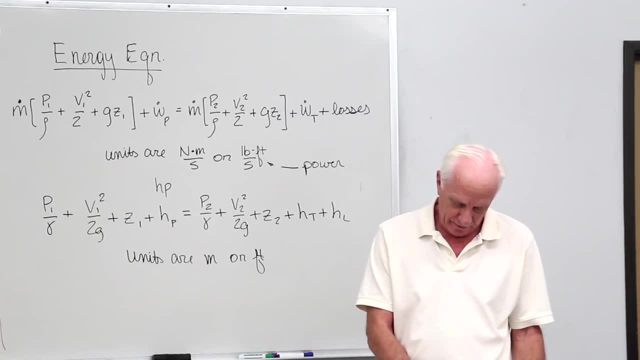 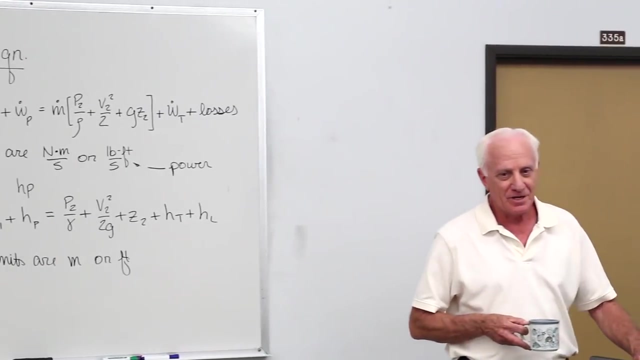 Chapter 3. You work, 12 for homework, 13 and 12.. 25 problems now you work. I worked at least four in class, So you've got about right now about 30 problems to work to review for the midterm. 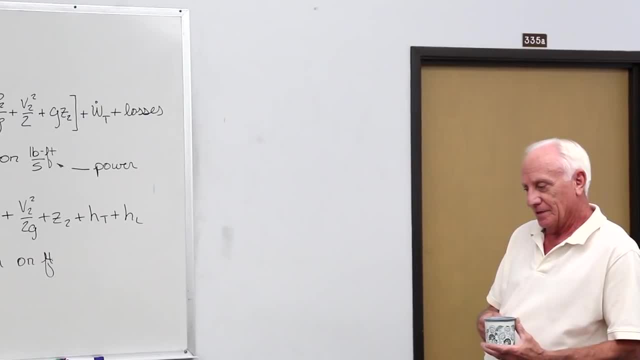 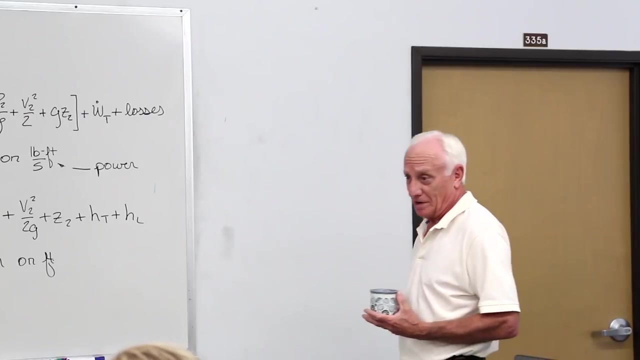 On Bernoulli's alone, What I worked in class, the ones you worked for homework and the ones worked out in textbook. That's a big library of work problems. You don't need to study much else than that. study much else than that. Okay, that's chapter three. There will be, of course, one problem. 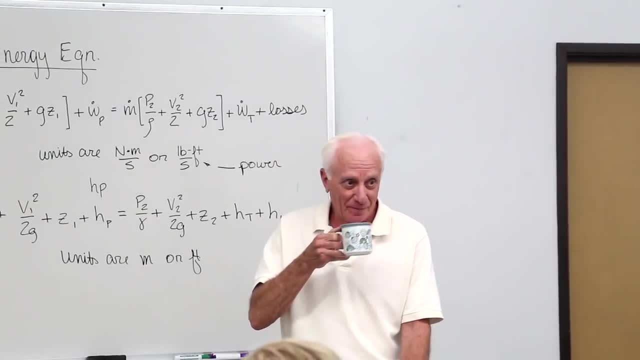 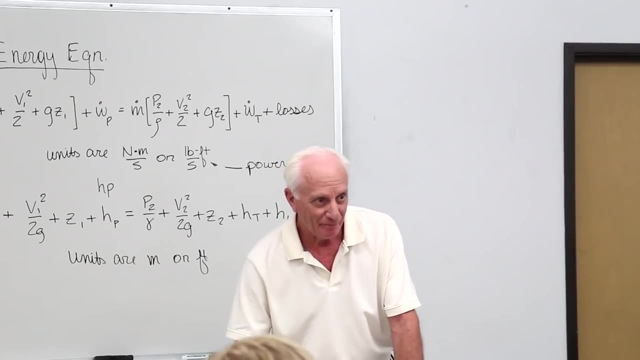 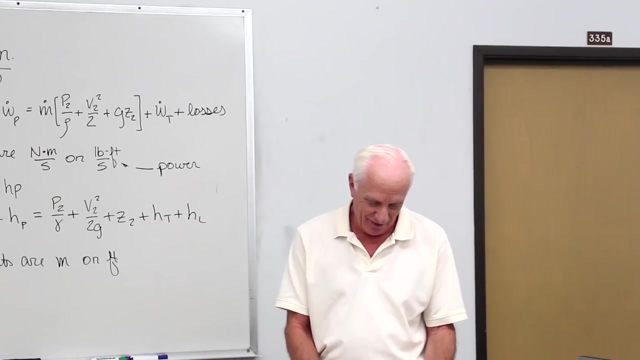 out of chapter three on a big term: Okay, Overall, the pressure is static, dynamic, total, Static dynamic, stagnation, total. Okay, Now there'll be nothing on the last sections of chapter three that I mentioned in the course syllabus. 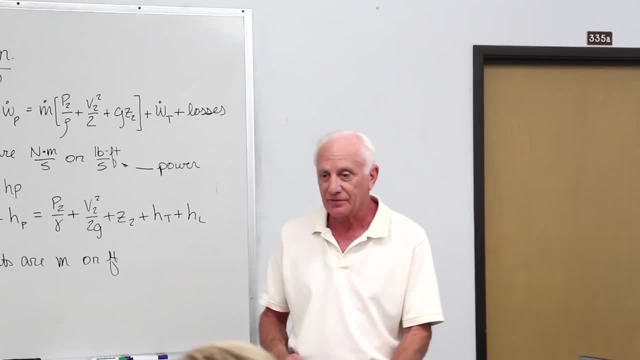 No, it's not, but nothing on section three, seven, three, eight. Nothing on sections three, seven and three, eight. Now we go to chapter four. It's a shorter chapter but it's a little more difficult, maybe, to understand. 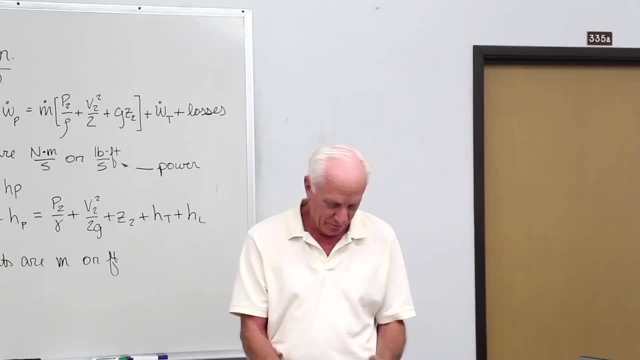 We talk about the velocity field and the accelerations. We start off talking about the difference in the Eulerian and the Lagrangian approach in fluid mechanics. The Lagrangian approach: you're following fluid particles. The Eulerian approach: you sit at one spot and say what's happening as things go past you. 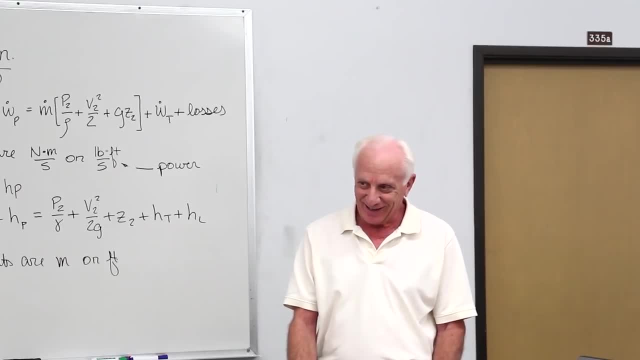 We looked at streamlines, streaked lines and path lines and you had some homework plotting streamlines and streaked lines And we did several problems in class on the board with streaked lines, as you know, and streamlines. Okay, Then we get to the acceleration field and we define the acceleration field. 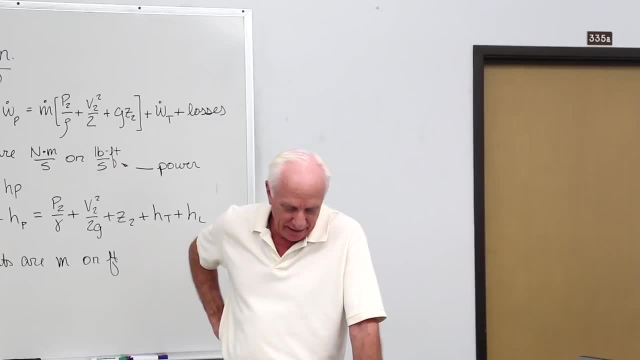 And we talked about the material derivative, the capital D DT, We talked about the convective acceleration, We talked about the local acceleration. So obviously those are important concepts. And the last part of Chapter 4 talks about the Reynolds transport theorem, which we did a bit. 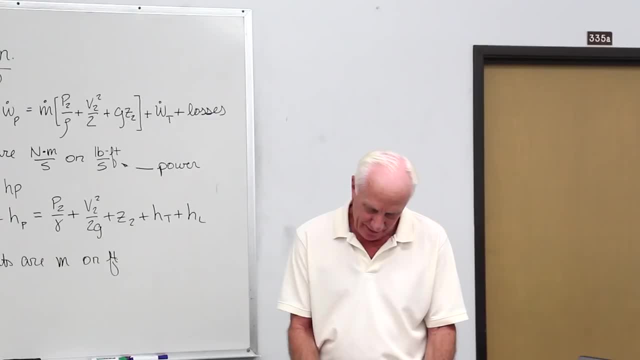 Okay, Let's see here Seven work examples. in there I probably worked Six, seven in class, That's 14.. Plus your homework, Nine, Fourteen and nine, That's 23. problems worked on Chapter 4, either for homework in the textbook or what I worked in class. 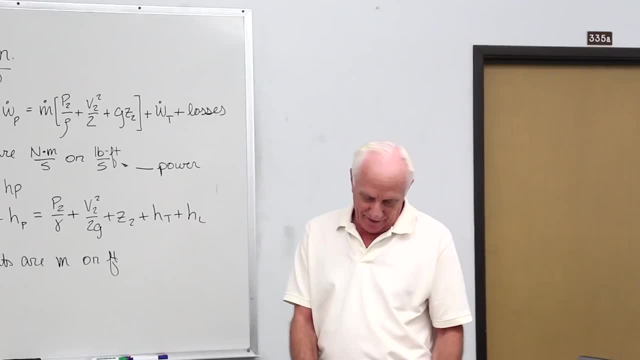 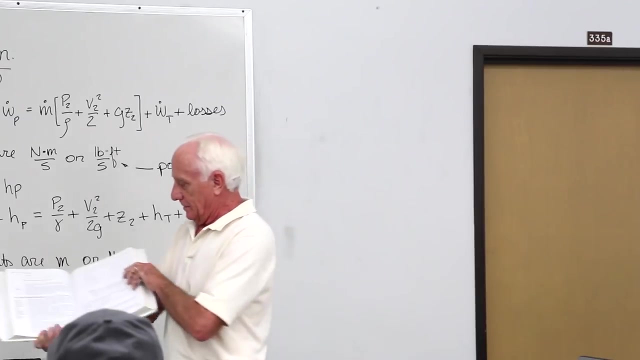 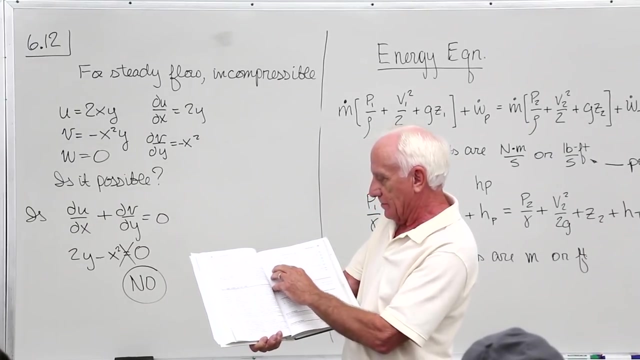 Lots of problems worked there for you to review. By the way, at the end, as I mentioned before, at the end of each chapter there is a study guide with a table which lists what the author says are the most important equations in that chapter. 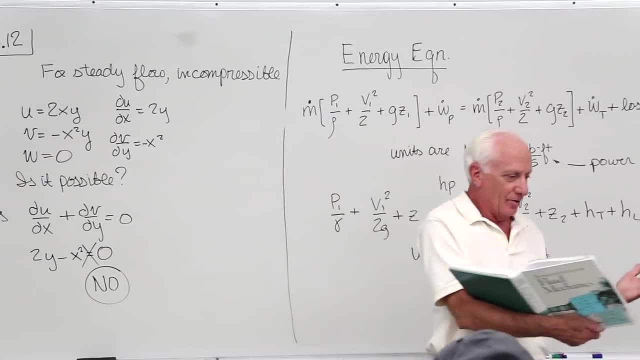 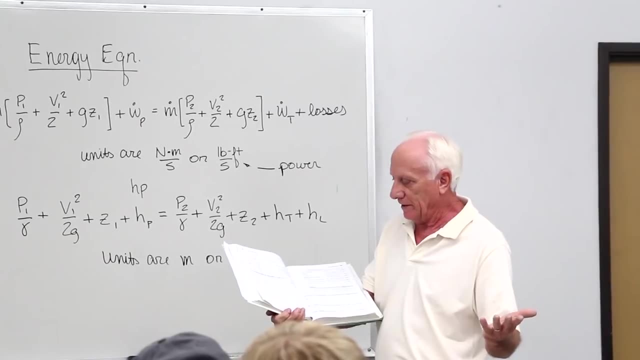 So again, you'll have that on your own equation sheets I give you, which is a table of properties of water, oil and air and so on, And you'll have them from chapters 3,, 4,, 5.. 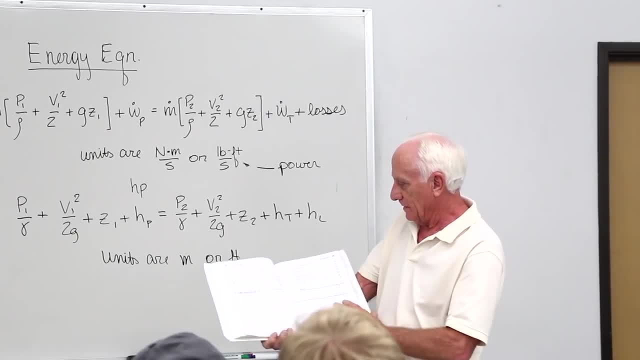 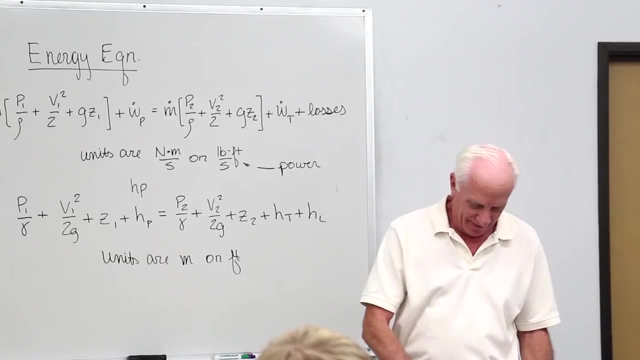 3, 4, and 5. that table at the very last chapter. chapter summary study guide. Okay, let's go on. Now we get to chapter 5.. That's the big one. In chapter 5, we apply the Rome's transport theorem to the basic laws of physics. 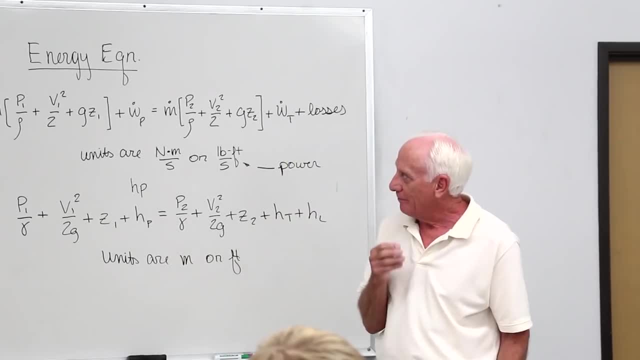 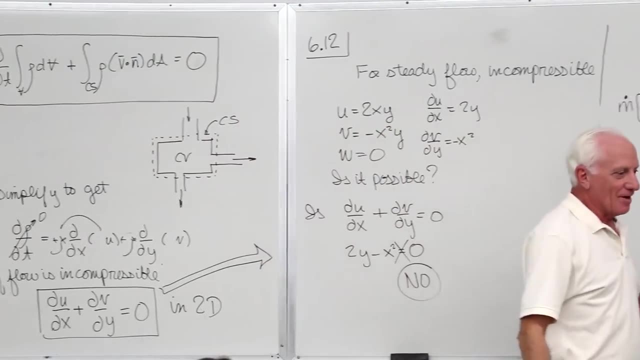 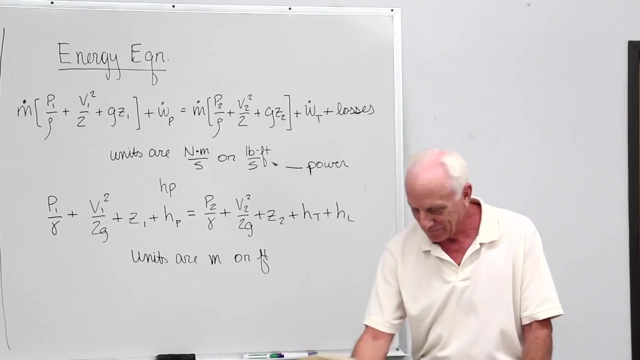 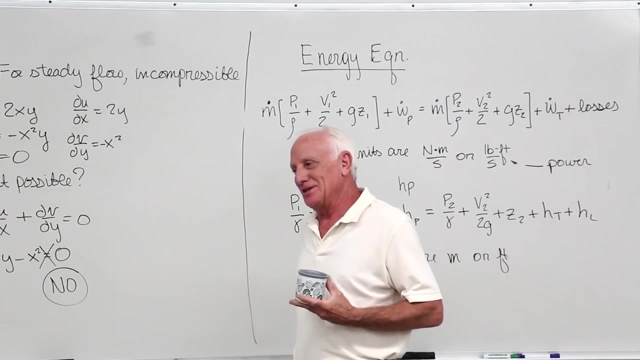 We start off with conservation of mass. We talked about how you identify a control line, how you draw dashed lines about this control line. That's the first step, Just like in statics, the first thing you do- successful people draw free body diagrams. 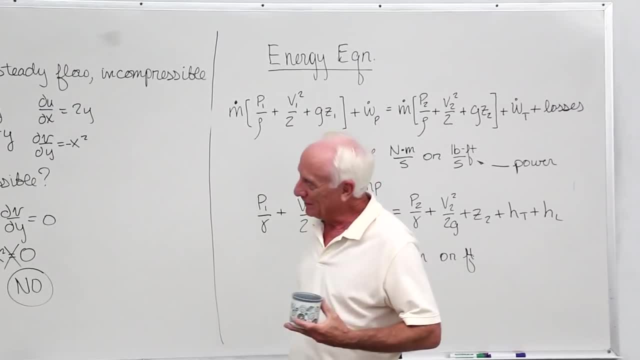 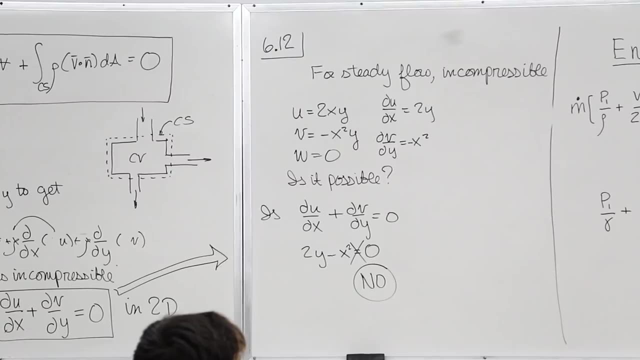 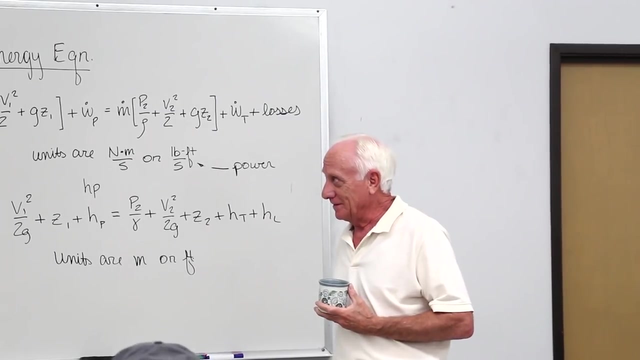 The same thing holds here. Successful people draw a control line correctly. Then you label the points, and that's not always easy. Points 1,, 2, or 3, if there's multiple places where fluid flows in, Yeah, label the points. 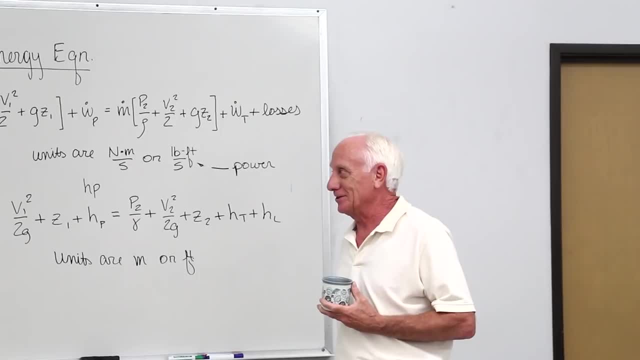 Even if you don't get too much else right, at least you get some partial credit on the exam for doing things like that. It shows me you're off in the right direction. So you know, put down some things on the table. 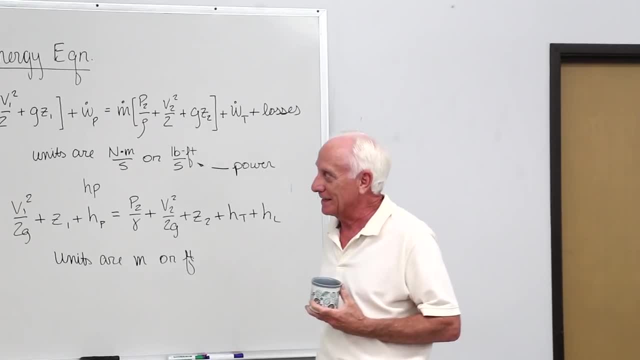 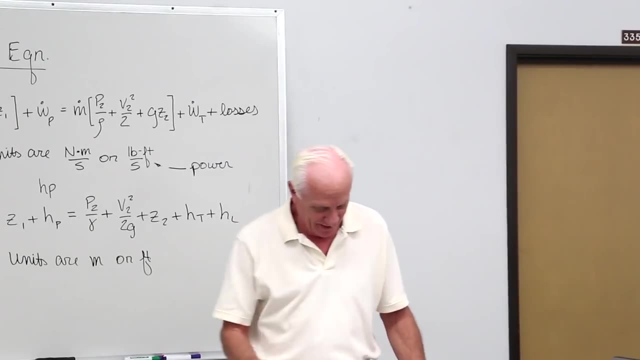 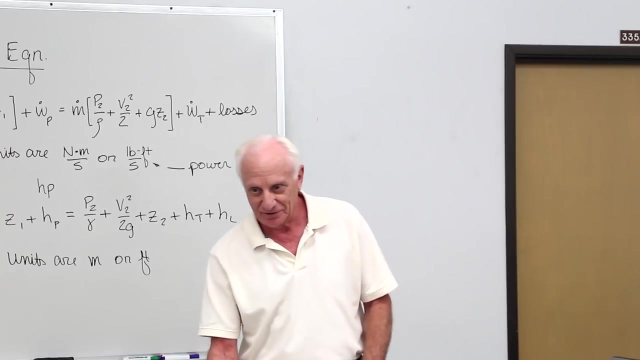 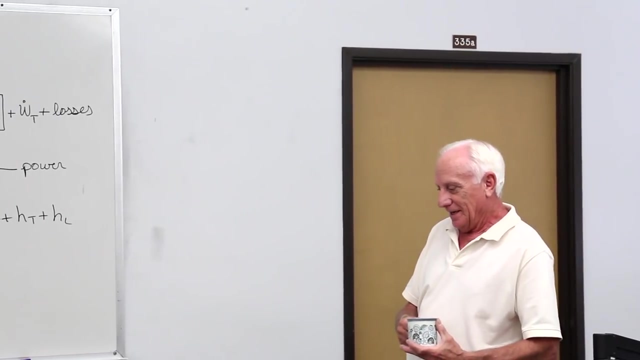 On the paper that you think can get you started, just like I did right here: Label things. Okay, conservation of mass. All right, fine, Now we move on to momentum, Probably the most difficult topic in all this material for a check for the second midterm: 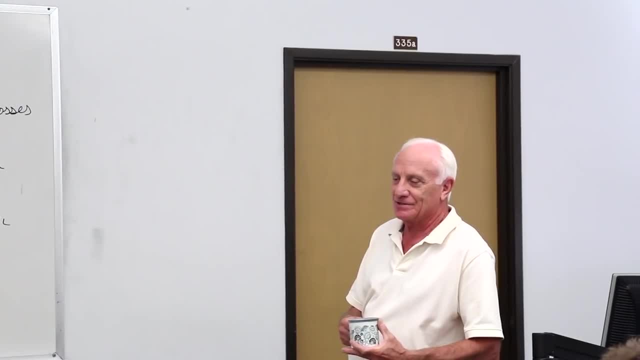 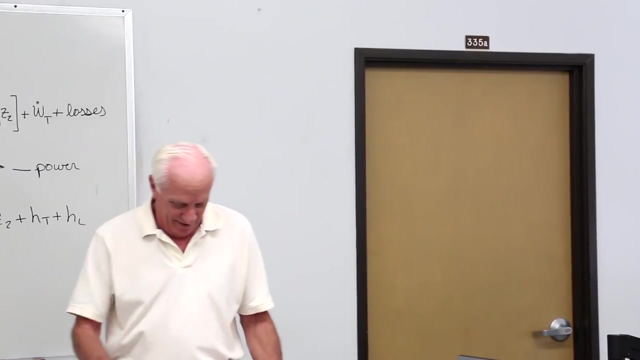 Yeah, there's dot products and vectors in there. There's signs of things that can go wrong. Things can change. You have to draw the right control line or it makes life much more difficult if you don't do it. Yeah, it can be difficult. 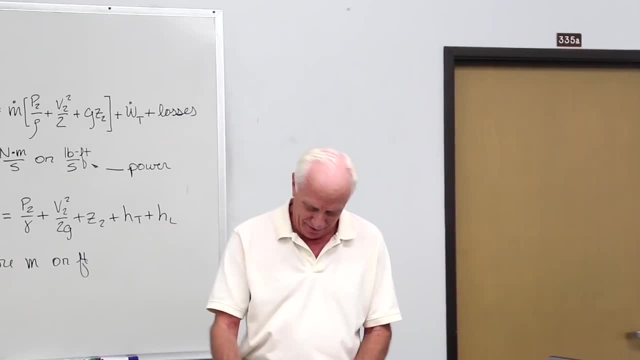 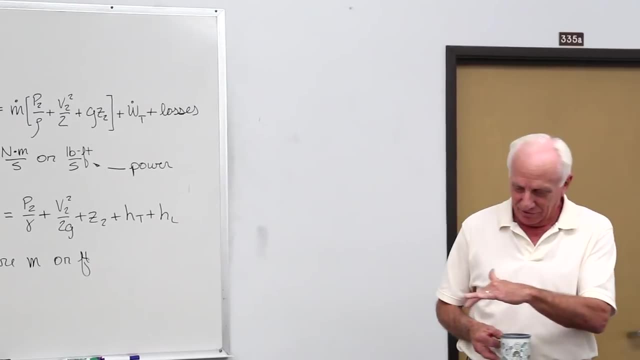 All right, you have the equation. It's pretty simplistic. There's just about one equation there. And don't forget he said that in this first level course we're going to consider steady state with momentum, So don't worry about non-steady state. 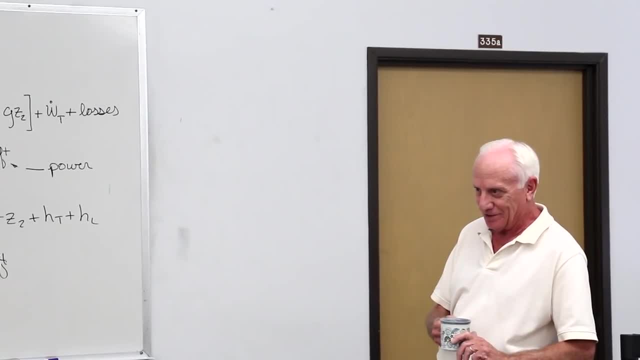 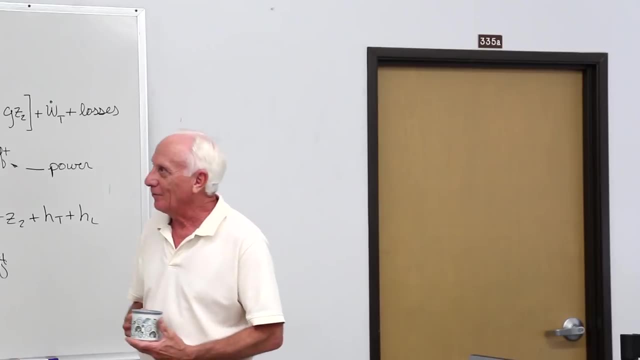 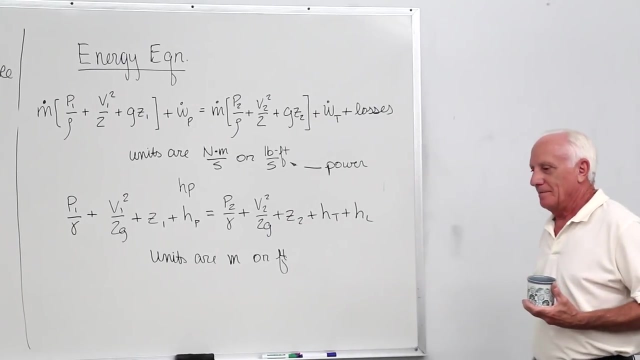 Don't worry about the time-varying term. He said we're going to consider only steady state and momentum. And then what we did today with the and last class meeting last Wednesday with the energy equation. Of course you should put down all three of those equations on your equation sheet. 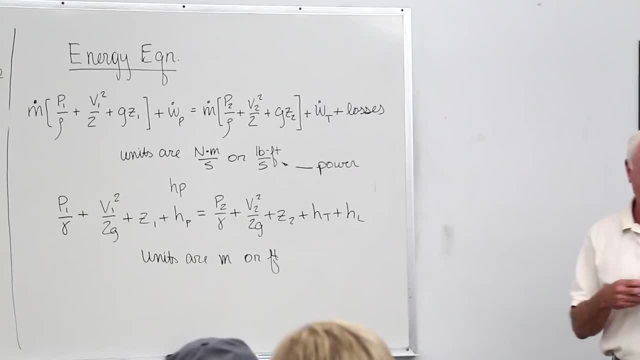 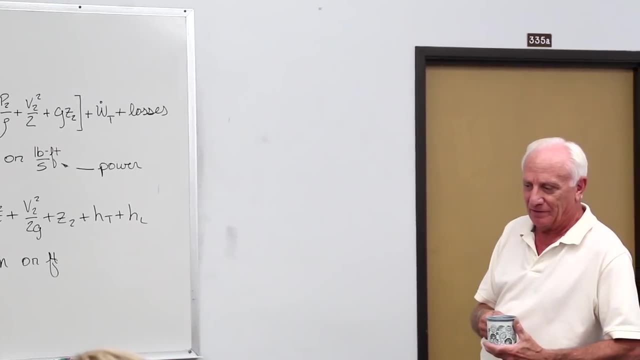 And Bernoulli's equation. Of course you should put down all three equations on your equation sheet for Bernoulli's equation, Because you don't know which one you might use. Typically, one might be easier than another one, the form it's in. 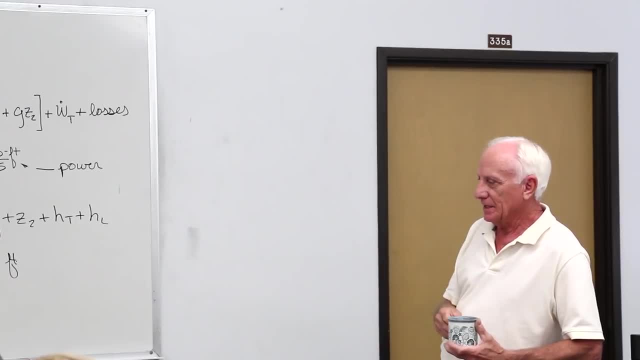 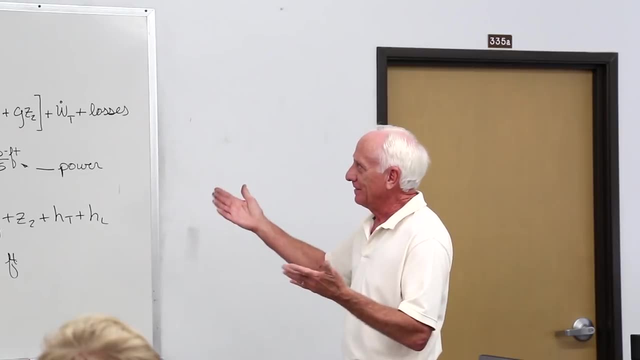 Whether it's a head form, a power form, the same thing for Bernoulli's. You know, and really can you just write down one, just write down the three equations and they apply for Bernoulli. Sure, Take these two guys out, take this guy out and guess what you got. 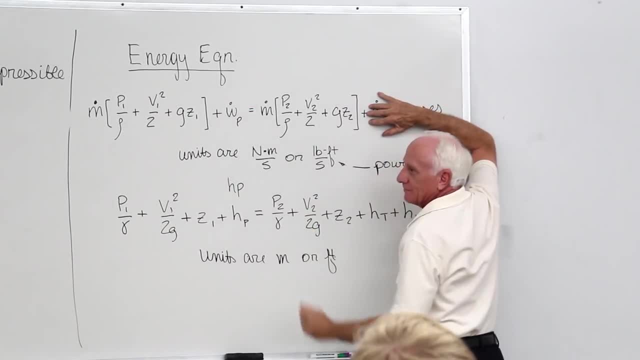 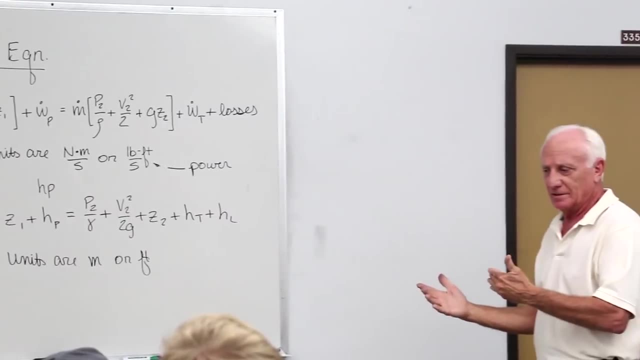 You got Bernoulli's. If there's no pump, if there's no turbine, if there's no losses, guess what? That's what you got. You got Bernoulli's. So how do you modify Bernoulli's or the extended Bernoulli? 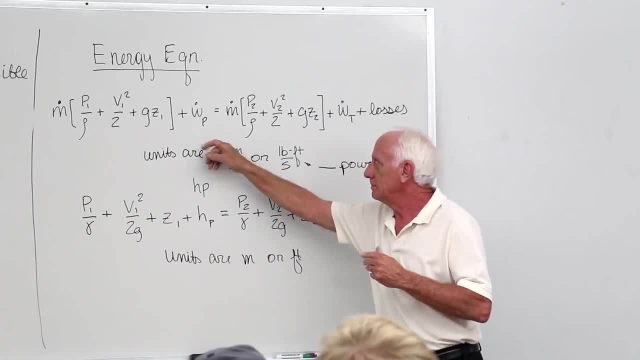 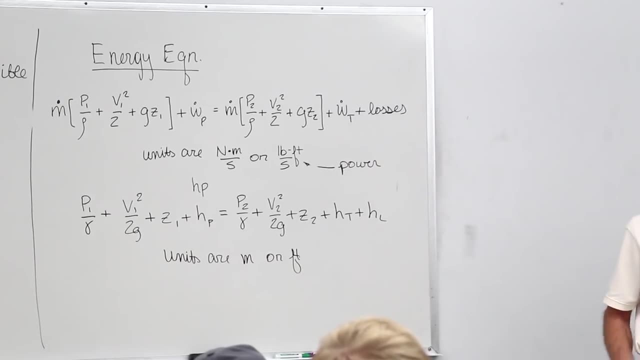 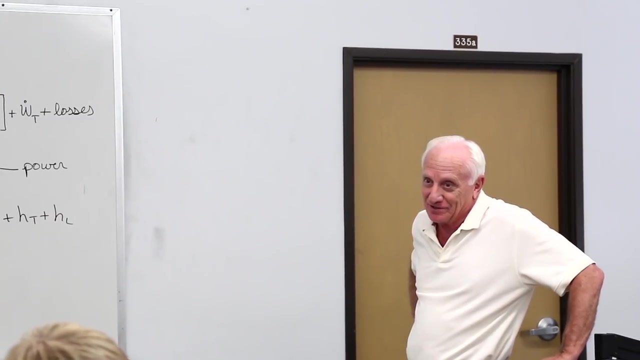 You add mechanical equipment, like a pump, like a turbine, And you know there's going to be losses in the piping network. Now you had the equation for efficiencies. Write those guys down on your equation sheet. How do you find the efficiency of a pump? 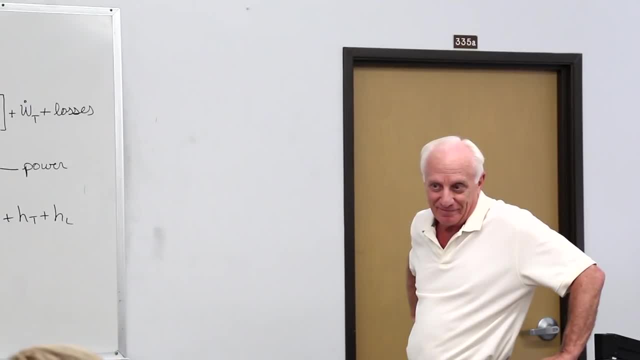 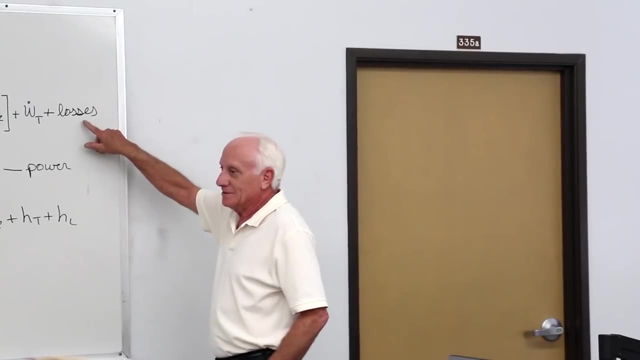 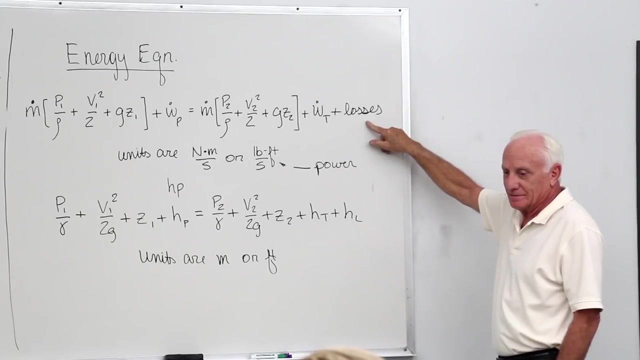 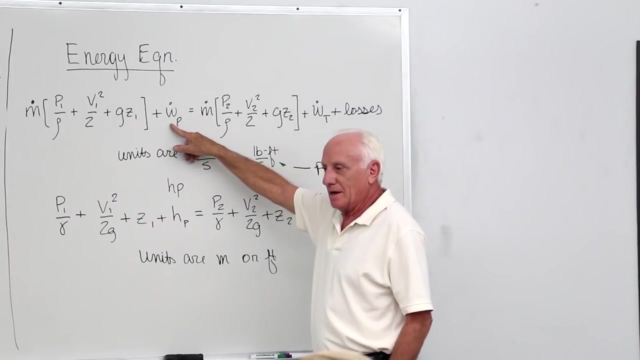 How do you find the efficiency of a turbine? Are these losses part of the inefficiencies of turbines and pumps? No, These are the piping losses. This is the amount of power that goes into the- let's say it's water, the amount of power that goes into the water from the pump blades. 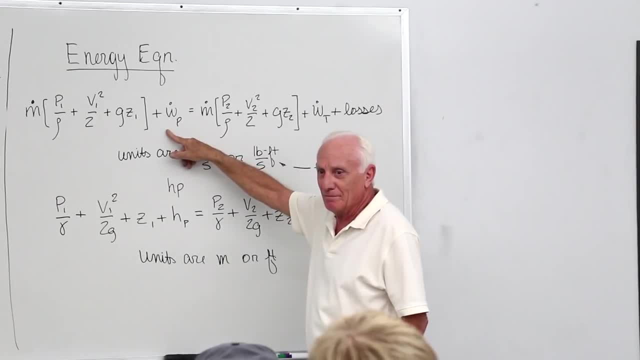 How much power does it take to drive the pump with a motor? That's where the efficiency comes in. If you multiply the efficiency of the pump by the motor power, that gives you this guy. This guy is the power that goes into the water from the blades of the pump. 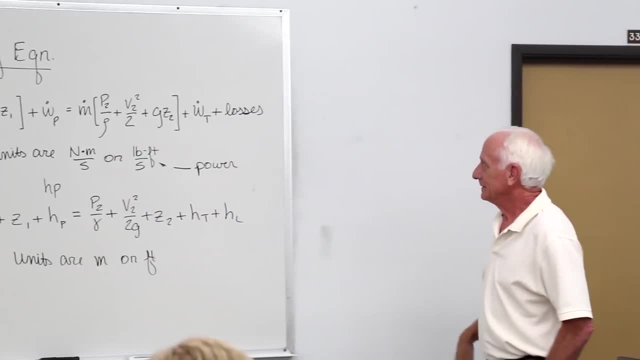 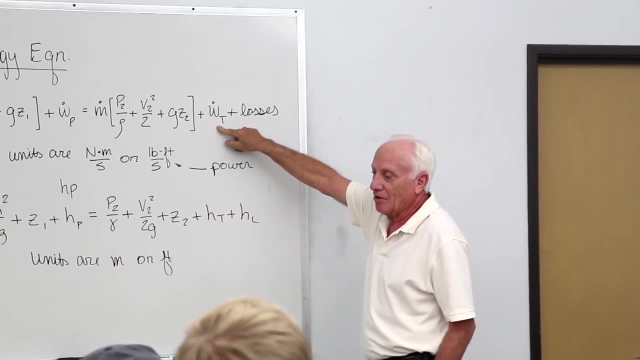 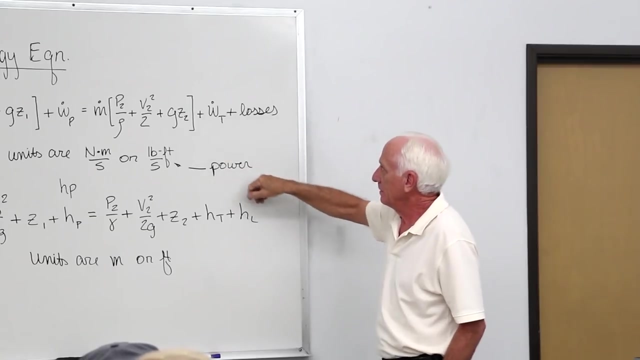 Same thing here: Turbine. What does a turbine do? The blades take energy out of the water. Then what does the power do? Oh, it typically runs a generator, for instance, Or it does some useful work. So these losses are only piping losses. 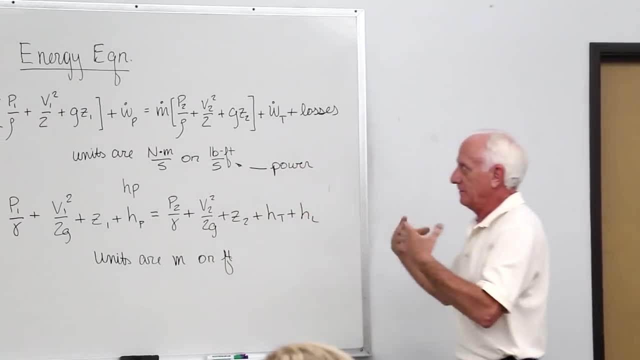 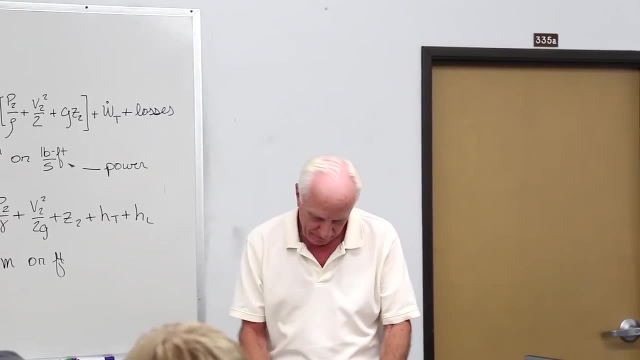 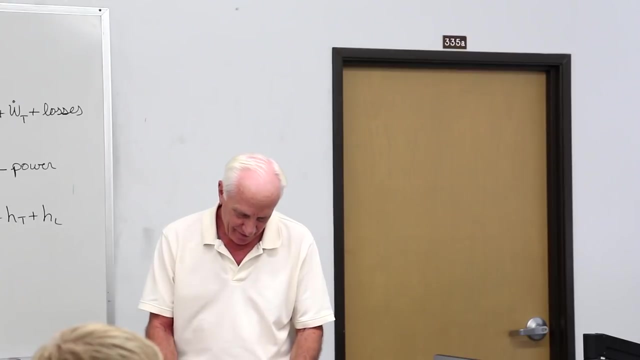 The other losses these two guys come in, wrapped up in their definition of what W dot P and W dot T is Okay, Energy equation. Yeah, Oh boy, Okay, 16 and 20, 28.. 38, 48 minus 4.. 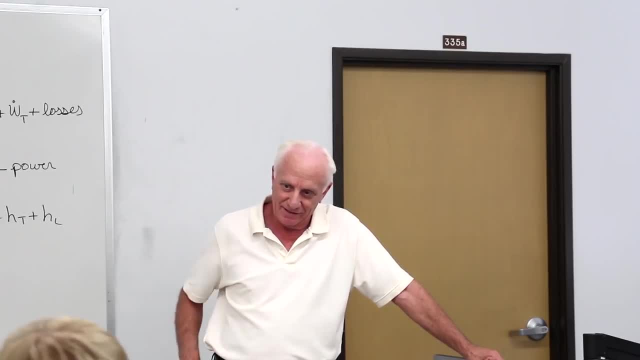 44 problems you have there. I've worked at least a dozen in class 44 and 12.. You've got between 55 and 60 problems now in your library of things to study for the second midterm on chapter 5 stuff. 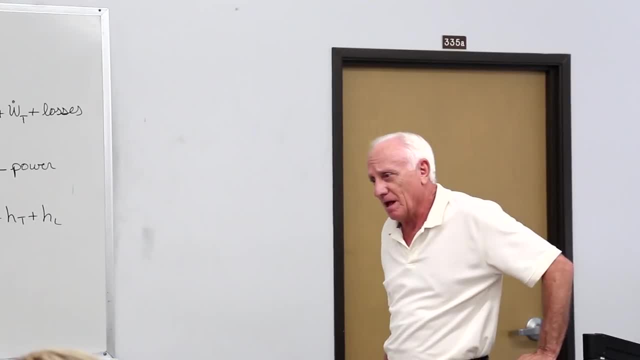 Wow, 55 problems Between the problems I've worked in class, the ones you've worked for homework and the ones that are worked out in the textbook. That's pretty major. Should you study anything else, I don't see why you should. 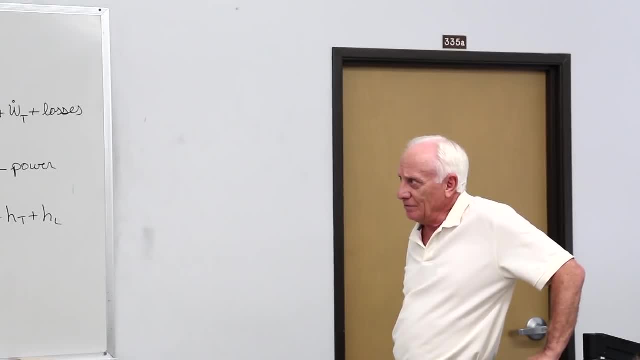 Because that's where I get my ideas. How do I get my ideas? I say: you know what? I assigned that problem for homework. I'm going to tweak it, I'm going to turn it around, I'm going to give you something different and ask you for something different. 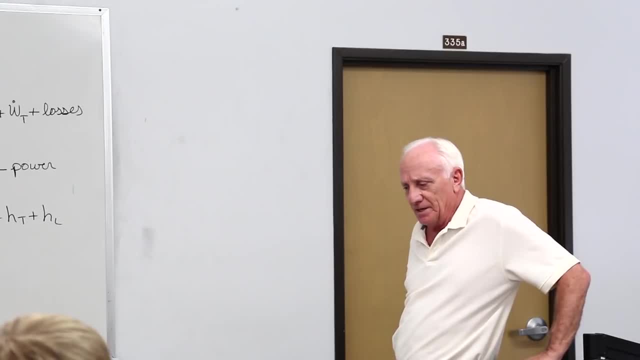 Or I might change the geometry In momentum. Maybe something came in and turned by 45 degrees. I'll have it come in and go back out. this way, 45 degrees, Not that way 45 degrees, This way, 45 degrees. Can you work that problem? 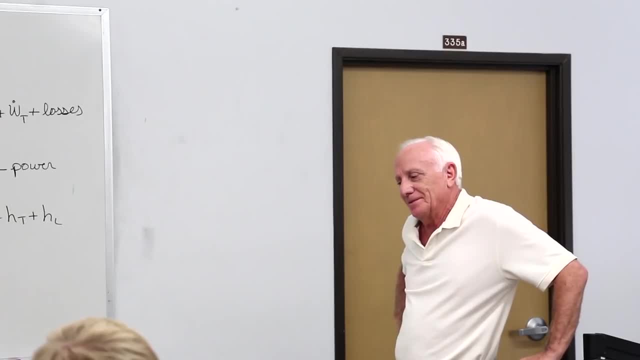 Because the signs are critical. That's where I get my ideas. Why do I assign those guys for homework? Because I think they're important. That's why I assign them. That's how you study for the midterm. That's where I get their ideas.